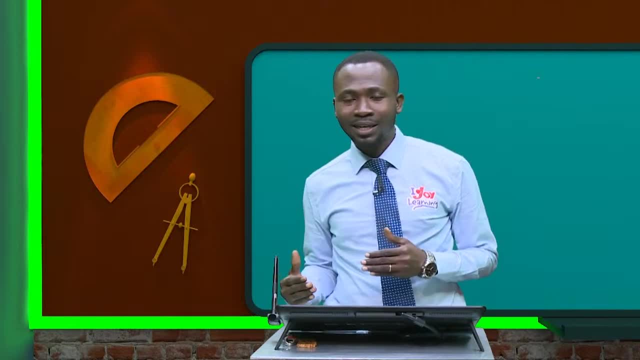 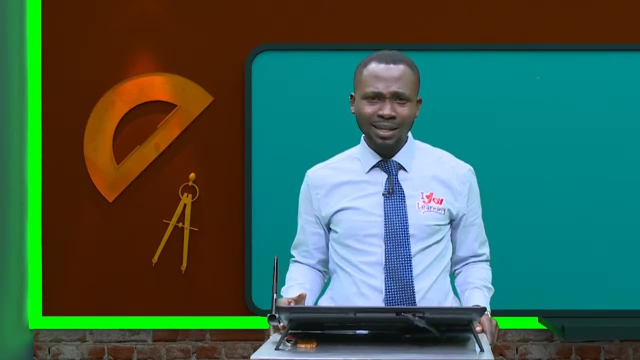 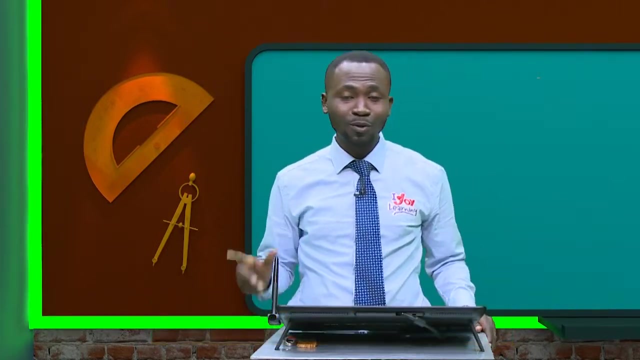 Do you know that teachers who have observed they've taken analysis of the kind of questions that YAEC asks students in exams and with their experience they advise that students should answer some particular kind of questions. They should prepare and answer those kind of questions. Are you aware of that? 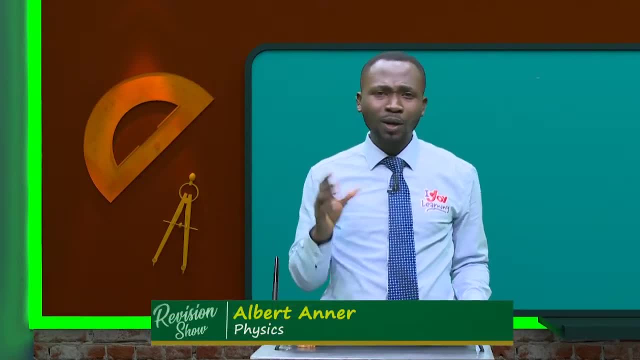 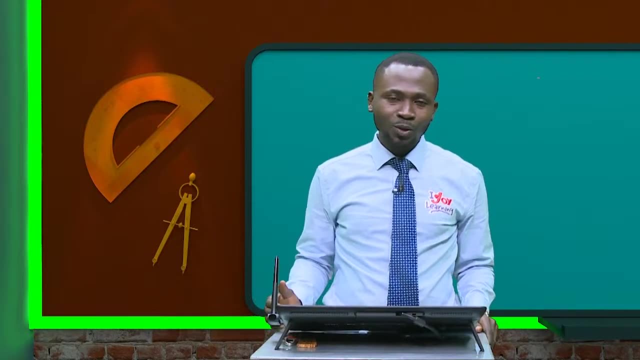 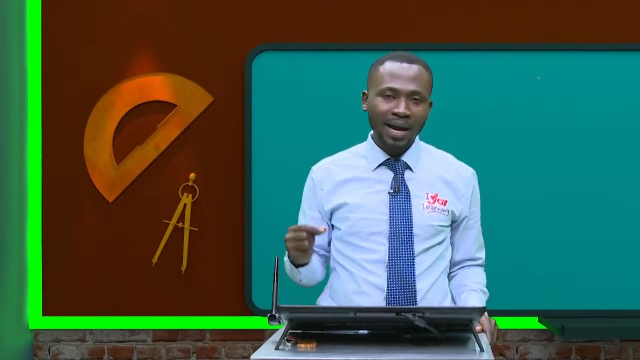 Then one of those questions or one of those areas is atomic and nuclear physics. If you should prepare very well to go and answer questions on atomic and nuclear physics, the chances that you're going to score more than 80% of the marks for question number 12, atomic and nuclear physics- is very high. 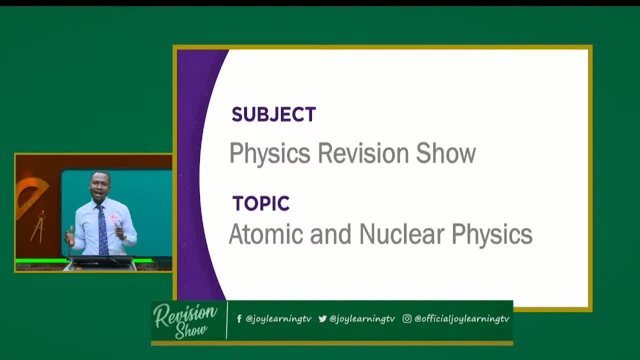 So tonight I want to take you through some portions, some aspects of atomic and nuclear physics And if you should take it so seriously, I am very sure it will help you to come out with a very good grade as far as the WASI physics exam is concerned. 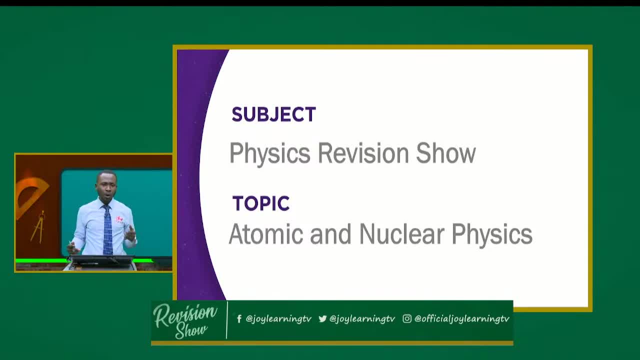 So stay glued with me. Let us do a recap of the things you have learned right from SHS 1.. And then let's prepare for the forthcoming exams. You can call other friends to also tune in and enjoy the lesson. Now, as the lesson gets to its tail end, I'm going to give you the chance to call in. 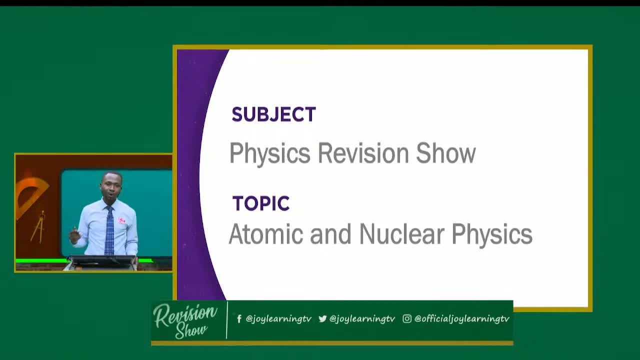 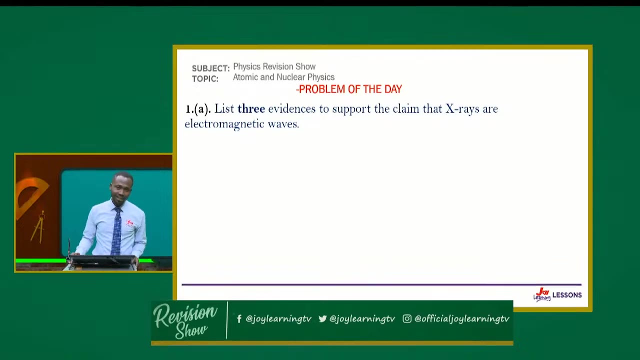 And answer what we call the problem of the day. So before we start tonight's lesson, let us take time and go through the problem of the day. The first one says: list three evidences to support the claim that X-rays are electromagnetic waves. 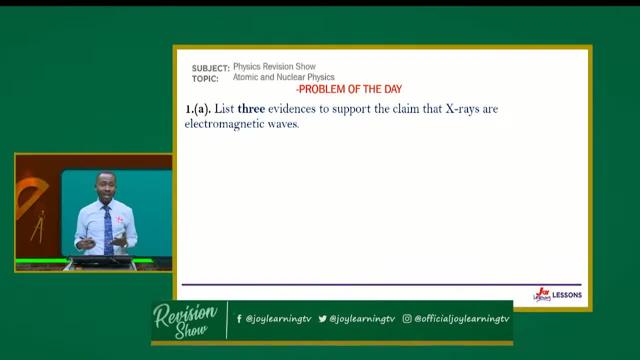 So, as the lesson goes on, we will look at what we call X-rays, And then you should be able to tell me why X-rays are, or they form part of electromagnetic waves. Next one says light of wavelength 4.5 times 10 to the power minus 7 meters is incident on a metal, resulting in the emission of photoelectrons. 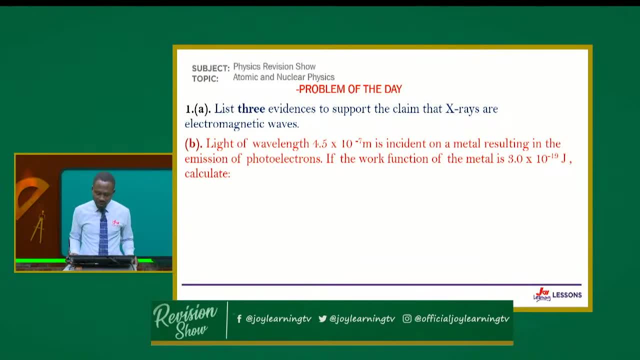 If the work function of the metal is 3.0 times 10 to the power minus 19 joules, then we calculate: I, the frequency of the incident light, Then II the energy of the incident light, Then III the energy of the photoelectrons. 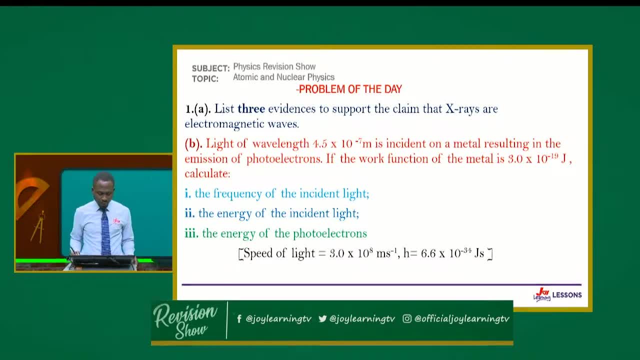 That is our problem of the day. We'll be giving additional information. that speed of light- here it should be speed of light in air 3.0 times 10 to the power, 8 joules per second. Then H, which is Planck's constant, is 6.6 times 10 to the power, minus 34 joules per second. 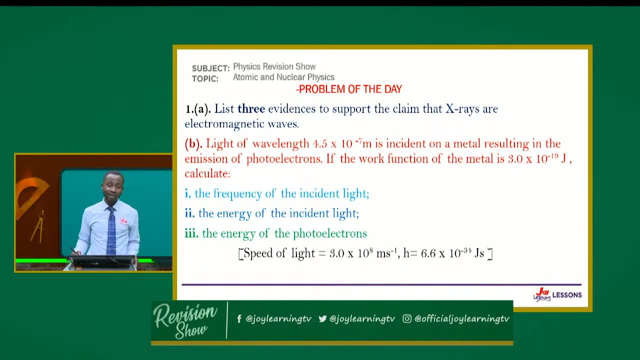 That is the problem for tonight's revision show. Try to take a shot of it and try your hands on it as we go through the lesson. I'm very sure that when I open the phone lines you will call to give me answers to these questions. 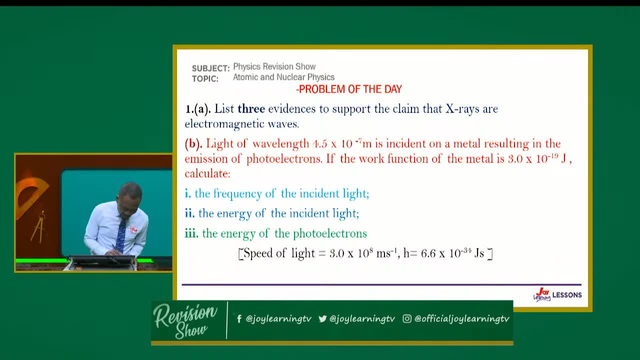 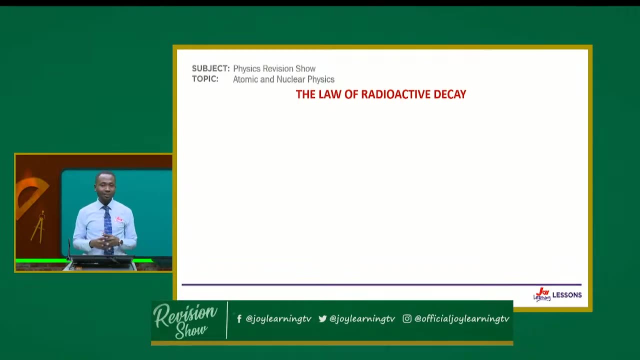 All right, this is also a past question, so it's a likely examination question. What is June 2018, questions 12B and D: Good, so let's start by rolling. Tonight, I'm going to look at the law of radioactive VK. 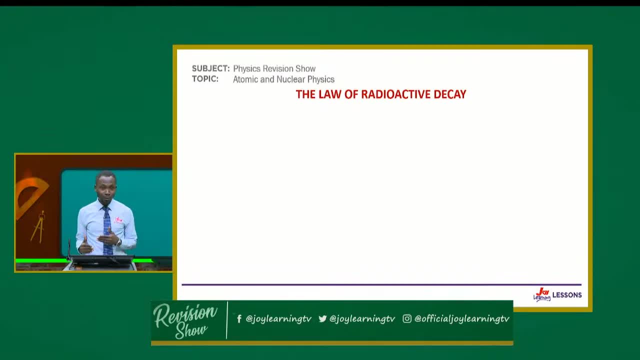 an aspect that most of the times may confuse or may trouble students. So I'm going to take my time and take you through it step by step. Make sure that you follow all that I'm going to do tonight And I'm very sure that after the revision show, when you lay your hands on any questions on radioactive VK. 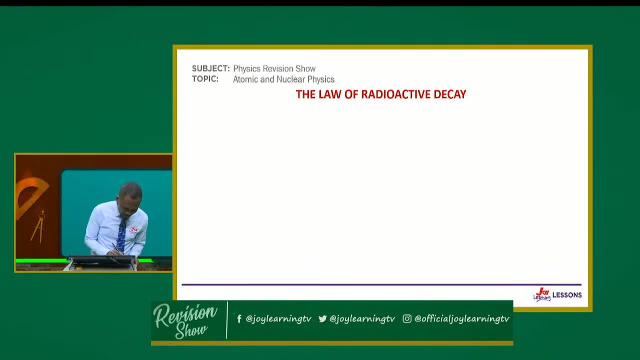 you will be able to answer. All right, what does the law say? The law of radioactive VK says that the rate of decay to rate of decay of a radioactive nuclei is directly proportional to the amount of radioactive nuclei present at that time. The rate of decay of a radioactive nuclei 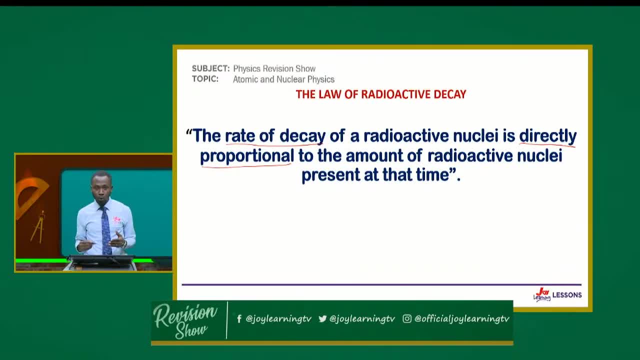 how fast or how slow a radioactive nuclei will break down or split open or decay depends directly on the amount of the radioactive nuclei that is present. So if you have a radioactive nuclei in a huge or large amount present at a particular time, it will decay at a faster rate as compared to one that is in smaller quantity at a particular time. 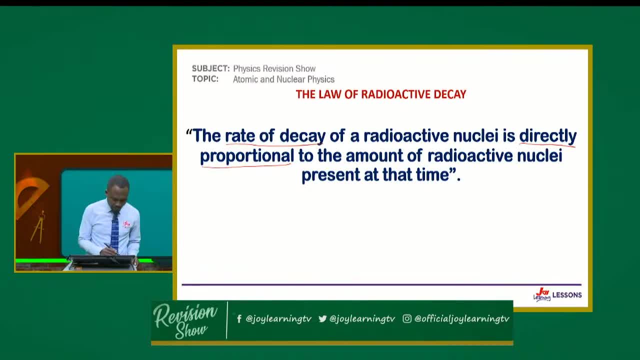 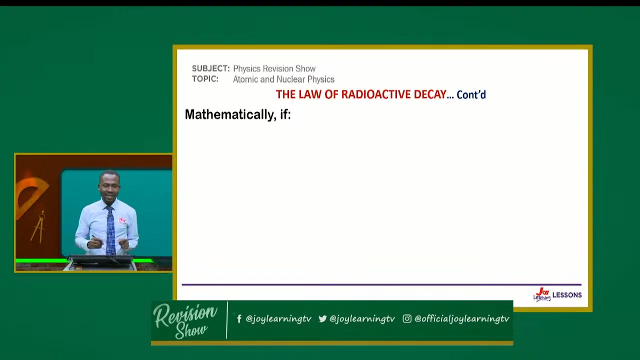 That is the law of radioactive VK. So you have to keep this law because that will help you to write mathematical expressions of the law. So mathematically we want to put this law into an expression. It says that the rate of decay of a radioactive nuclei okay. 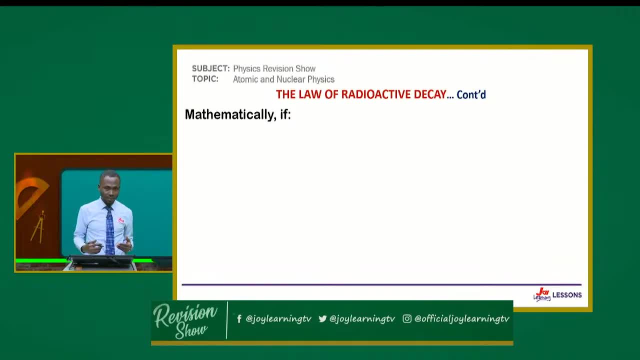 so the rate is how much of the nuclei decays per time, per change in time is directly proportional to the amount of radioactive nuclei present at that time. So we want to use n to represent the number of nuclei initially present in a radioactive sample. 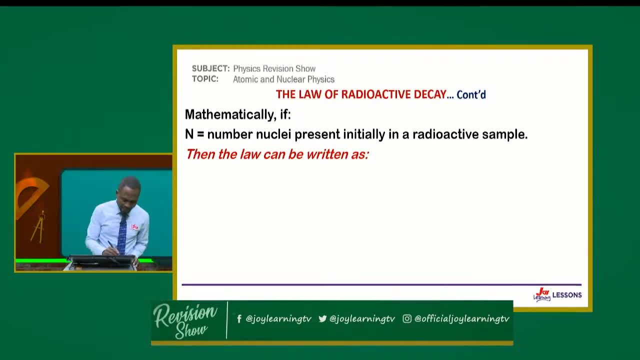 Right. So the law can be written as dn on dt. This is the rate of decay, dn- change in the amount of radioactive nuclei present. dt with change in time is directly proportional to the amount present at that time. So the whole law can be summed in this. 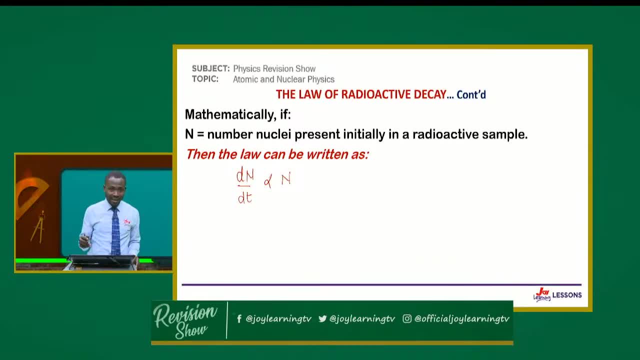 The n on dt is directly proportional to n Right. So the n on dt is our rate of decay of the radioactive nuclei, and is directly proportional to n, the amount that is present at that time. So the n equals the amount of nuclei that decays. 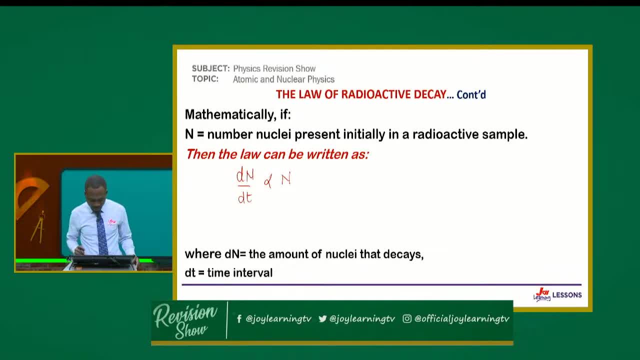 and then dt is the time interval. Let's move on. So the n on dt together gives us the rate of decay. So the expression that I just wrote, which is the n on dt, is directly proportional to n. This expression can be written as: 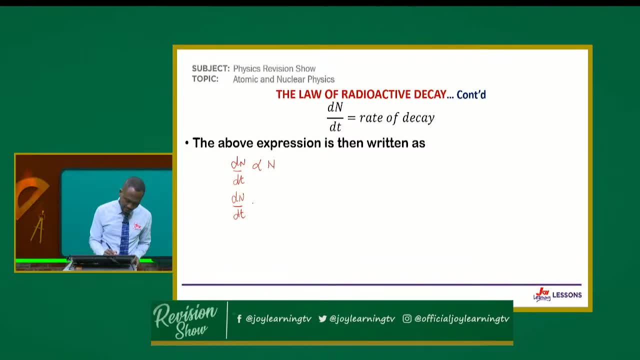 dn on dt is equal to minus lambda n. So here I have changed the sign of personality, this sign, and I've brought in an equal to sign and I've introduced a constant Here. the constant is lambda, called the decay constant. 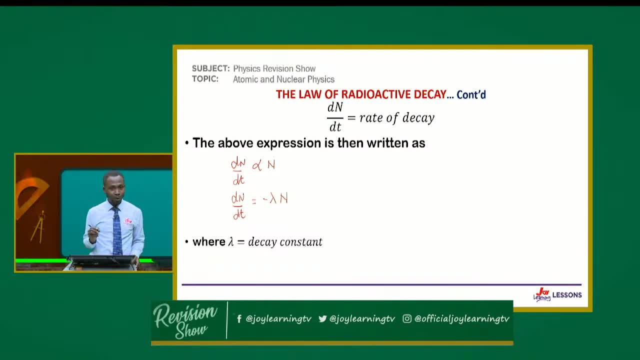 So lambda is equal to decay constant. I can't work with a sign of personality, so I change into an equal to sign And to take care of whatever errors might come in the equation, I introduce a constant of personality which is the decay constant, lambda. 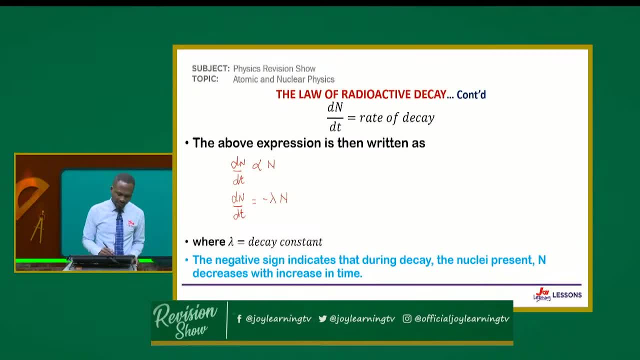 So why do you have negative sign there? The negative sign indicates that as decay goes on, during decay of radioactive nuclei, the nuclei present, the amount present decreases with time. So if you have a radioactive nuclei and it is decaying, 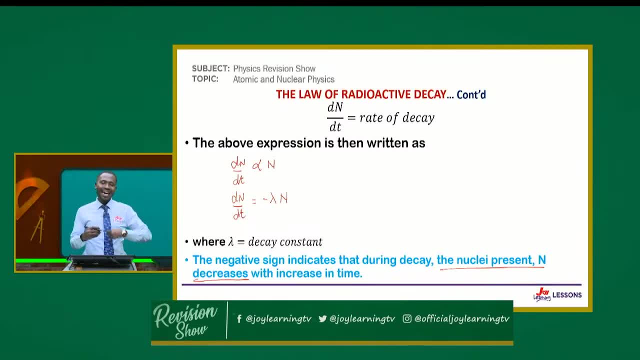 as time progresses. as time increases, the amount that is present, the amount that is left will be reducing with time. So the negative sign only indicates that the amount of radioactive nuclei present as decay goes on decreases with time. So our decay equation gives us: 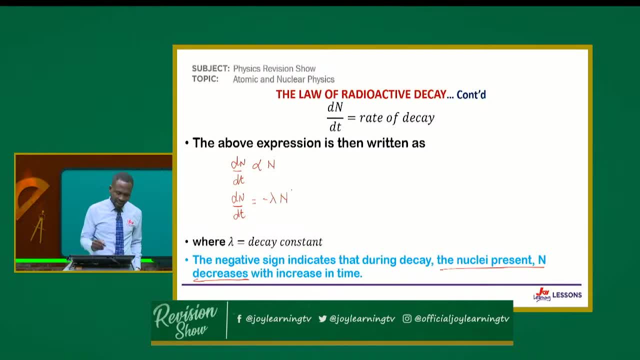 the n on the t is equal to minus lambda n. You don't have to forget this expression. It's very important. Alright, let's move on to higher things Now. decay constant. We just wrote an expression. The n on the t is equal to minus lambda n. 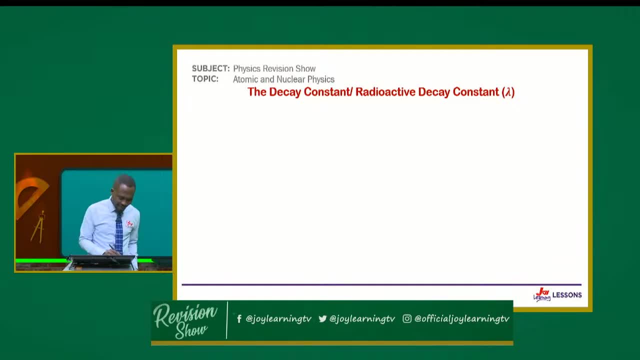 And we are saying that lambda is the decay constant. So if lambda is a decay constant, that's it. what will be our definition of it? Well, we can try and make lambda the subject from the expression. So from the n on, the t is equal to minus lambda n. 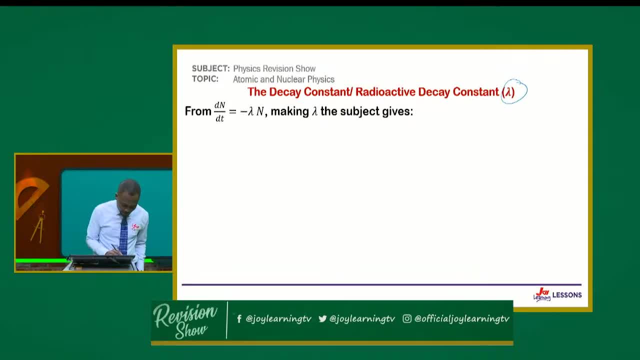 let us make lambda the subject So I can say lambda will give me minus. into brackets the n on the t right all over n. How I try to divide what I have on the left-hand side by n so that lambda will stand alone. 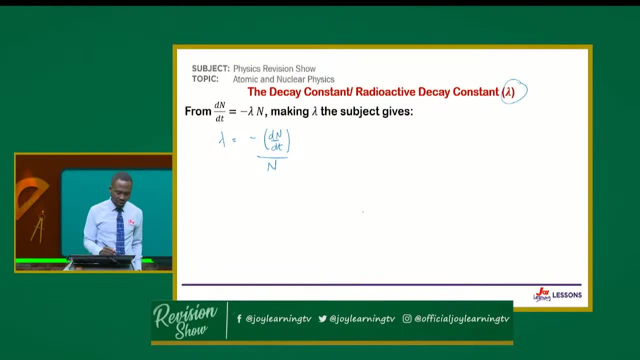 But there's a negative sign there, so the negative also goes to the other end. So if I have lambda, which is my decay constant being equal to minus, into brackets the n on the t, all over n, I'll just forget about the negative in my definition. 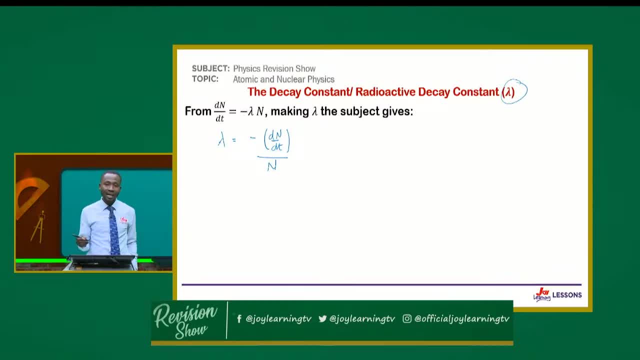 because it is only telling me that the amount of nuclei that is left as the decay continues with time decreases with time. But the n on the t is the rate of decay and n is the amount of radioactive nuclei present. So what will be our definition for the decay constant? 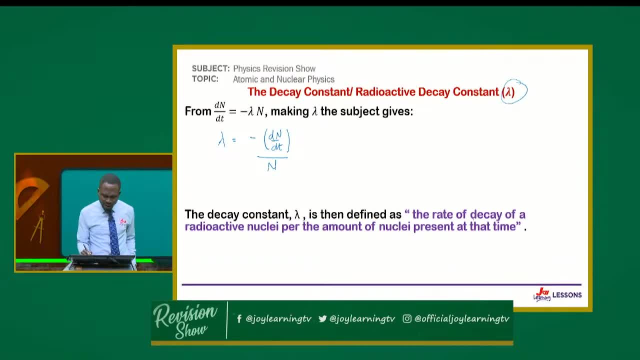 We will say that the decay constant is the rate of decay. The rate of decay refers to what? It refers to this, the n on the t. So it's the rate of decay of a radioactive nuclei per the amount of nuclei present at that time. 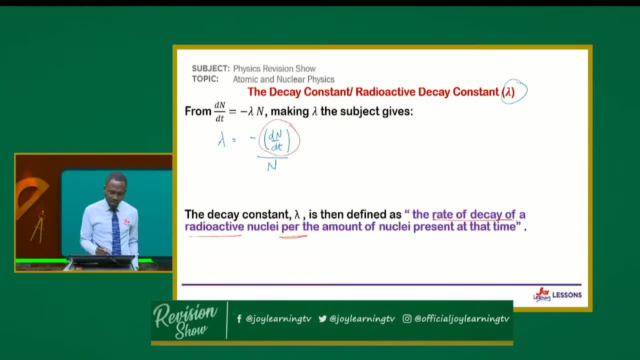 So I could say it is the ratio of the rate of decay of a radioactive nuclei to the amount of nuclei present at that time. So lambda, which is a decay constant, is the n on the t, which is the rate of decay. So it's the ratio of the rate of decay. 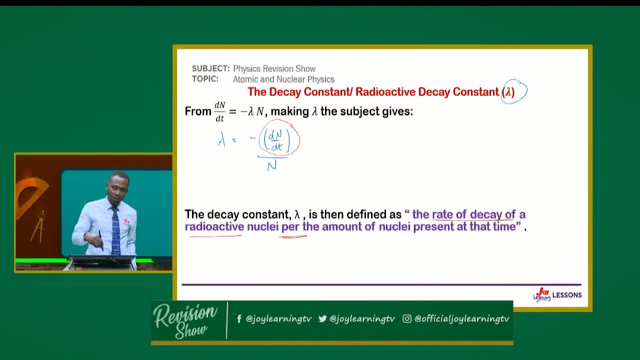 that is the n on the t, on the amount of radioactive nuclei present, which is n, And that would be our definition for the decay constant. Now the s I need is per second. Why is it per second? Per second, Look at the expression I'm giving to you. 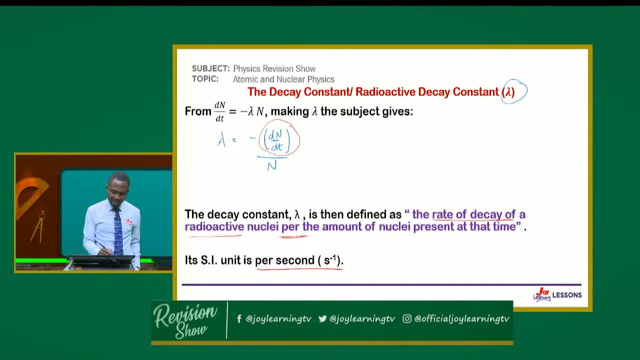 You have the n on the t. Change in n over change in t all over n. Change in n is just a change in the radioactive nuclei present. So up here I'll get one. If I look at units, change in n on change in time. 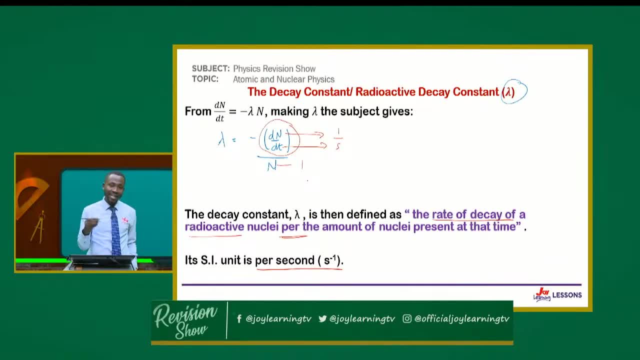 time in. second- And this is just one because I'm not going to get a unit for it- The number of atoms. the radioactive nuclei present is also a number of atoms, So no units for them. So if I have just one, on s, 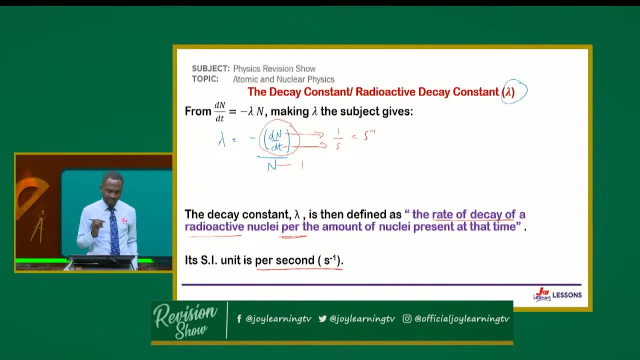 I'm going to get s to the power minus one And that gives me per second. So whenever you have the decay constant you are asked to solve for the decay constant. you make sure that you attach the unit per second to it. Very important. 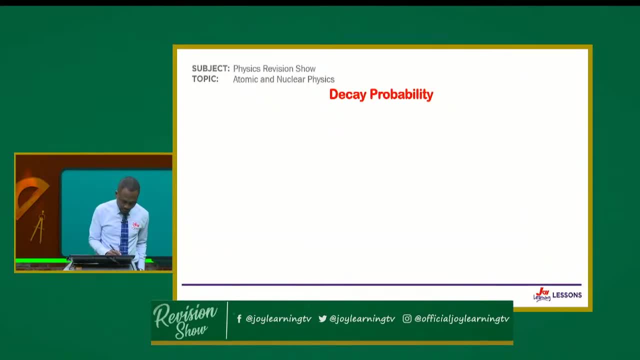 All right, Now we can look at decay probability. When you are going to look at probability, then it means that you have what we call the sample space- All that is available for you to consider. Then you are going to pick something out of all that is available to you. 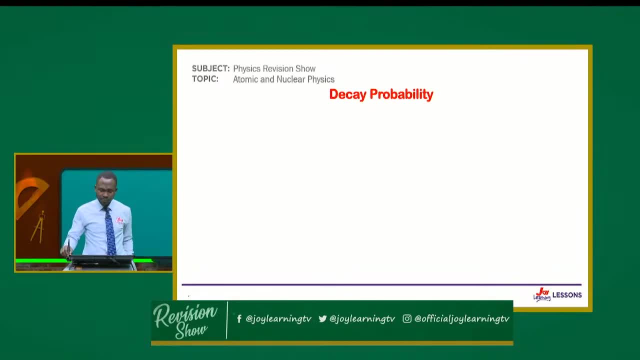 So decay probability Here. in this case I have n, which is the amount of radioactive nuclei present. Then part of it, some of it, will decay, which is dn. change in n. So change in n out of all the n should give me my decay probability. 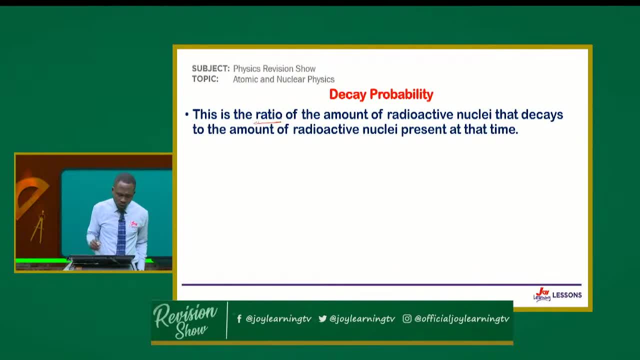 So we are saying that this is the ratio of the amount of radioactive nuclei that decays, which is dn. So all this, the amount of radioactive nuclei that decays, is the dn Right To the amount of radioactive nuclei present, which is n. 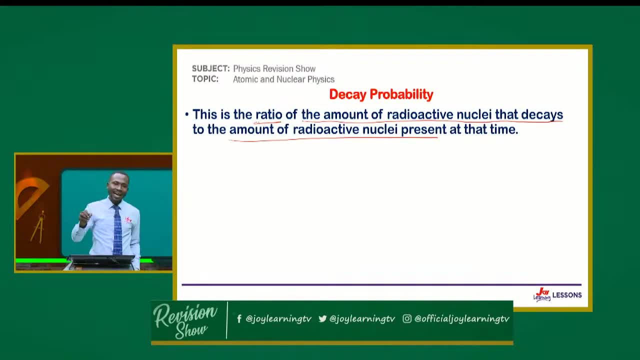 at that time. So if you keep the n on n with you, the definition will come to you naturally. So it is a ratio of the amount of radioactive nuclei that decays to the amount of radioactive nuclei present at that time. Mathematically, 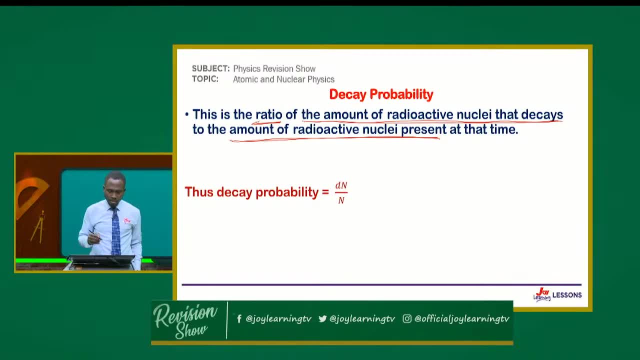 I'm going to get. decay probability is equal to dn over n, where dn is amount of radioactive nuclei that decays And then n is the amount of radioactive nuclei present at that time. The decay equation: The decay equation. So we have to also take a time and look at that. 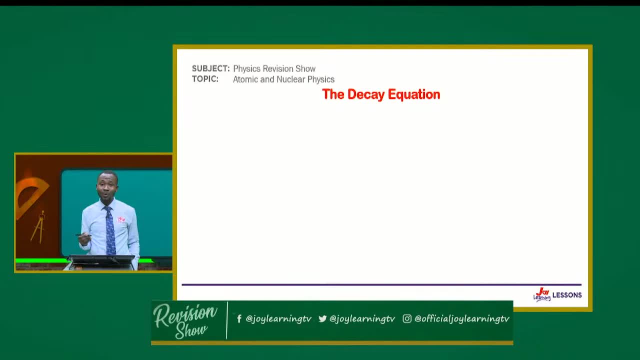 And keep the equation, Because when you are asked questions, you will be required to use the equation to solve, And if you don't know the equation, it means you will not be able to solve the question, Right. So what is the decay equation? 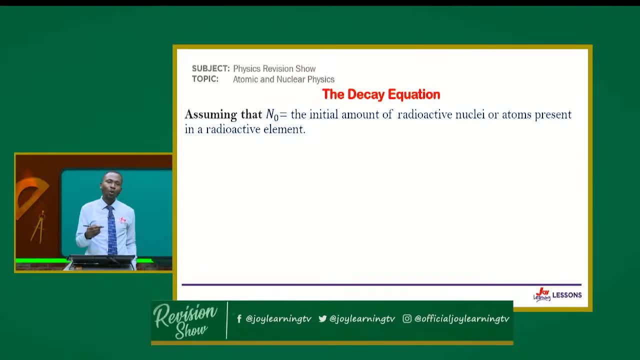 These assumptions are very important. You have to know what represents what. Other than that you won't be able to fish out the correct data And that will affect your solution. So in this case we are saying that n naught is the initial amount of radioactive nuclei or atoms present. 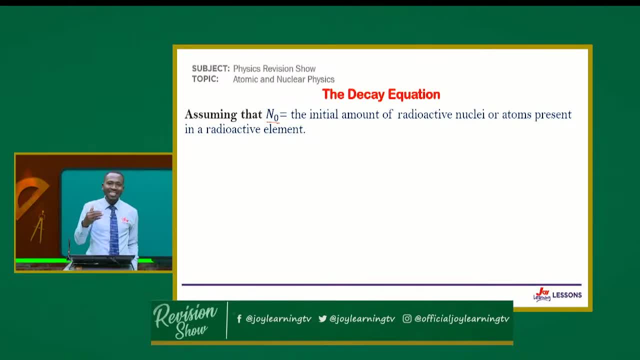 So in the reductive element before the decay there will be a radioactive nuclei present, So the initial amount of that radioactive nuclei present even before the decay starts. we are using n naught to represent that Now the decay will take place. 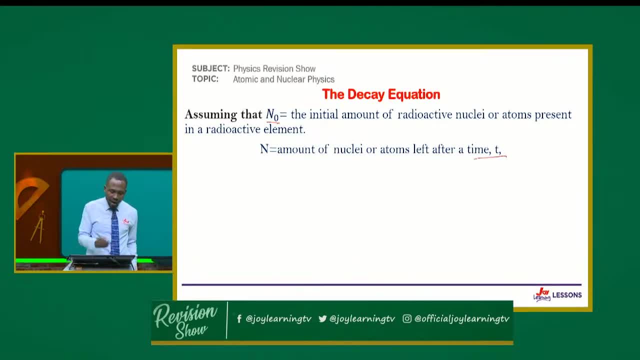 So after a time t, the amount of radioactive nuclei or atoms left after the decay is n. So n naught is what we have initially. Now, after it has decayed for some time, what is left is n. Now we are good to go. 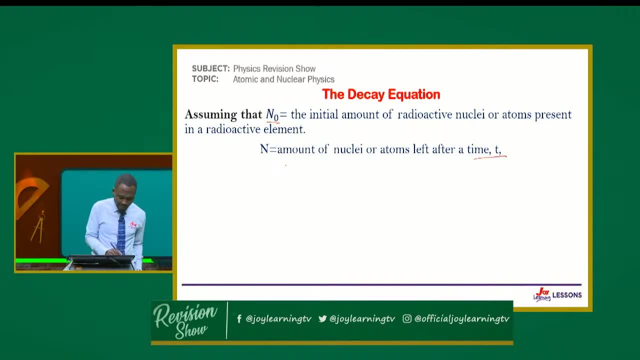 So if you have n naught to be that and n to be this, then the decay equation is given as: n is equal to n naught exponent minus lambda t. Watch that carefully, Very important. n is equal to n naught exponent minus lambda t. 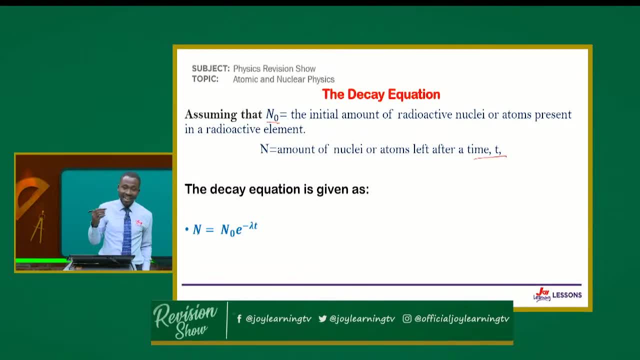 So here, n is the amount of nuclei that is left after some time of decay is equal to the initial amount of the nuclei that we have. n is equal to n naught exponent minus decay constant, which is the lambda times, t, which is time. 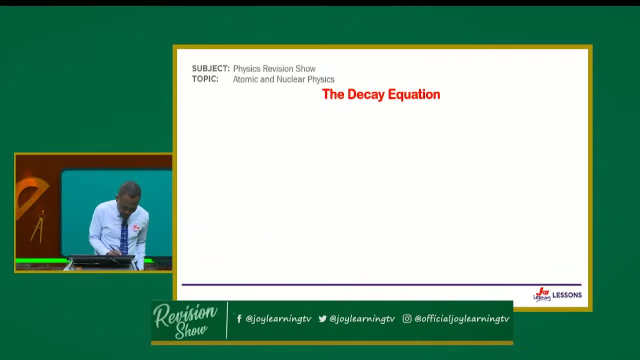 So that gives us that. Okay, So that's our decay equation. We can try and get a graph. This graph is telling us something. Our n is the amount of radioactive nuclei, this one that is left with time. But initially, 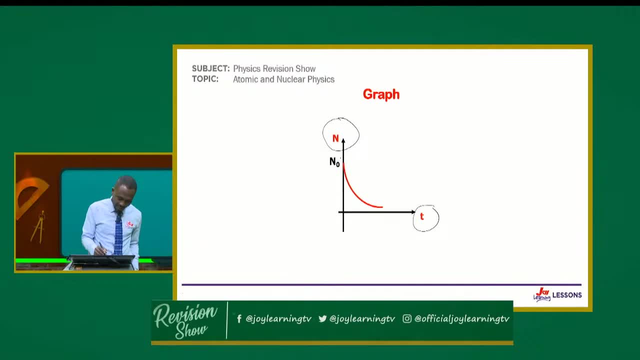 we had n naught. So n naught is the amount of nuclei you had before decay. Then the graph sucks, moves downwards. the curve moves downwards like this: It tells you that one, the decay of the radioactive nuclei is not really directly proportional to time. 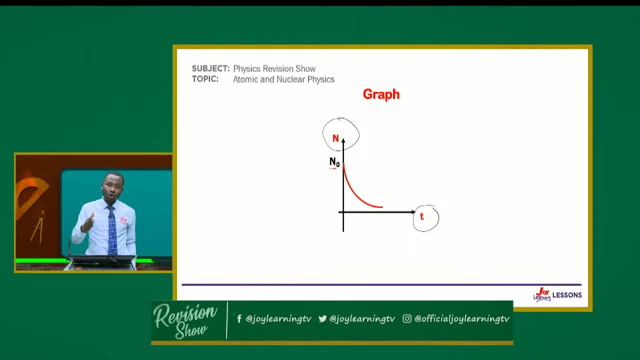 That doesn't mean that there is an equal amount of decay. You don't have an equal amount of decay of the radioactive nuclei with equal change in time interval. No, So it could be that at a point it can be a point in time. 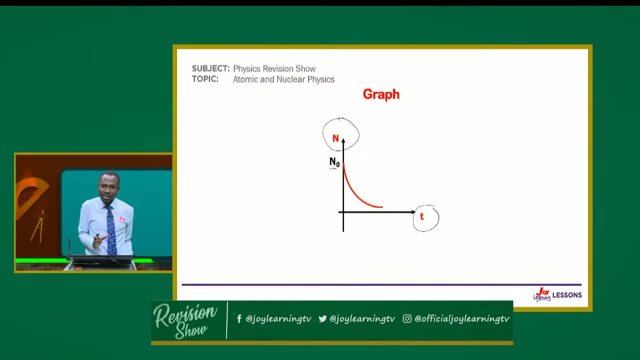 you have much more of the nuclei decaying within a short time, Then at a point in time there could be just a little amount of decay within a longer time. But we can also note that with time as time progresses, if you look at the graph carefully. 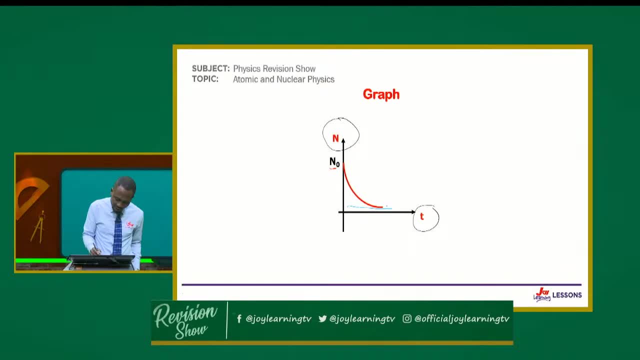 as time moves on. so, from here time axis, we are going forward this way. this n naught is rather coming down, it's reducing, it's coming down. So it's telling you that the initial amount of the radioactive nuclei present 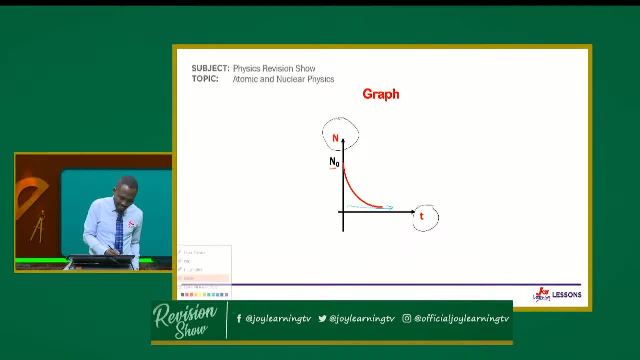 which is the n? naught, is decreasing decreases. okay, it's decreasing like that as time progresses, And that's how the graph could be interpreted. Now we can move on to half-life, Half-life, The half-life of a radioactive element. 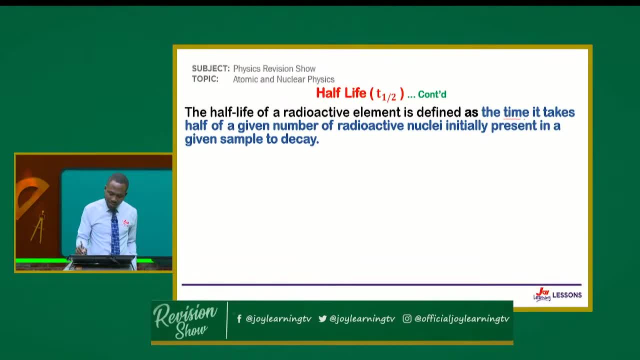 is defined as the time. so you see now half-life is time It takes half a given number of radioactive nuclei initially present in a given sample to decay. The time that it will take half of a given number of radioactive nuclei initially present. 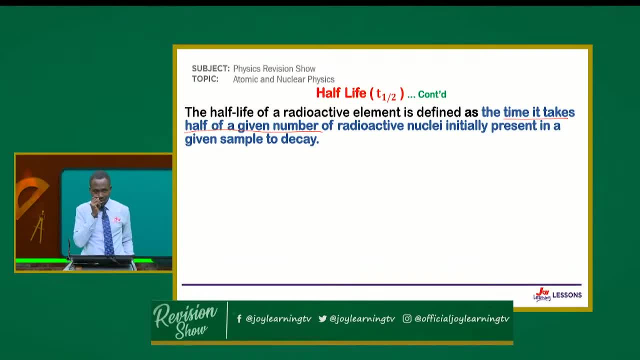 in a sample to decay is its half-life. So just imagine if you knew your half-life as a human being. If you know that maybe your half-life is, let's say, 60 years, Ooh, then you are blessed. It means that it will take you. 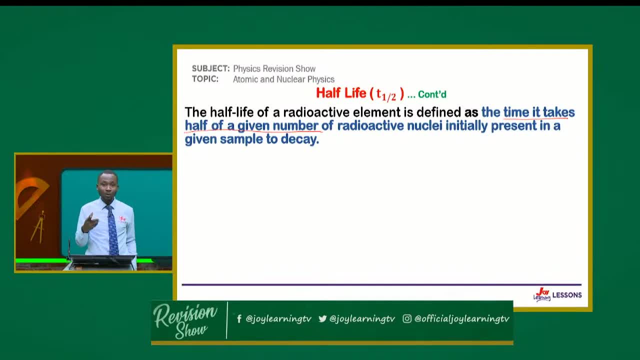 60 years for half of your life to go away. So probably you are going to live for 120 years. That's quite huge Anyway. so now you have a radioactive sample. Let's say it has got 20 atoms. How long will it take it? 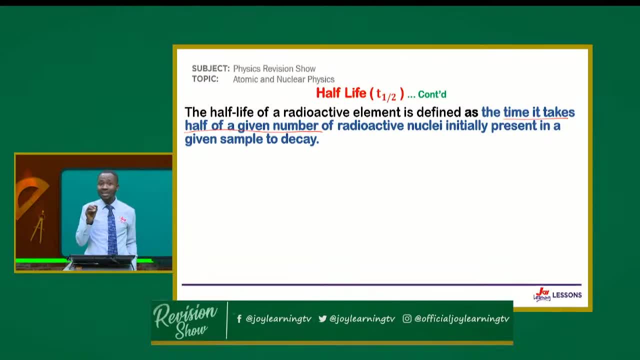 for 10 of the atoms to decay, That becomes its half-life. So the time it will take half of the initial amount of radioactive nuclei present in a given sample to decay. is its what half-life? And we will use that one with T. 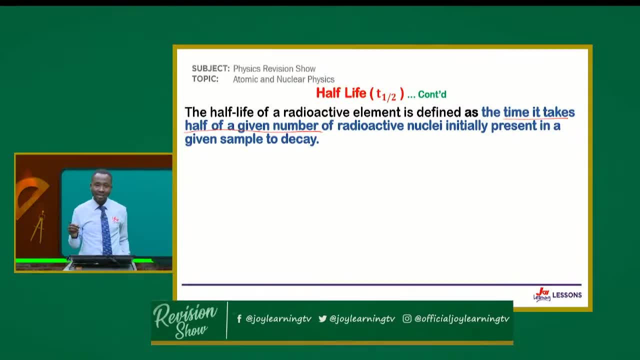 subscript half. Our other test will make it a capital T subscript half. So that's half-life. So mathematically you're going to get: half-life is equal to natural log of 2 on the decay constant Lin 2. 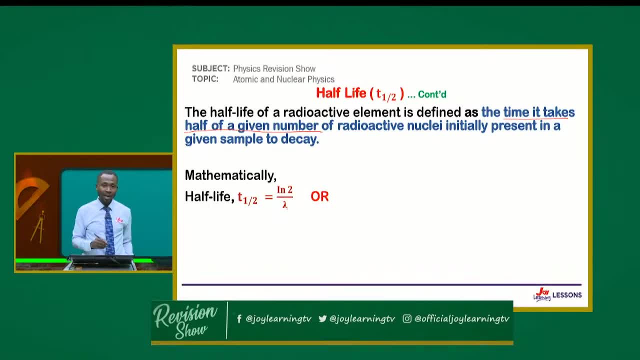 on decay constant. Now lin 2 is on your calculator. It's a first function, So you will see a button with IN. That's natural log like that on your calculator, like this: If you press, you can try it right now at home. 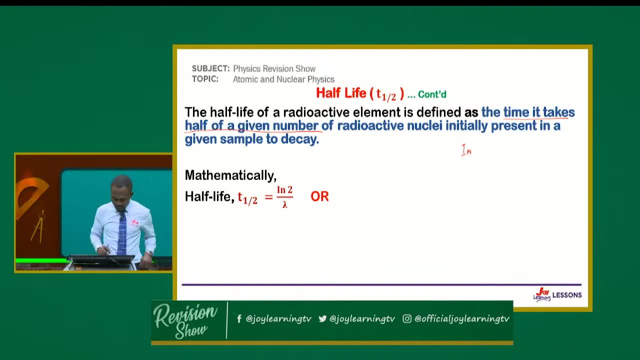 and let's look at it. So if you press that, what are you going to get? Natural log of 2,, so lin 2.. What are you getting So that we get to know the other expression for half-life? So I'm getting. 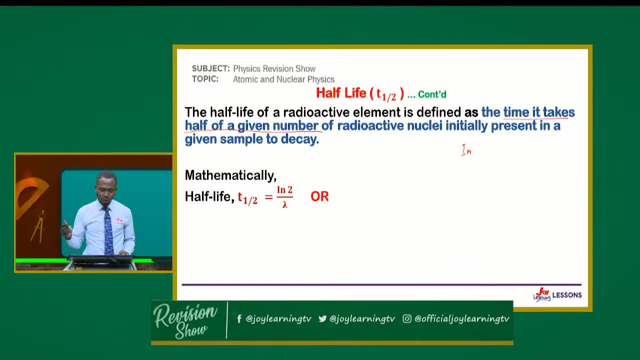 0.69314. blah, blah blah. So, instead of writing, half-life is equal to natural log of 2 on wavelength. it's lambda. it could also be half-life: t half is equal to 0.693 on lambda. 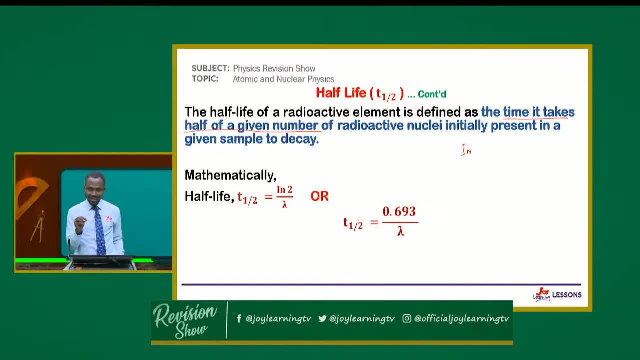 If keeping figures is quite difficult for you, then stick to in 2, stick to natural log of 2 on wavelength, because you have your calculator with you and you can always press point natural log of 2 and get a value 0.693. 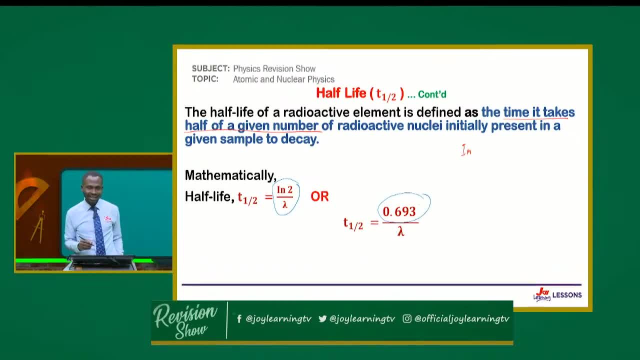 on the decay constant. That's our expression for half-life. This one, too, is very important, and you don't have to lose it, because if you lose it, you may not be able to solve any question when it comes to decay constant. half-life decay probability. 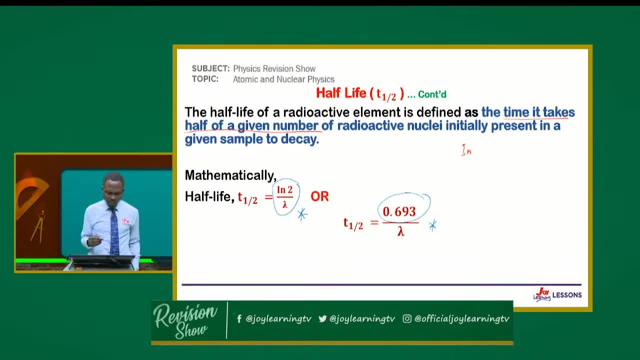 and then the law of radioactive decay. Now we can be asked to show why half-life is equal to natural log of 2 on the decay constant, which is lambda, or 0.693 on lambda. So let us try and look at the proof of that. 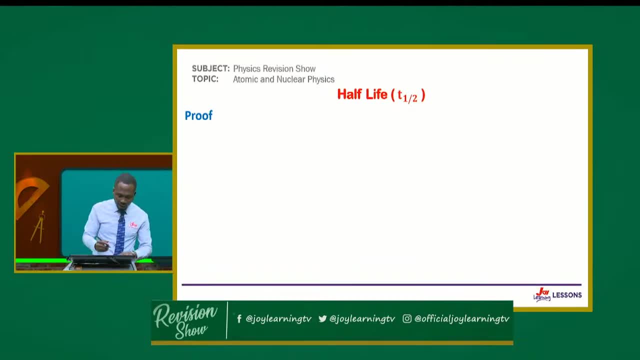 So we are going to prove why or how come you have. t half is equal to natural log of 2 on the decay constant. So let's set the ball rolling. We come across the decay equation, which is: n is equal to n. naught e. 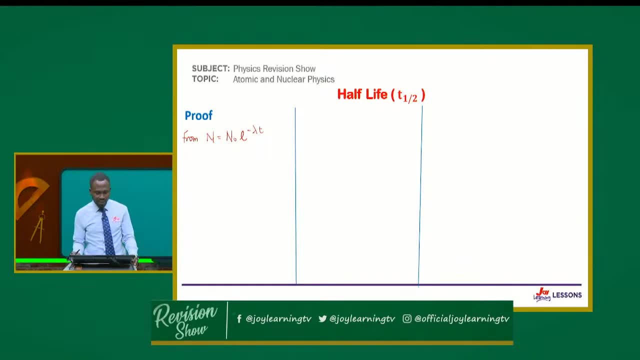 minus lambda t. So we got this as a decay equation right. So after a period of half-life, what happens? We are saying that half-life is the time it will take half of the radioactive sample present initially to decay. So 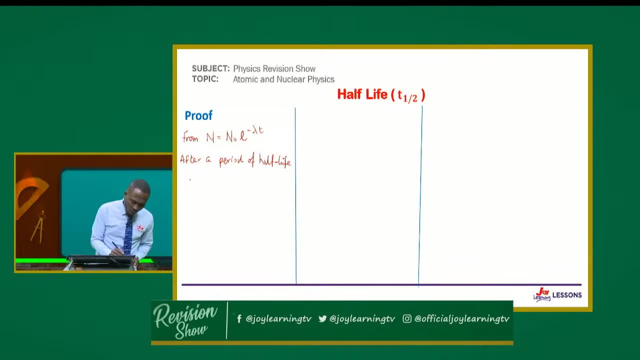 after a period of half-life. if still our n is the amount of radioactive nuclei present after the time of decay and n naught is the amount present initially for decay, then what will be left after half-life? what will be left which is n? 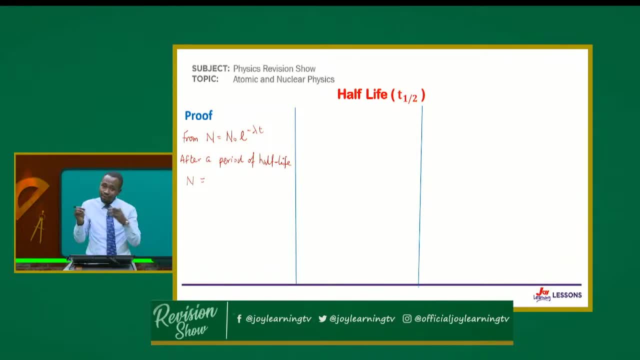 will be equal to what we had initially. half of it So, like half of what I had initially is the same as n naught on 2.. So you have to get this straight. Half-life here is telling us time that it will take. 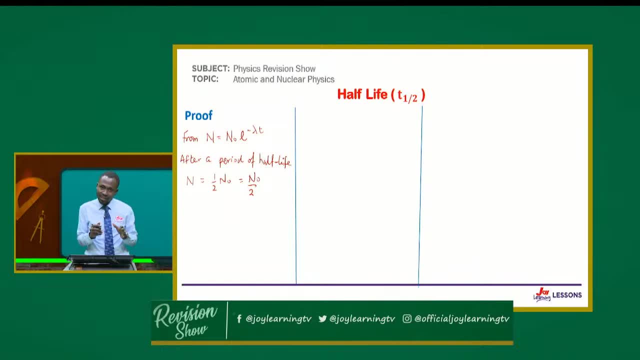 for half of any amount of radioactive nuclei present to decay. okay, And here we are using n naught to represent the total amount of radioactive nuclei that we have present initially after decay. So n is representing what you have left after decay. 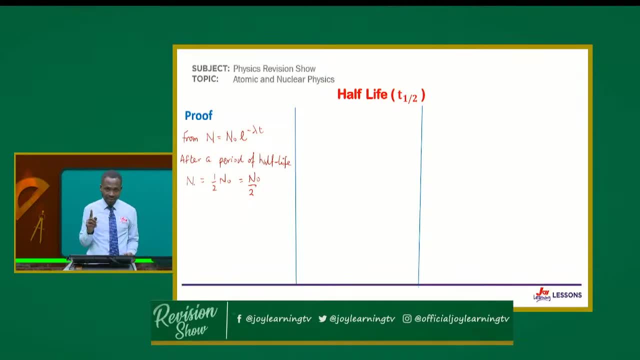 So after half-life, half of what we had initially will be left. So what is left? n is equal to half of what I had initially, which is equal to n naught on 2. Then the time will now become t half. 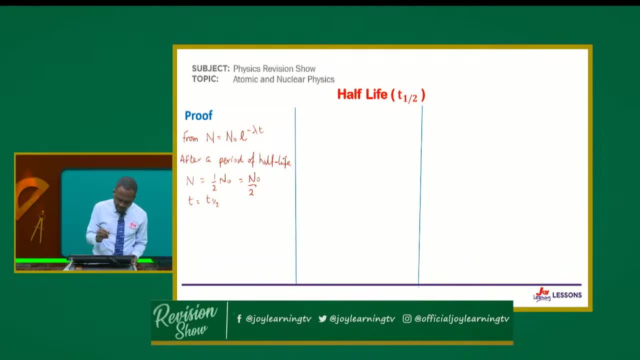 because it's half-life, So let's put this back into our decay equation. So we have n naught, So I'm going to get n naught on 2.. n has now turned into n naught on 2.. 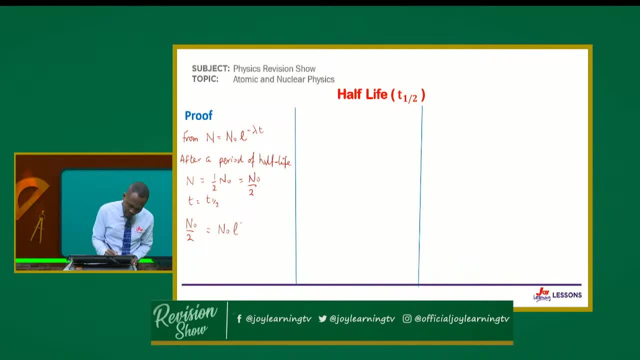 So in place of n, half n naught on 2 is equal to half n naught. the exponent minus lambda t is now t half. So t half right Now n naught is equal to 1 on 2,. 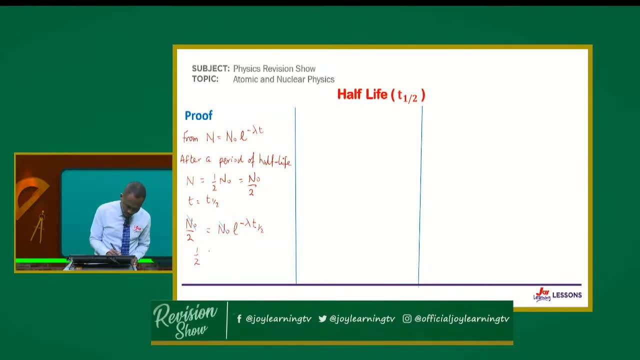 right, It's equal to e minus lambda t half. I don't want to be keeping the negative sign here, So if I should make all this denominator, I'll be able to do the negative sign. So I'll get 1. 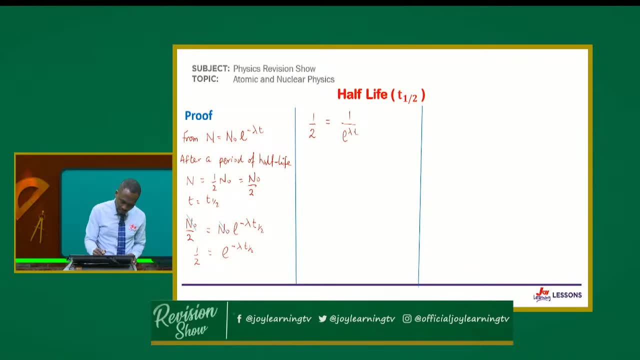 on 2.. 1 over e- lambda t half. Is that okay with us? So on my left hand side I have 1 over 2.. On my right hand side I have 1 over e to the power- lambda t. 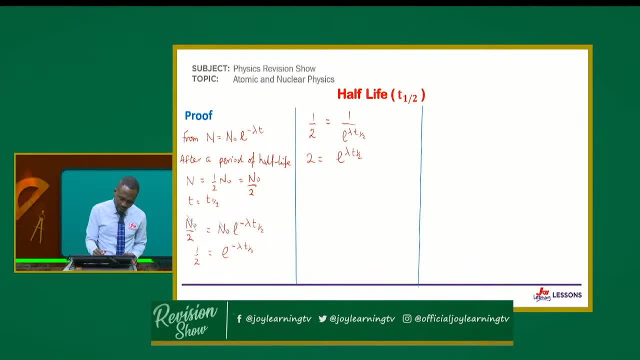 half. So in that case I can just pick the two sides of both sides, In other words natural log of both sides. that's what we call log to base e. So if I have log 2 to base e, 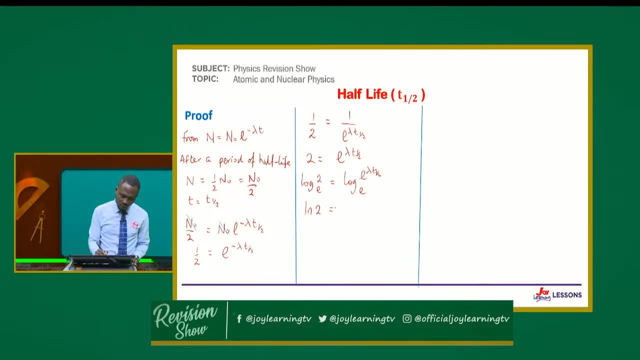 then here I'm going to get log e t half now log e to base e. So log e to base e will give us 1.. Right, So we're going to get natural. log of 2 is equal to lambda t half. 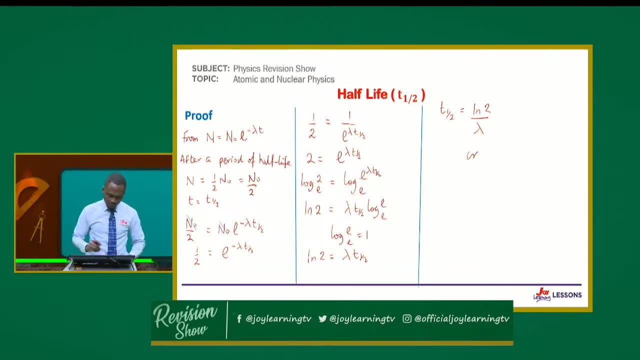 Good, Or, since we know what we can get, what natural log of 2 is, then t half will give me: with the calculator you can get natural log of 2, 0.693 on lambda, So that's equal to 0.693. 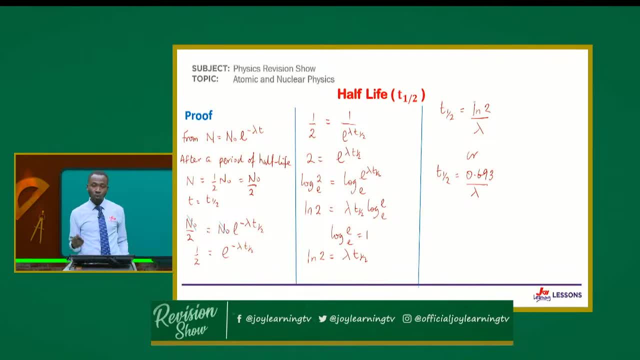 on the decay constant or natural log of 2 on lambda. I am pretty sure that when you are asked to show why t half equals 0.693 on lambda or t half equals 0.693 on lambda, So we have to solve. 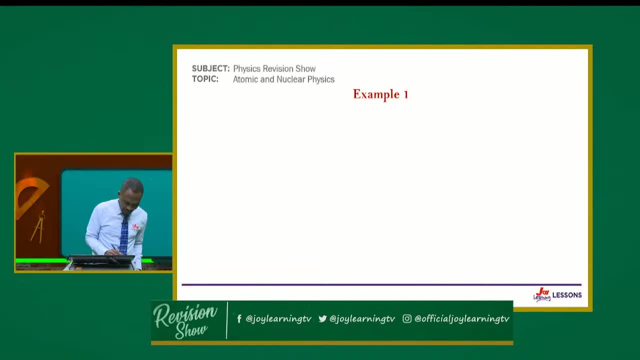 one or two questions based on all that we have gathered so far. I want to see whether we have got the answer or not. So let's see if we have got the answer or not. Let's see if we have got the answer, or? 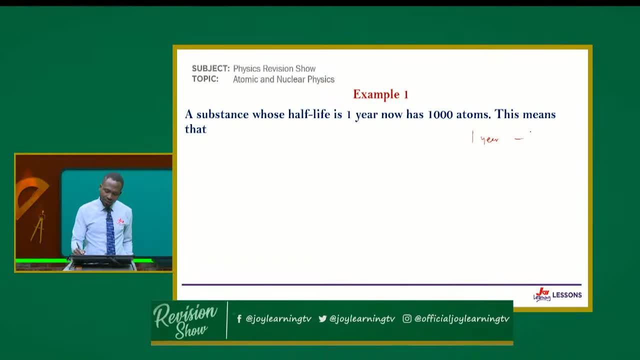 not. Let's see if we have got the answer. So after the next one year, which is now two years time, know that every one year half of whatever is left will go. So after one year, again half of it. 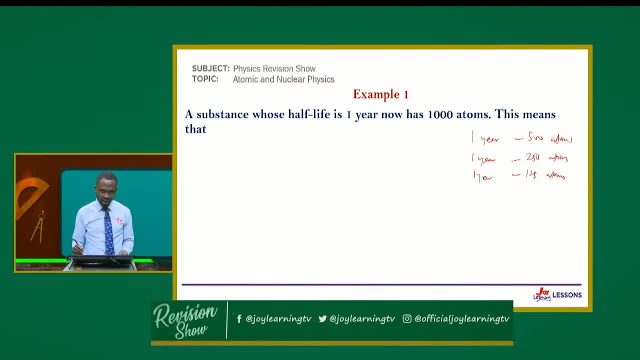 is the one thousand that we have now, So one year ago, half of it is the one thousand that we have now, So one year ago half of it will go and now you have one thousand, So one year ago. 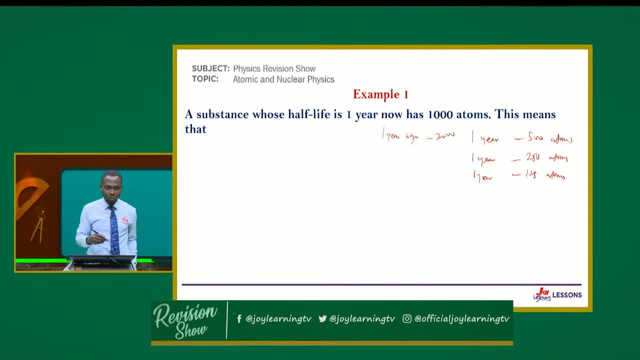 we had two thousand atoms of it. It's half life, It's one year, So after one year it has two thousand atoms. So in that case let's look at the options, Option number one One year ago. 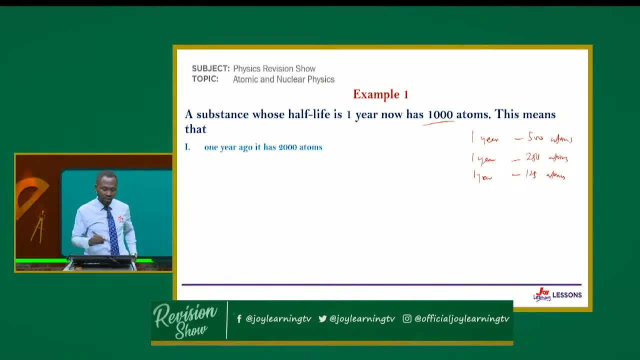 it has two thousand atoms. Is that true? It had four thousand atoms. Okay, let's just try and see: One year ago two thousand atoms. Now, after one year, one thousand. So half is gone Two years ago. 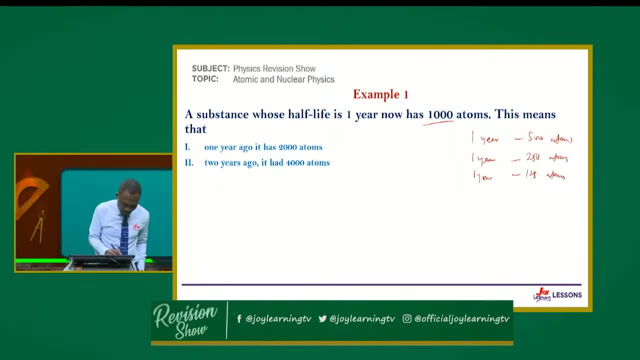 it had four thousand atoms. In six months' time it will have five hundred atoms. Can that be true? Now it has got one thousand atoms right. In one year half of it is gone. I don't think it is true. 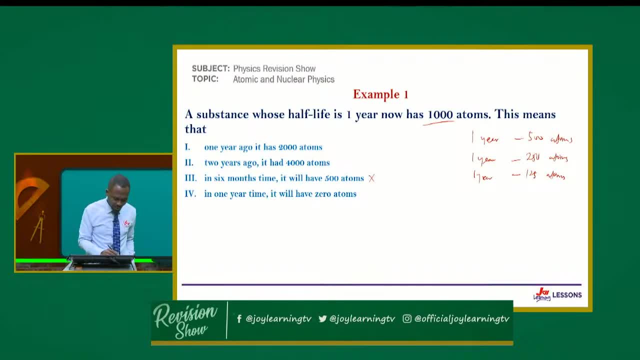 Now, in one year time it will have zero atoms. Really, I've done this here. One year to come: if now it has three thousand atoms, it will have six thousand atoms. The answer is A I and I, I only. 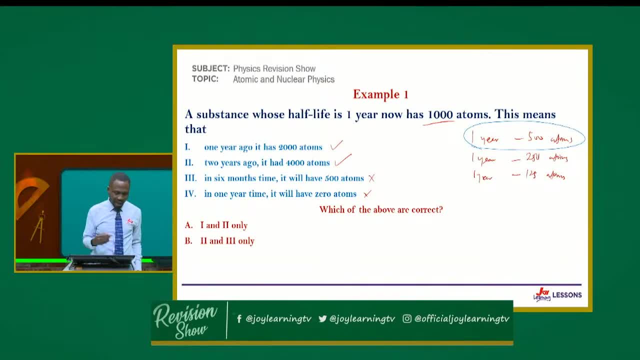 That's interesting. B- I, I and I I, I only, So I only. C- I, I, I and I V. Both of them are not correct, Do not feel for it. And D- I, I, I, I, I, O only. 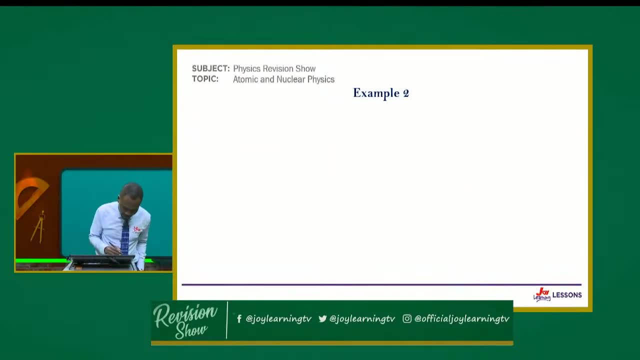 It cannot be so. I have an example two for us to look at. What does it say? Ooh, it's a diagram: 20 grams going to 10 grams, going to 5 grams. Then it says one year, two years and three years. 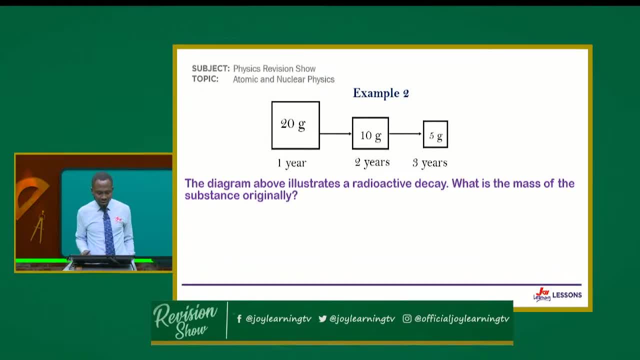 Okay, What do we have to do? It says: the diagram above illustrates a reactive decay. Okay, what is the mass of the substance originally? Hmm, originally, So one year ago, or after one year? we have 20 grams of the substance. 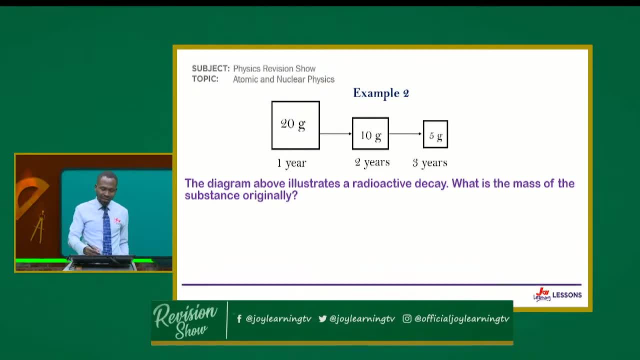 After two years it has decayed to half. Now you have 10 grams. After three years it has decayed to half of what we had After two years: 5 grams. So 20, half of it 10, half of it 5.. 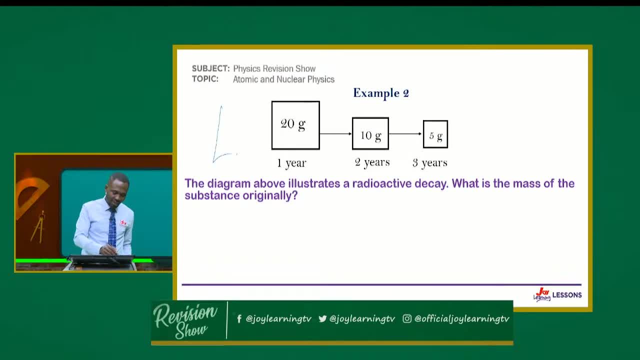 So before, before then, there should be something here. You can guess it. This half of it gave us this, Half of this gave us this. So it means that whatever answer we get here, half of it should give us 20.. 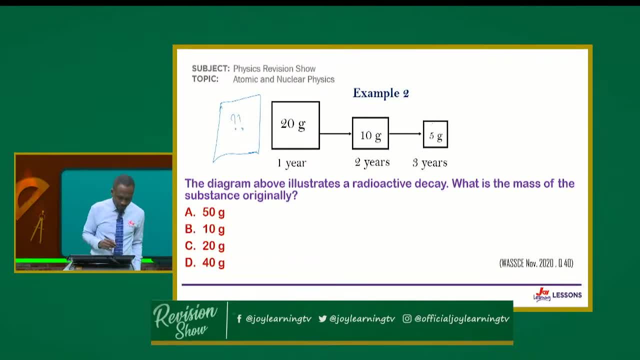 It follows that logic. Let's look at our possible answers. Ooh, 50.. Half of 50, will it give me 20?? No, So this will be out 10.. Half of 10, will it give me 20?? 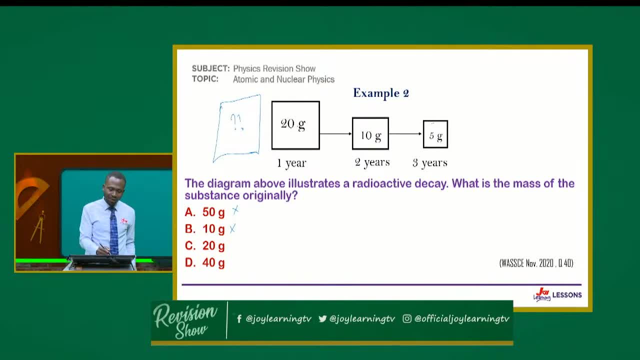 No, This will be out 20.. Half of 20,. will it ever give me 20? Out 40. So if we put 40 here, then half of 40, 20.. Half of 20, 10.. 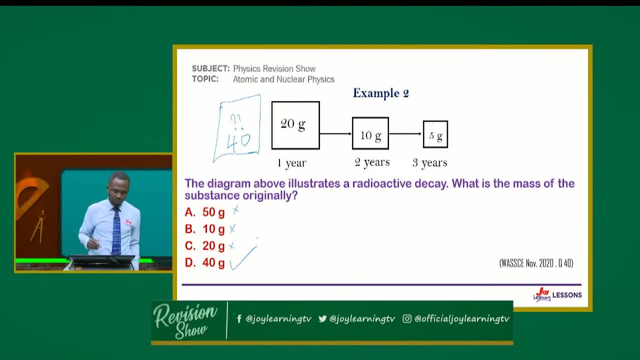 Half of 10.. 10, 5.. So 40 grams will be the correct answer. This is WASI Private Exams 2020.. So I believe you have been able to understand all that I'm trying to talk about as far as half-life is concerned. 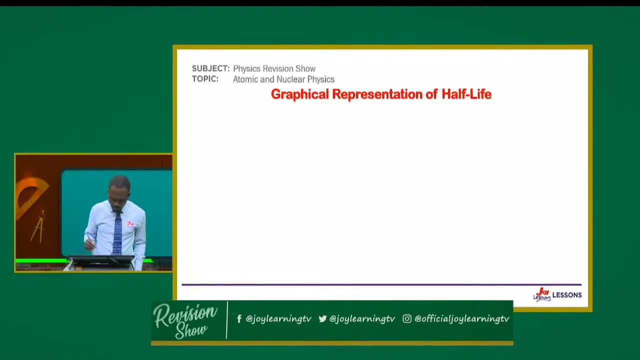 Good, Let's move on Now. I want to take my time and go through the graphical representation of half-life So that we try to see if we can use this to get some other things for ourselves. So I want to draw a graph of I'm going to get the vertical axis and then I'm going to get horizontal axis, like that. 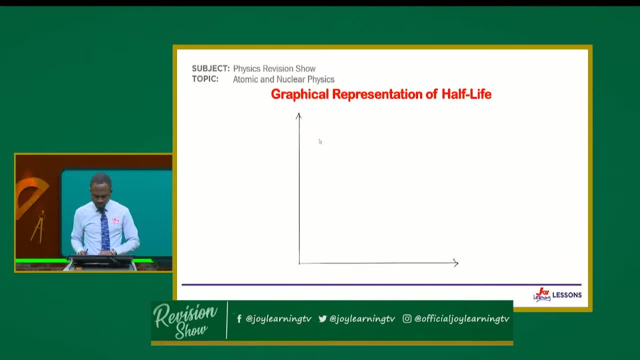 I'm going to label my graph And here I have the amount of the active nuclei initially present. Okay, Then not. Then I have time, So let me draw my graph Like that. So I'm going to look at first half-life, second half-life, third half-life. 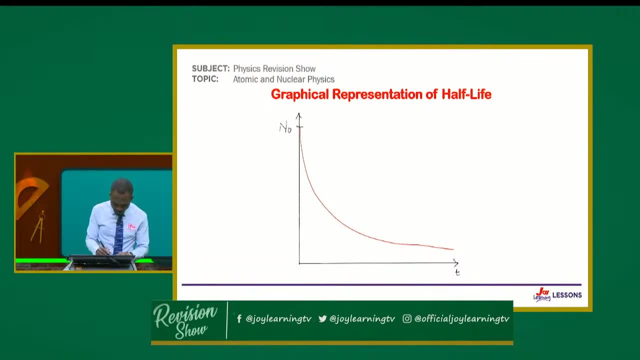 If possible, we go to fourth half-life. So I'm going to pick from here. So let me say T half and find out what will be left here. Then let me move to T2, or two times the first half-life. 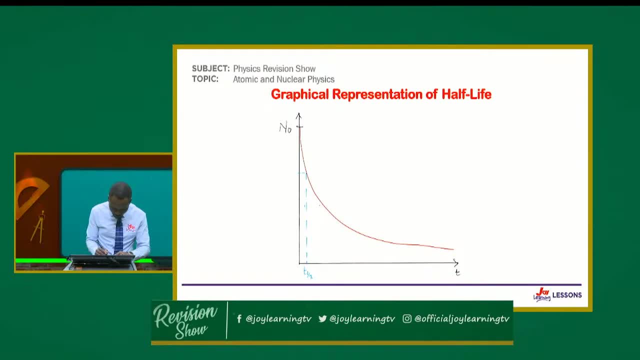 Right, So here there we go. So two times half-life- what happens? What will be left Then? let's move to three times half-life. What do we have Then? probably I'll end with four times half-life. 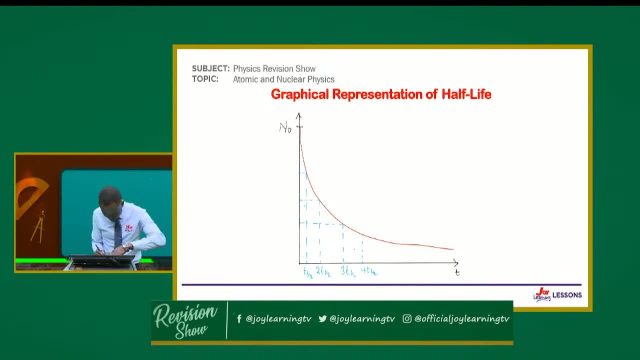 Four times half-life. Then we see what we're going to get. Okay, From our understanding, we are seeing that after the first half-life, for the first half-life we should have half of the radioactive nuclei originally present. half of it should be left. 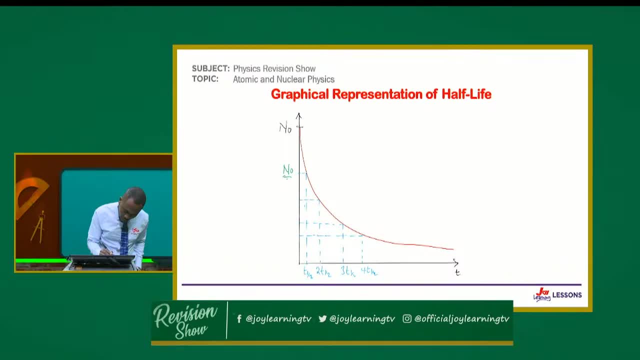 So I'm going to get N naught over two, N naught over two. So when our time is one, we have what is left to be: N naught over two. Okay, Now the second one, when our time is now two. 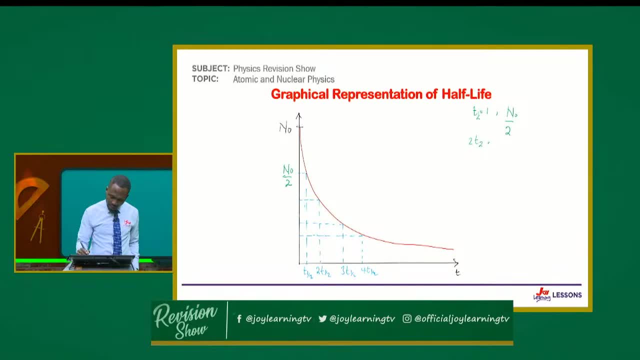 half-life. two times this, I'm going to get half of what is left. What was left is N naught over two, So that will give me N naught over four. So I'm going to get N naught over four. 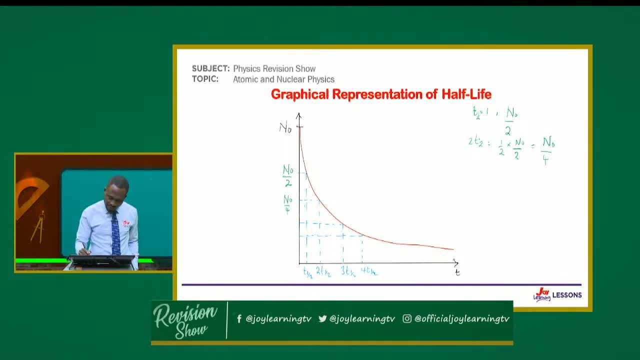 Are you getting this Now? third one: Three times the half-life. now is half of what was left, which is N naught on four. So times N naught on four, which gives me N naught on two times four. 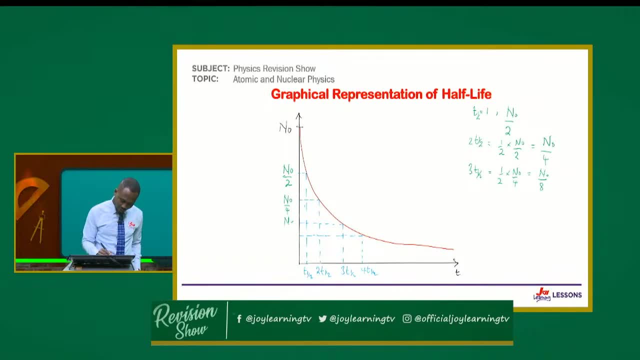 which is eight. So we're going to get N naught on eight. Last but not least, I'll just end with this one. Then if I have four times that, then I have half of what is also left here. times N naught over eight. 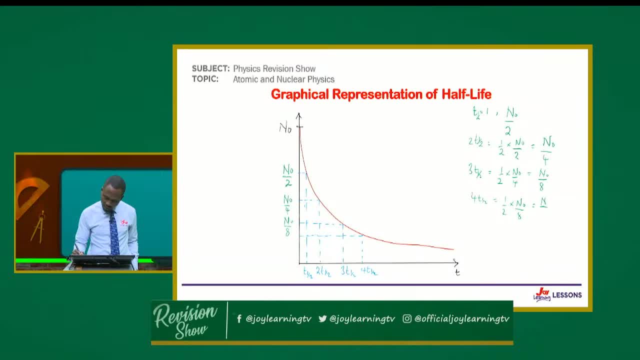 That gives me one over. sorry, N naught over sixteen, So I have N naught on sixteen. Are we seeing any expression, any trend? Yes, Here, I just have N naught over to the power one. Okay, 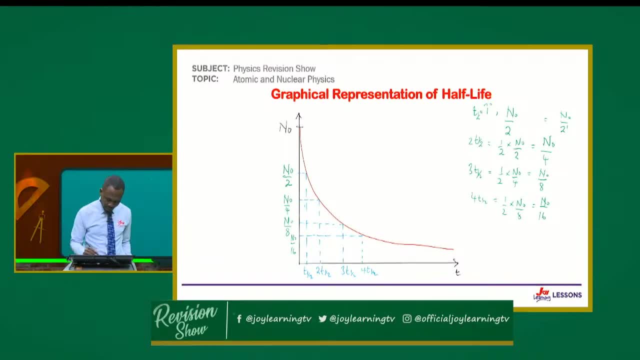 Here N equals one, So to the power. maybe, like this, N naught onto the power N, And here N is one. Here I can get N naught on two to the power two, because two times two, two squared, give me four. 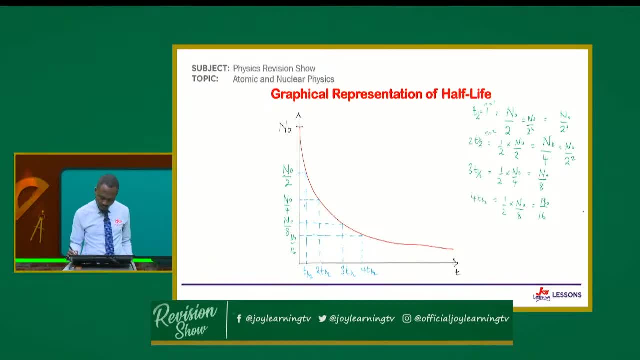 So here I'm getting N equals two. Then we get N naught on. this is eight. So two to the power three. Two times two, four times two, eight. So here I'm getting N equals three. 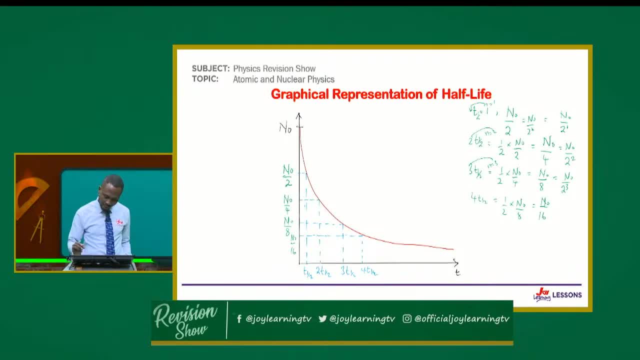 This, that That is one. Then here I'm going to get N naught on to the power: four. Two times two, four times two, eight Times two, sixteen. So here too, N is four, Like that. 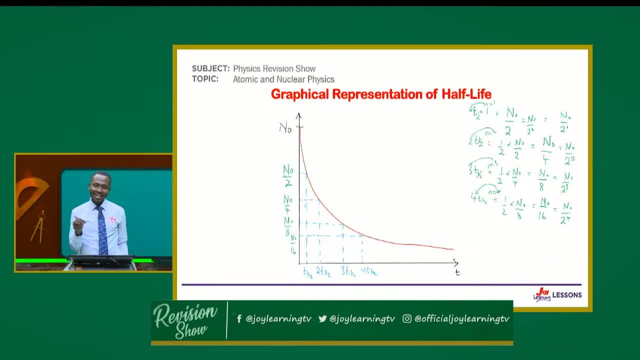 So out of this we can try and get an expression We are getting generally: we are going to get N naught whatever is left. N is giving us N naught over two to the power N, A very important relationship. 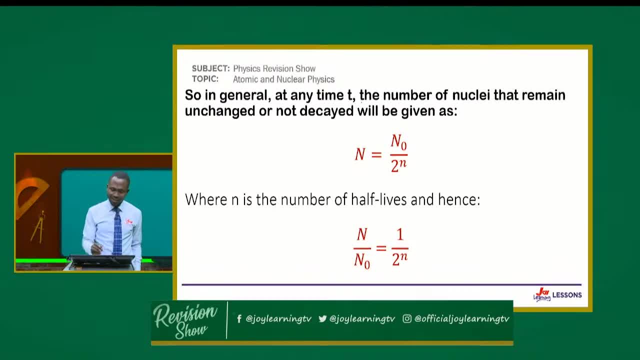 So that's it. So in general, at any time: t. the number of nuclei that remain unchanged or not decayed. the number of nuclei left yet to decay: N is N naught over two to the power N. 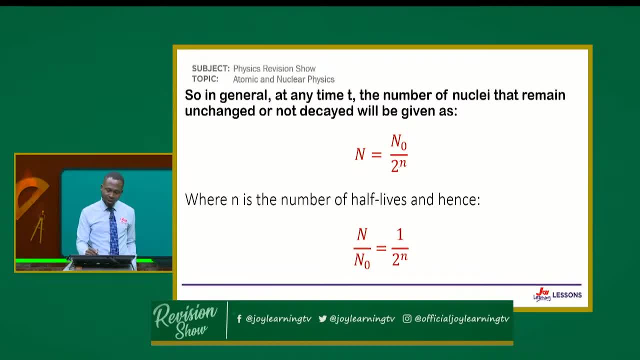 So when N equals one, when small N equals one, you're going to get N naught over two. When small N equals two, you get N naught over four. When small N is three, N naught over eight. If you should divide N by N naught. 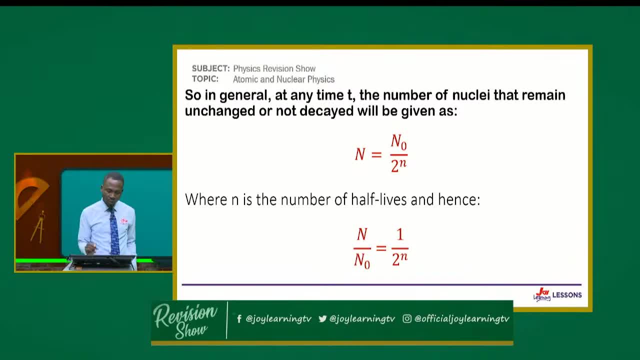 you're going to get N over N. naught is equal to one over two to the power N. This is a very important relationship. You have to take note of it. It will help you to solve number of questions as far as this topic is concerned. 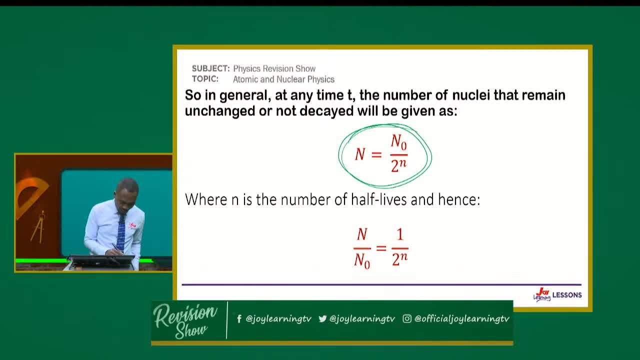 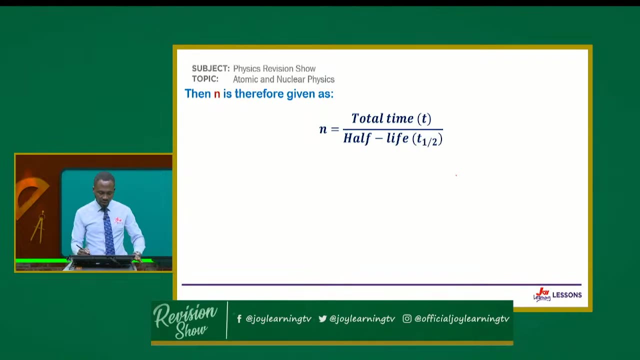 Good, It follows that what then will be N? N is equal to the total time over half-life, Total time on half-life. So N equals t on half-life. Okay, so let's move on. We can try and make t half. 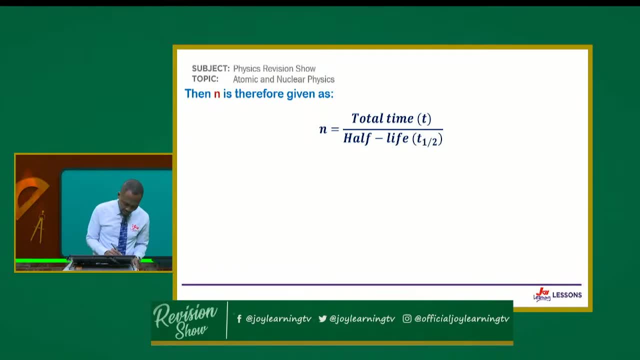 or the half-life, a subject. You're going to get N from N here that N equals t over t half, So t half will be equal to t over N. So the total time over N N Very important. 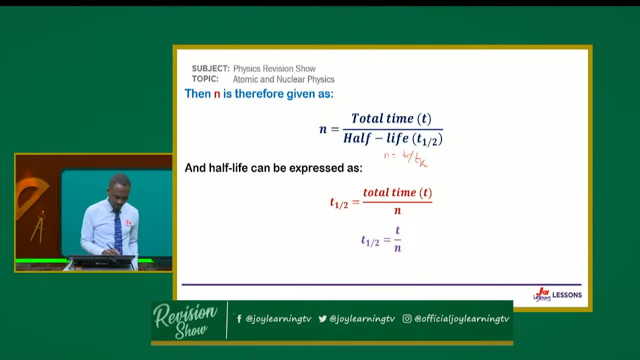 over the number of half-lives- Very important. Good, We can move on to what we call activity or decay rate. Don't forget we have looked at the N on the t, The rate of decay. So activity or decay rate. 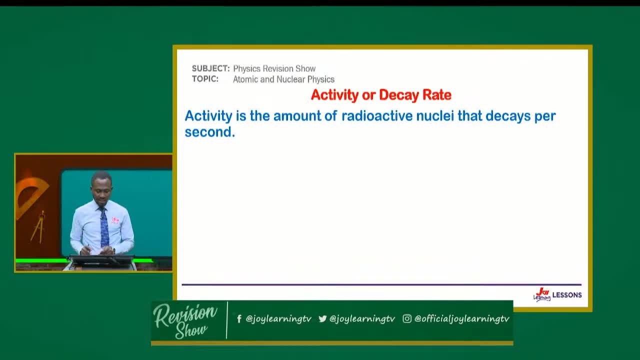 What will be our definition? It says activity is the amount of radioactive nuclei that decays per second. Activity is the amount of radioactive nuclei that decays per second. The amount of radioactive nuclei that decays per second is its activity. Or we can say: 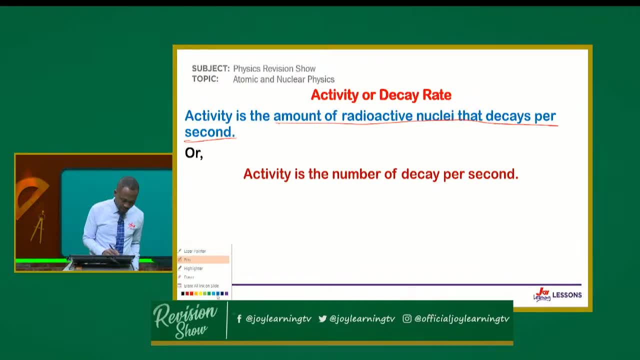 activity is the number of decay per second. Activity is the number of decay per second. So number of decay per second, simple terms, would be rate of decay. So activity, in simple terms, would be the rate of decay. So 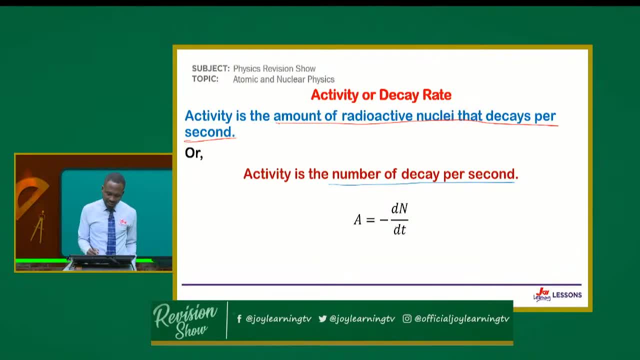 A is the N on the t And I believe you understand why the negative sign is there. As the time progresses, the activity decreases Because the amount that will be decaying per time will be decreasing. Half of the original will go, half of what is left will go. 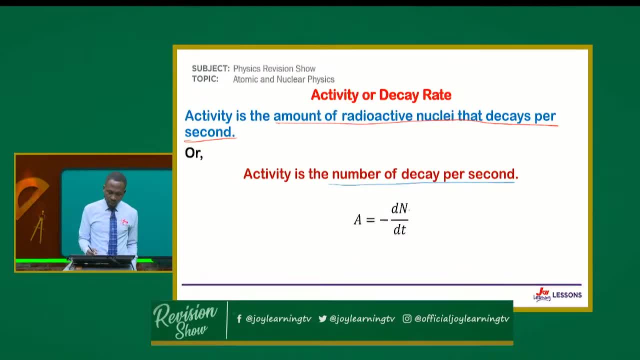 half of what is left will go and all that. So A is equal to minus the N on the t. The N on the t is rate of decay. So we can say that activity is the rate of decay, The amount of radioactive nuclei. 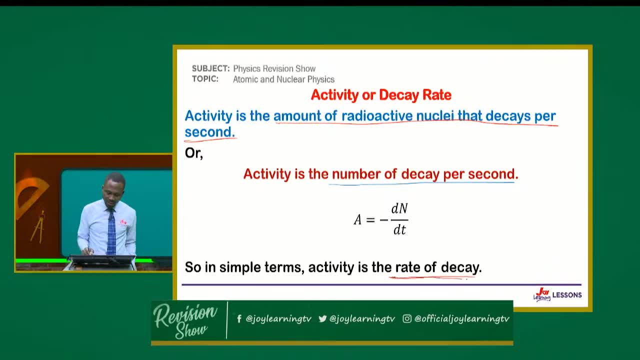 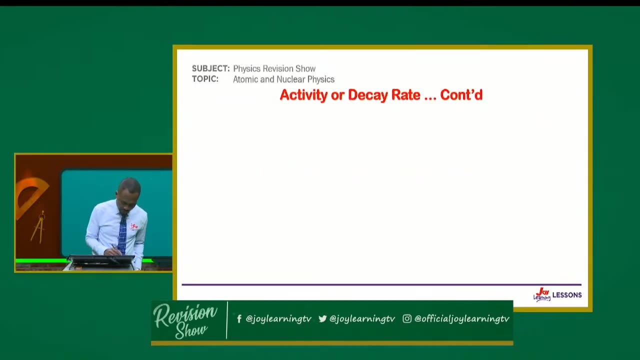 that decays per second. So activity is simply the rate of decay. So in place of the N on the t we could put A there, which is activity Right. The unit of activity is Becquerel, Named after the scientist. 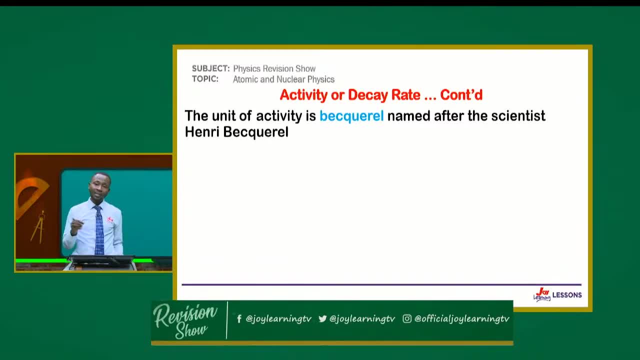 Henry Becquerel, So he could be asked in objective test, the one who propounded activity. So it's named after the scientist, Henry Becquerel. He brought about activity, Which is the rate of decay. So one Becquerel is equal to. 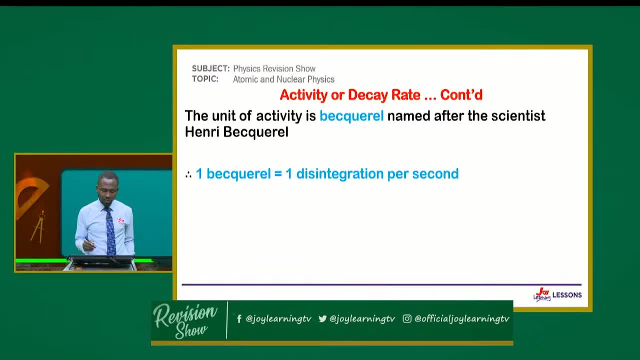 one disintegration per second. One Becquerel is equal to one disintegration per second, But usually, very often, the SI unit is per second. So when you are asked to calculate for activity, you leave your answer in the SI unit. 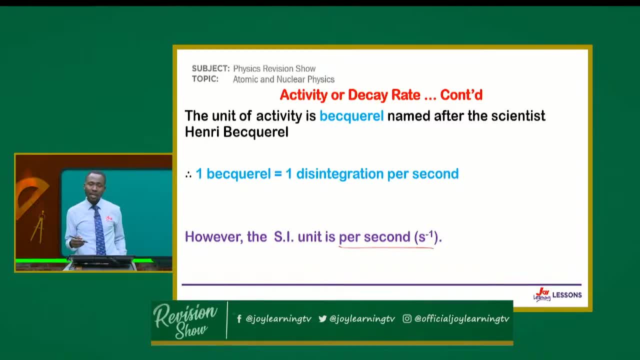 which is per second, But sometimes if the value of activity is given to you in a question, it may be given to you per week, per day, per month, per year. So there are other units that activity could be expressed in. 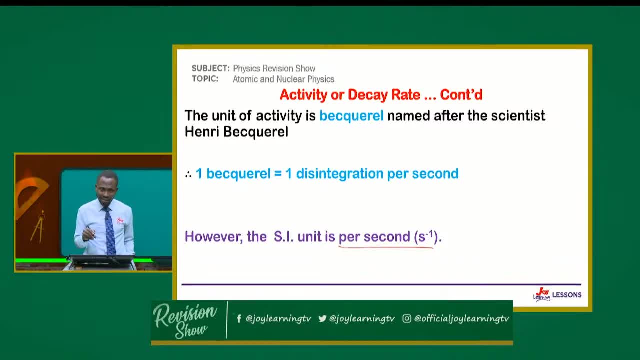 But when you are supposed to find the activity, you calculate for it, Then your answer you leave it in per second. Per second, So activity or decay rate, you are saying that from the N on the T it is proportional to N. 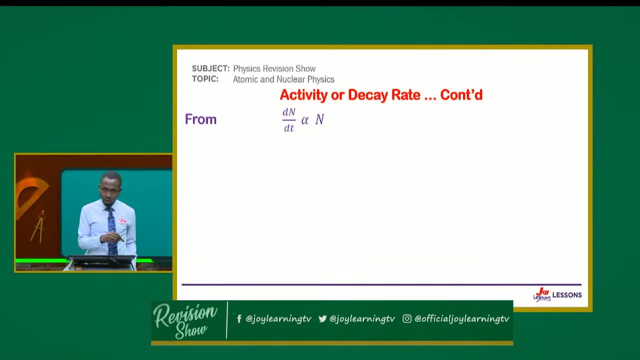 The very first thing. we began with the law of reactive decay. Now, from here, in place of the N on the T, we can put activity A there, because the rate of decay is the same as activity. So when you put A, 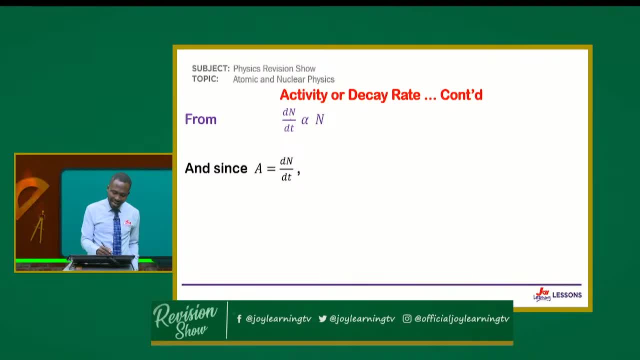 in place of the N on the T. you're going to get A is already proportional to N, So you're going to get A. activity is already proportional to N. In that case, when we take away the sign of partiality, we introduce an equal sign. 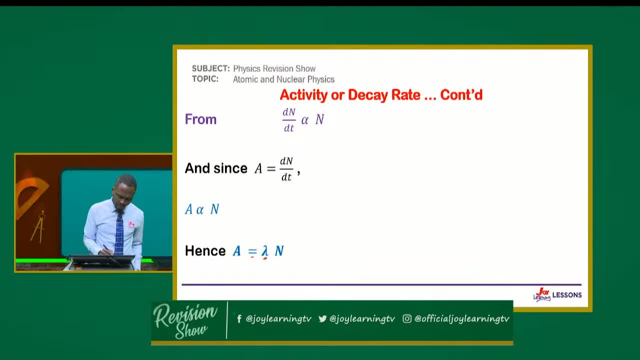 and then we bring a constant which is our decay constant. So A will give us equal to lambda N, A is equal to lambda N. Alright, Note if A naught is the initial activity of a radioactive element, the initial activity, 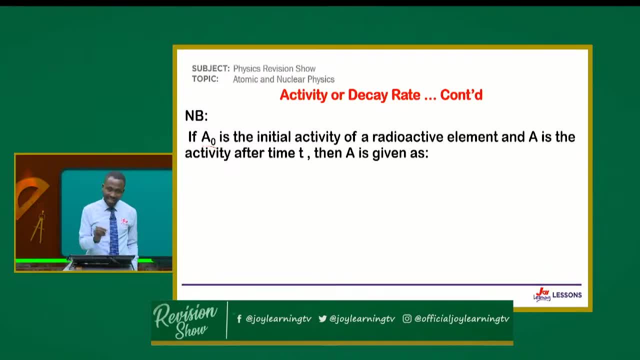 of a radioactive element is A naught, Just like we are saying that N naught is the initial amount of a radioactive substance present before decay And A is the activity after a time T. They are trying to write a decay equation in terms of activity. 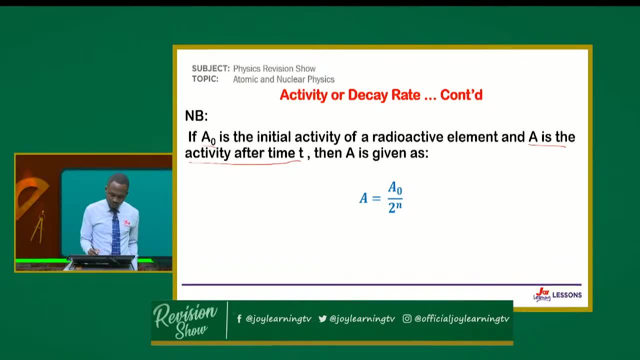 So then A will be given, as A is equal to A naught on 2 to the power N. Don't forget we had N equals N naught on 2 to the power N. Like this. So it means that in place of N, 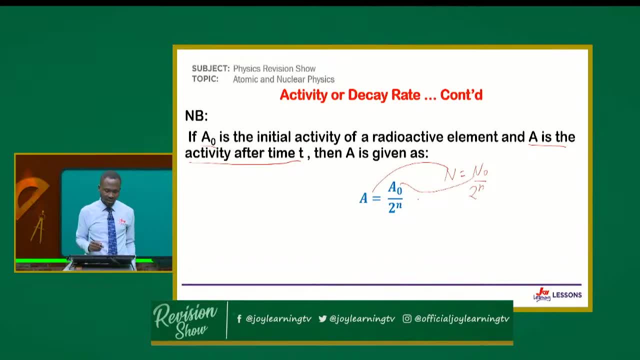 we are putting A is there In place of N naught. we have A naught Like that. So A is equal to A naught on 2 to the power N, And we know what N is Good, So we can write a decay equation. 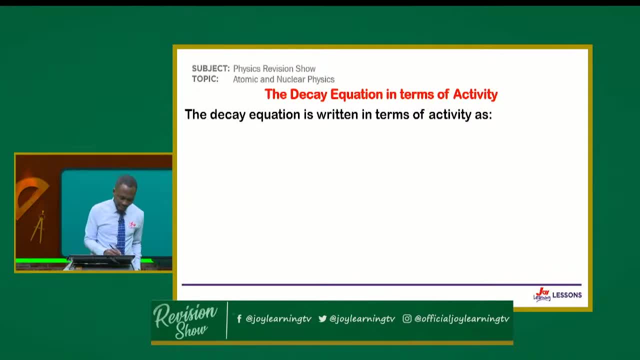 in terms of activity, as A is equal to A naught exponent minus lambda T, Similar to N equals N naught E minus lambda T. So we are only reporting N with A and N naught with A naught And any other thing. 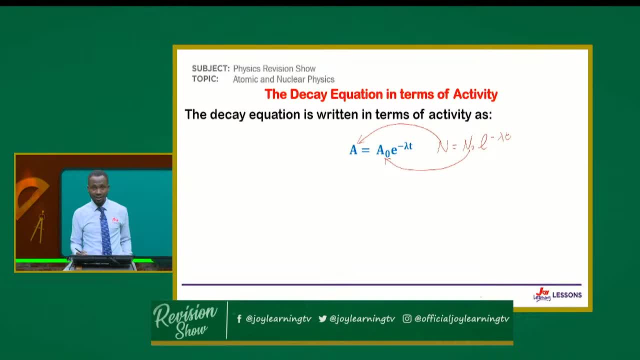 is the same. Any other thing is the same. So, depending on the question given to you, if it's in terms of activity, then you write a decay equation in terms of activity Like this: If it is in terms of, in terms of: 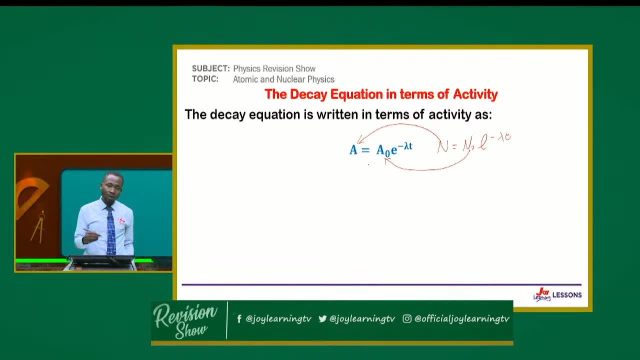 the amount of the active nuclei present, N and what is left. then you go to N and then A. So you can write a decay equation in terms of activity. So you can write a decay equation in terms of activity. 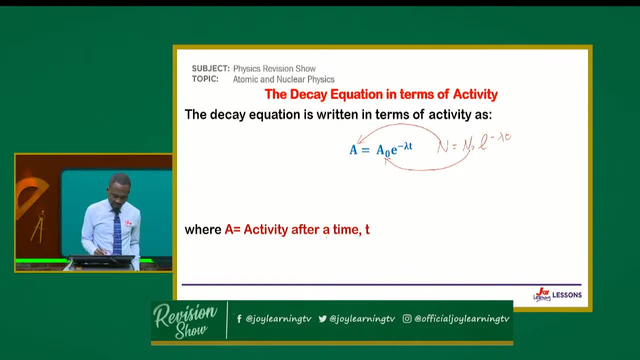 So A is N and then N naught, So A is activity after a time T, And then A naught is the initial activity, is the initial activity. So we can get a graph, just like we had a graph for. 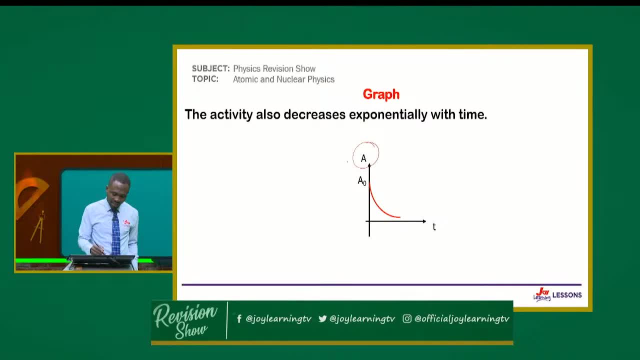 N naught. So A is activity left at the time, t is the initial activity and it says that the initial activity is decreasing, decreasing with time. So the rate of decay is decreasing with time because with time the amount that is left that is supposed to decay will also be decreasing, So the time at which it is going to decay it will be slowing down. it will be slowing down with time because the amount that is left will also be decreasing, becoming smaller and smaller with time. 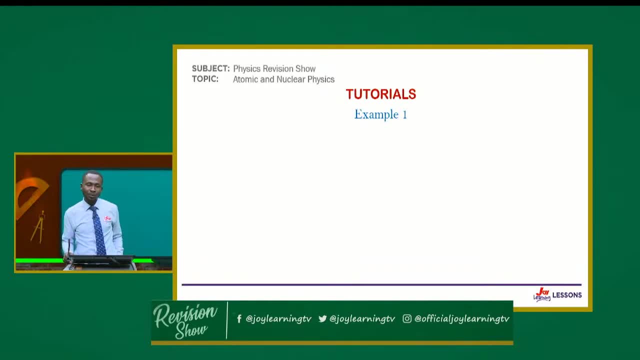 I think it is a good time to take a breather. We are going to take a breather, We are going to solve some questions based on things that formerly you have encountered, but I would like to go on a break, get something a little to sip, and then come back and then we continue. 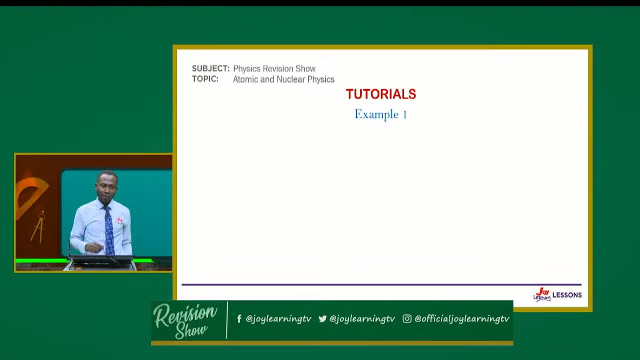 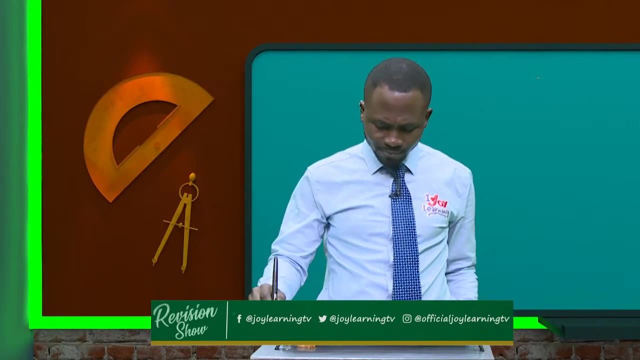 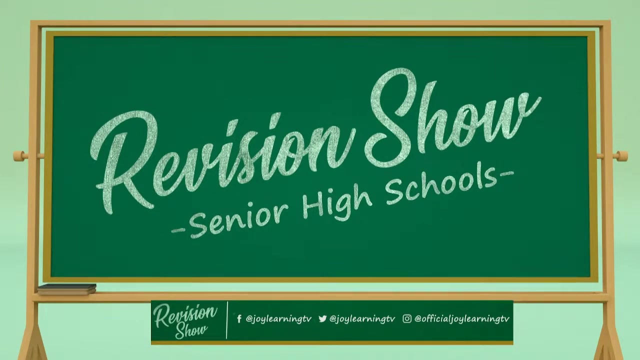 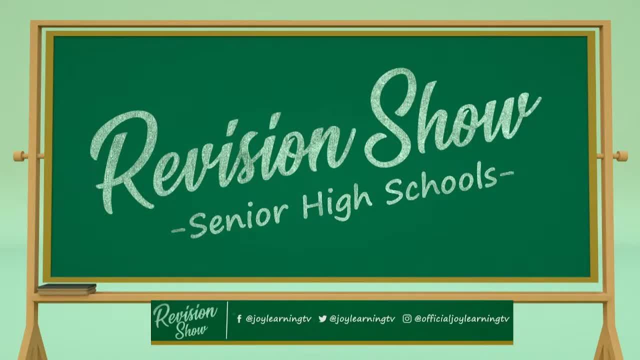 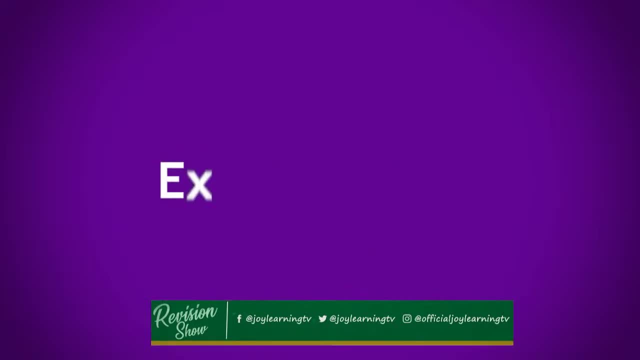 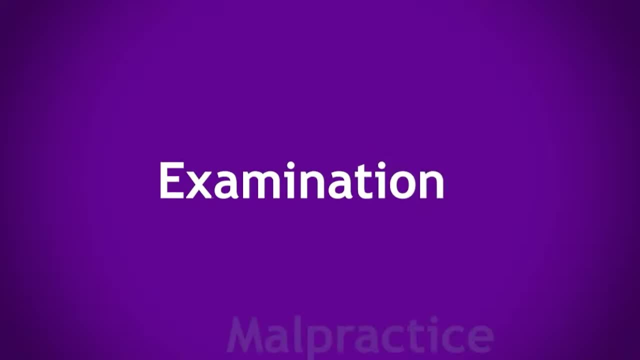 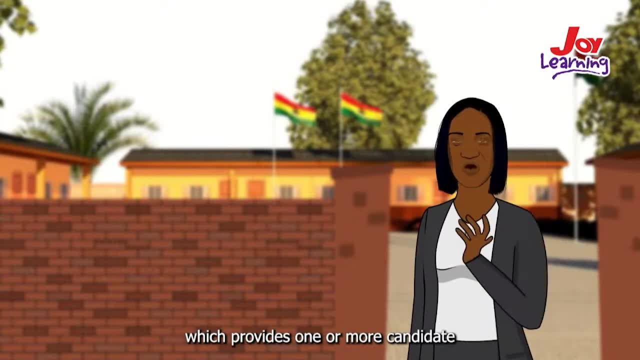 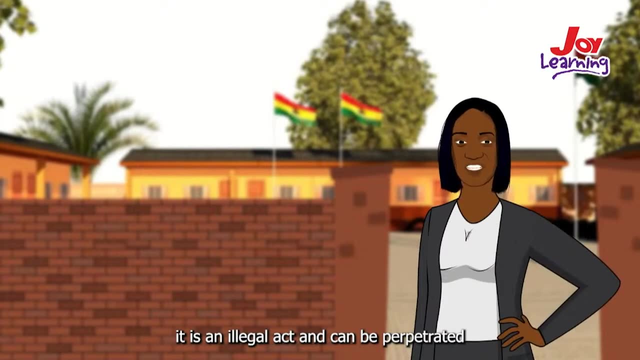 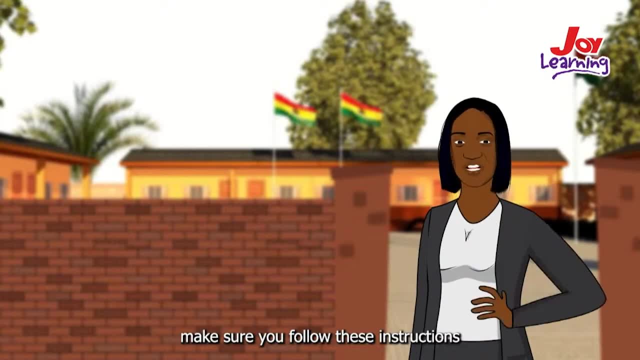 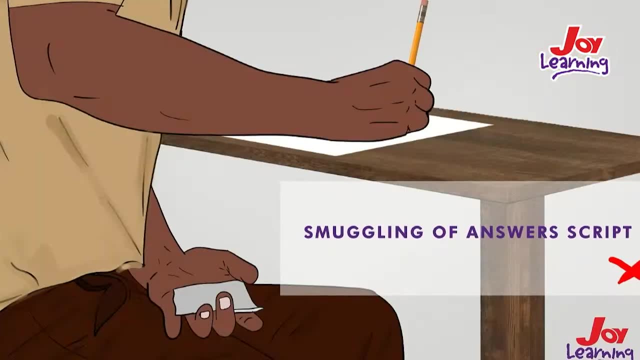 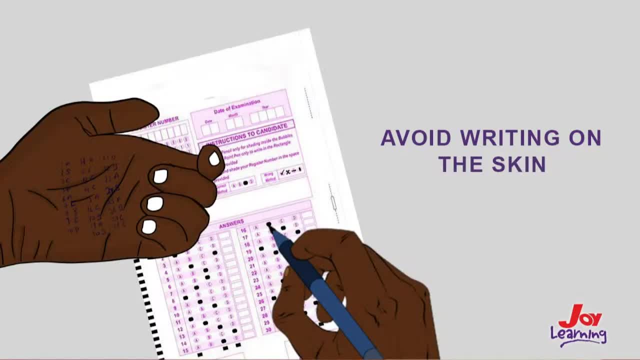 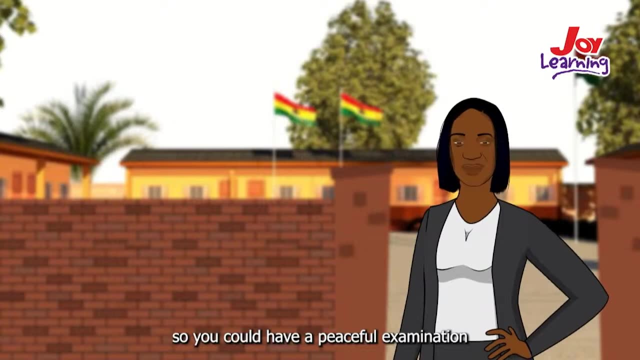 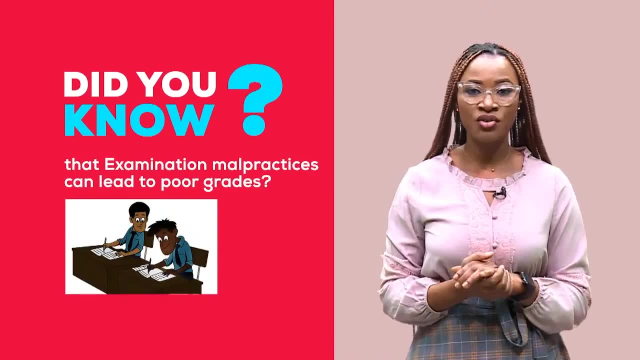 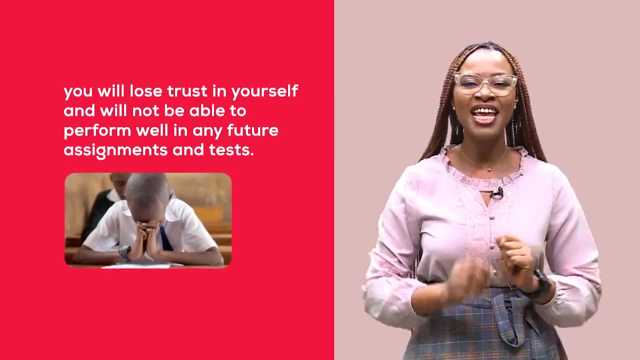 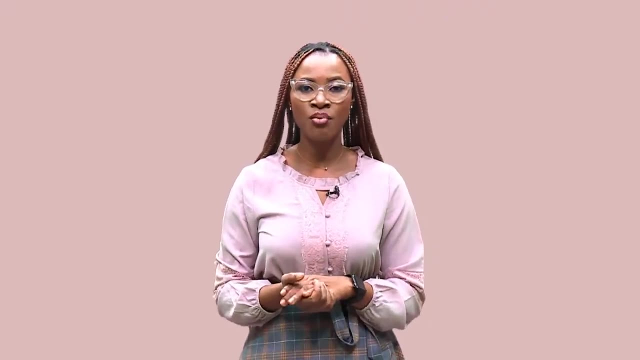 Did you Know that examination or practice can lead to poor grades? As a result of this, you will lose trust in yourself and will not be able to perform well in any future assignments and tests. So I'm here to give you simple tips on how to avoid examination malpractice. 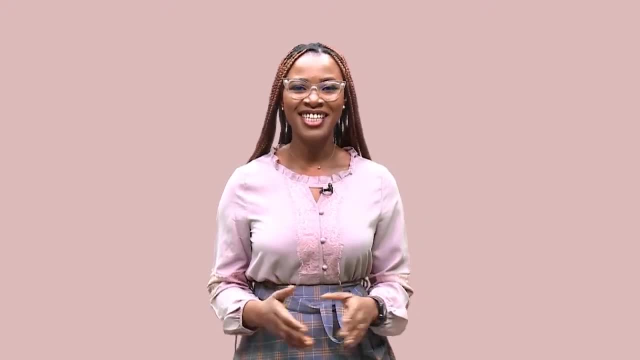 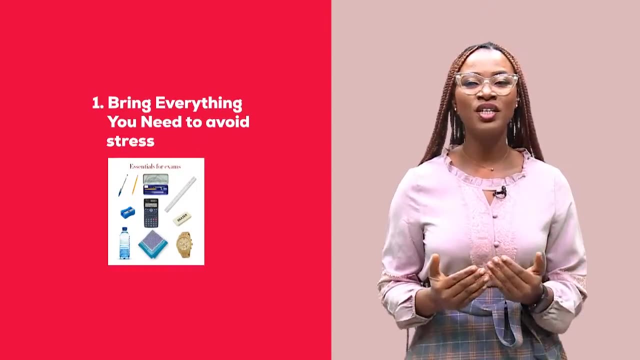 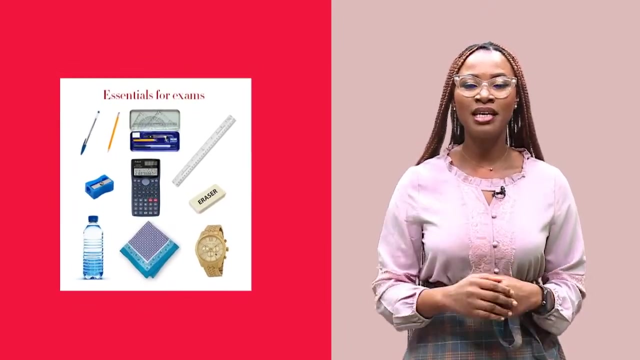 So let's talk about the do's in examination hall One. bring everything you need into the examination hall. It may sound simple, but a lot of stress can be avoided by making sure you have everything you need to do in the exam. Make a checklist the nights before each exam. 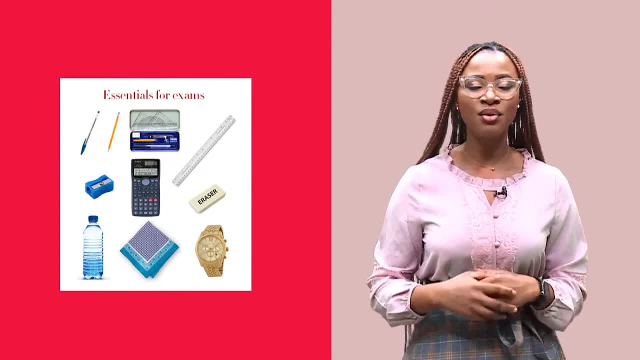 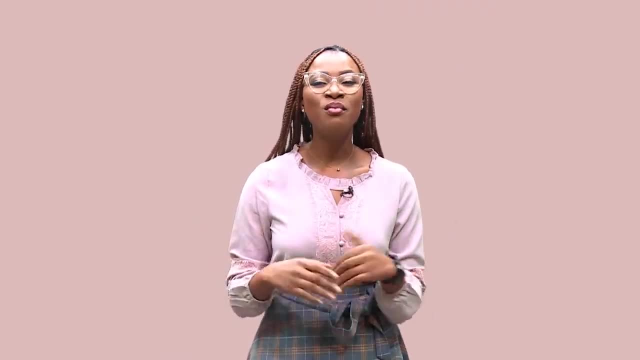 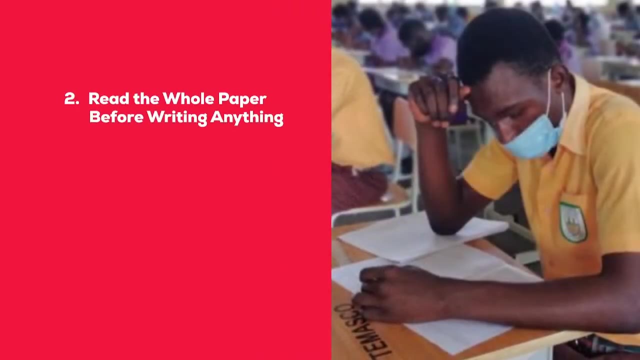 then go through it before you leave home and then again before entering the examination hall. Two: read the whole paper before writing anything. One of the most important exam preparation tips to dwell in during the run-up to exams: read every question before you start writing anything. 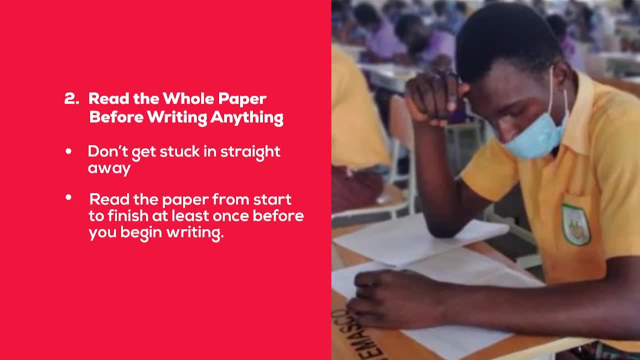 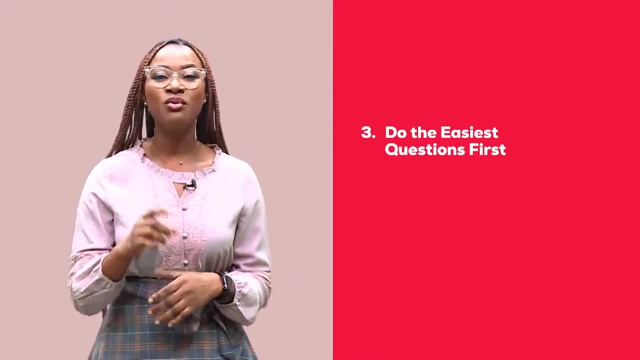 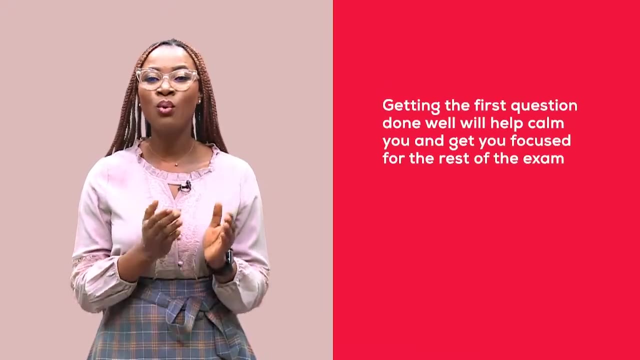 Don't get stuck in straight away. Read a paper from the start to finish at least once before you begin writing. Three: do the easiest question first. There is no reason to do the question in order. they are printed in the exam. Firstly, getting the first question done well. 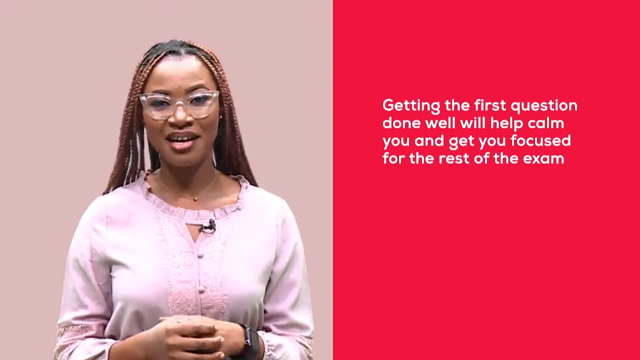 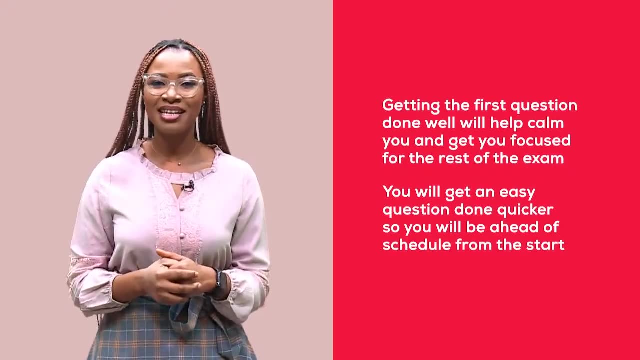 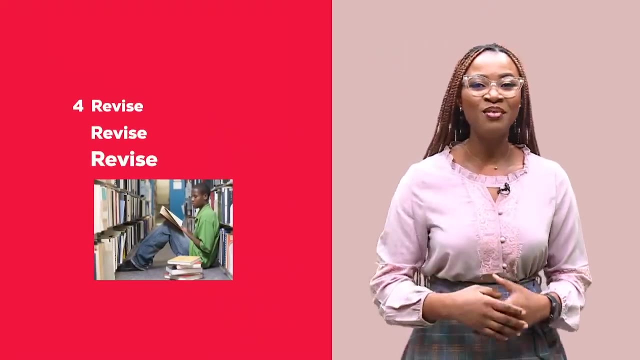 will help you, calm you and get you focused for the rest of the exam. Secondly, often you will get an easy question done quicker, so you will be ahead of schedule from the start. Four: revise, revise and revise again The nights before the exams is not the topic. 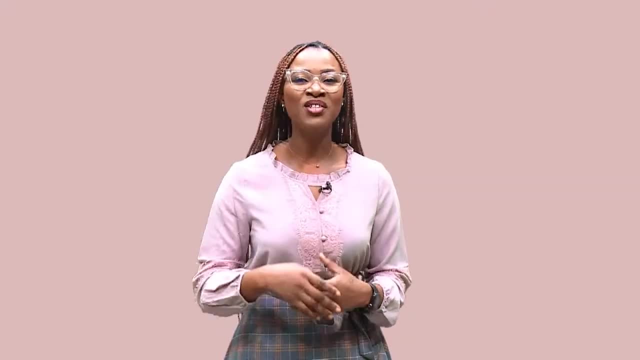 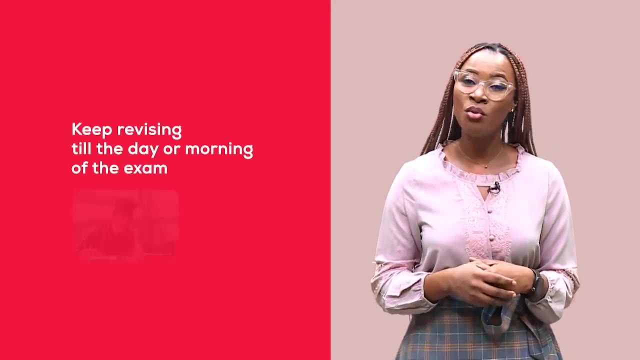 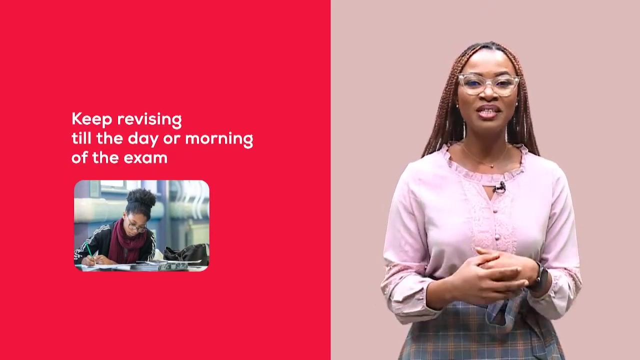 not the time to be trying to get your head around new concepts. Some students read and forget parts of the information during the exam. This is why you have to keep revising till the day or morning of the exams. This is one of the steady habits of highly successful students. Once you have become 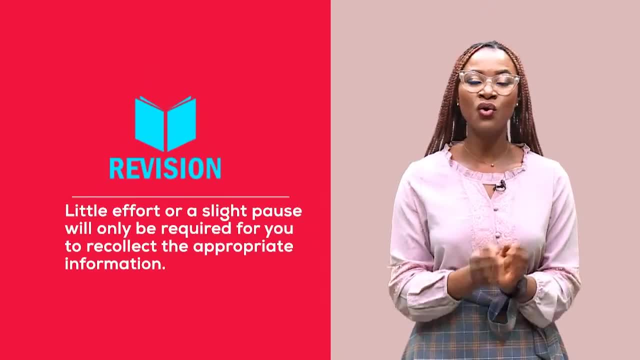 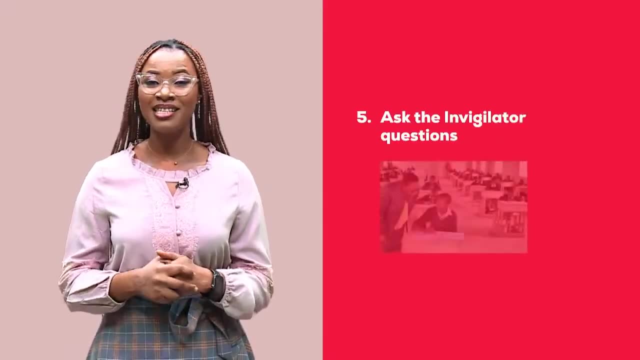 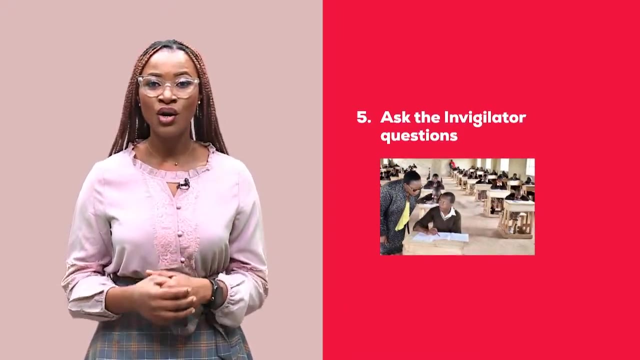 so complacent with your revisions, little or a slight pause will only be required for you to recollect the appropriate information. Five: ask the invigilator questions. If you are stuck on the meaning of a word or can't understand what a question requires you to do, put your hand up. 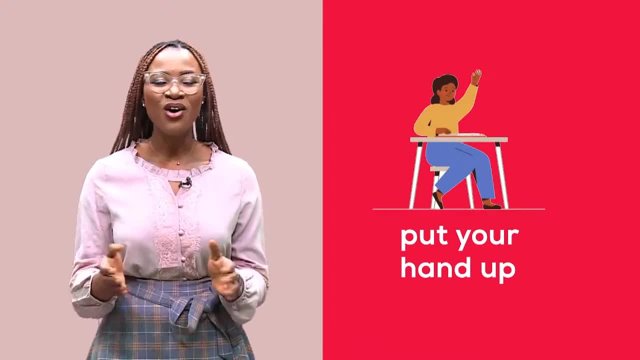 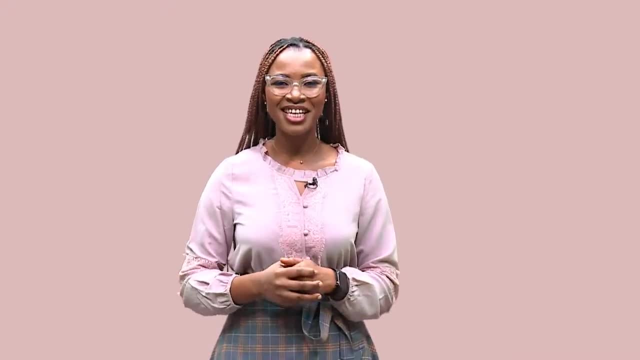 and ask the invigilator who is supervising the exams. More often than not, they will help you or point to you in the right direction. Six: look at the marking scheme. Keep an eye out for the marking scheme that shows how many marks are being awarded for each exam. If you are stuck on the 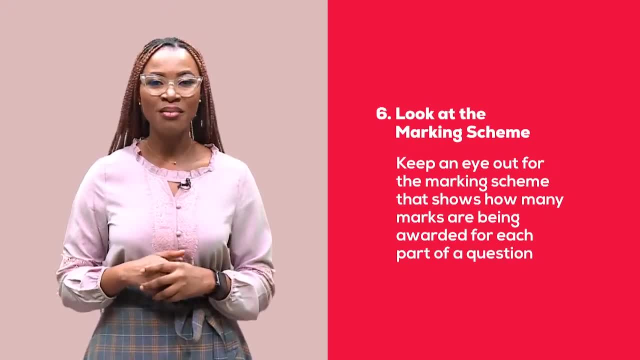 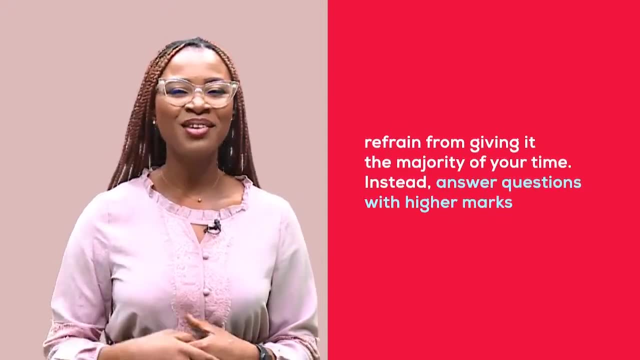 marking scheme. look at the marking scheme. that shows how many marks are being awarded for each exam. If there are only small amounts of marks going for a part of a question, refrain from giving it the majority of your time. Instead, answer questions with higher marks. Seven cross-check answers: 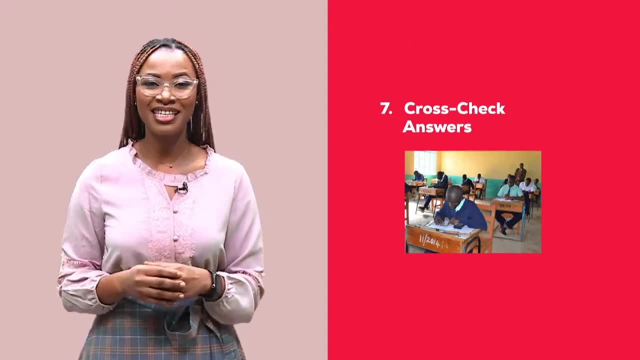 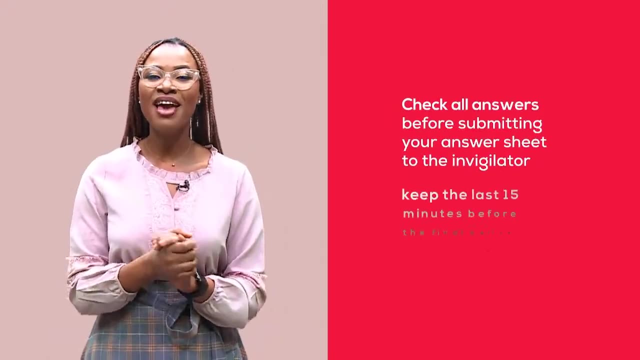 You must check all answers before submitting your answer sheet to the invigilator. You should keep the last 15 minutes before the final bell to cross-check your answers. A thorough revision of every answer is necessary, as it will help you to identify the answer sheet If you have. 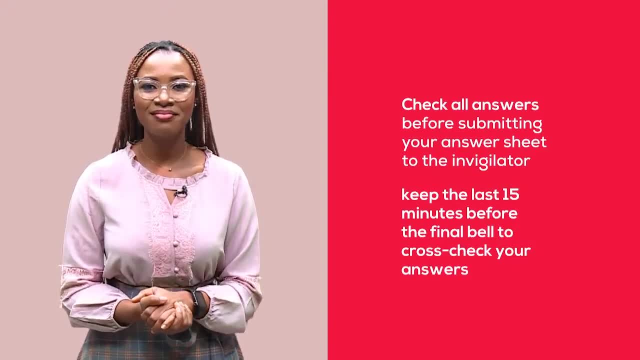 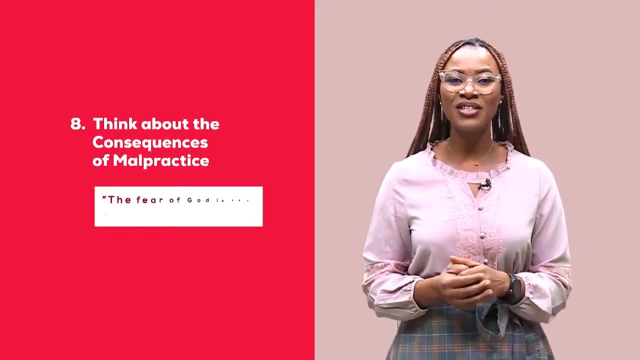 missed it. you can click to the next section to see what you have to say. Eight, think about the consequences of malpractice. Ever heard the saying: the fear of God is the beginning of wisdom? Always remember there is punishment for people who are caught cheating. 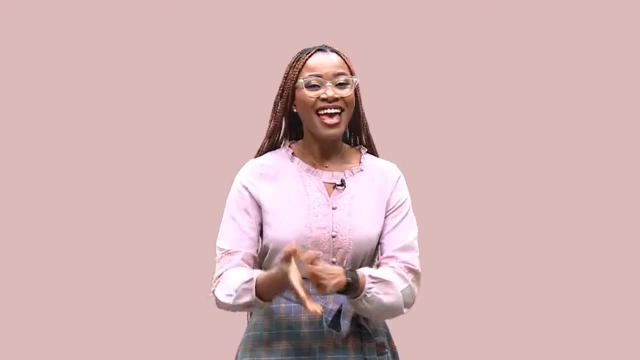 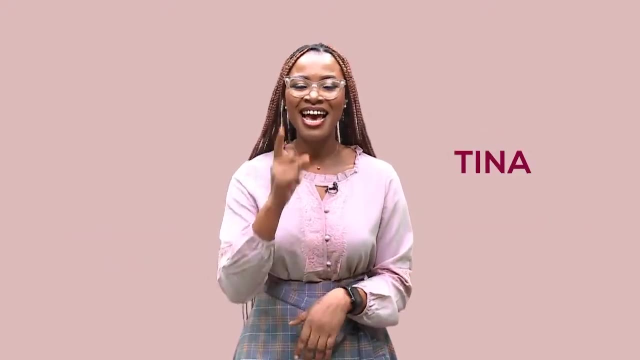 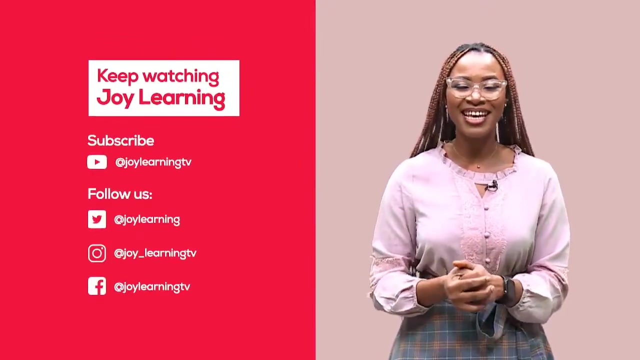 There you have it. Believe in yourself, prepare well and you will come out with flying colors. My name is Tina and I am your Examination Coach. Keep watching Joy Learning and follow us on platforms so they come your way again. sign on joy learning, keep learning. 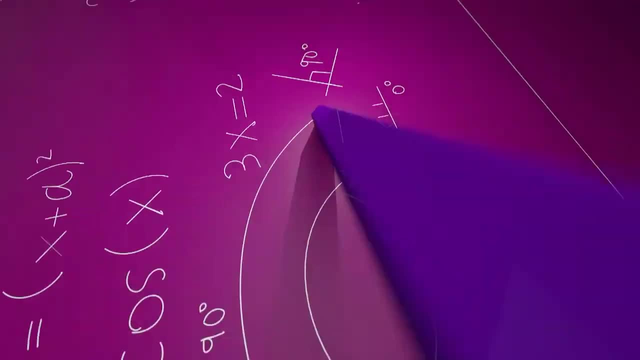 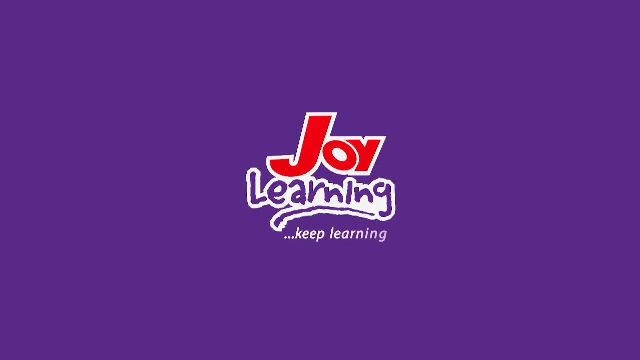 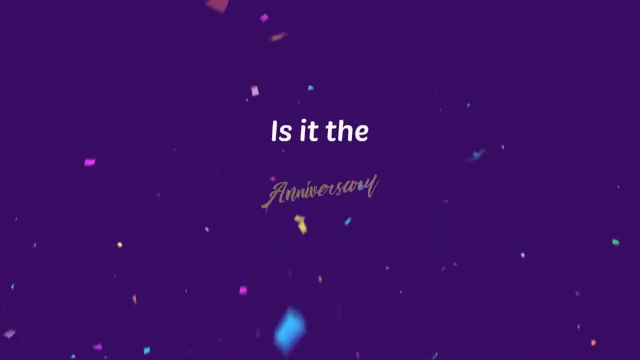 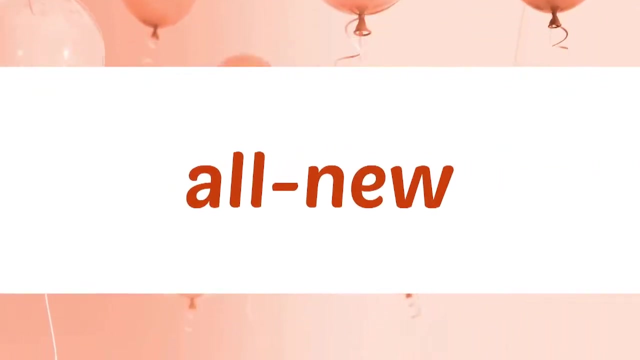 it's time to wish your loved ones well on that special occasion. is it the birthday or anniversary of your child, friend, classmate, your schoolmate, your teacher or non-teaching staff of your school? the all-new jl birthday wish by gunner's, number one educational tv channel, hits your regular. 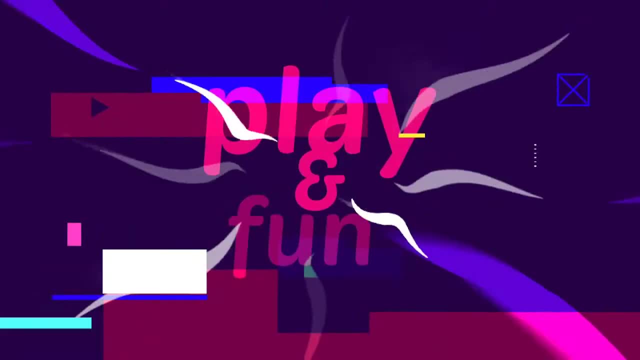 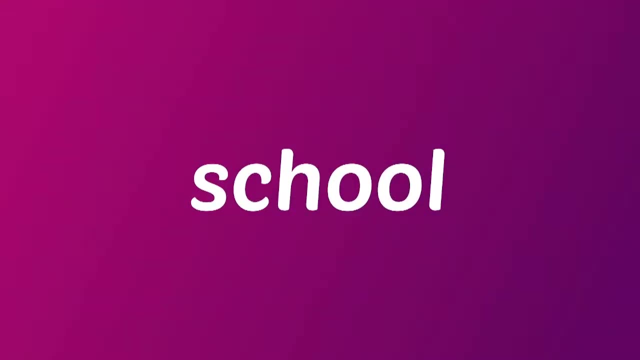 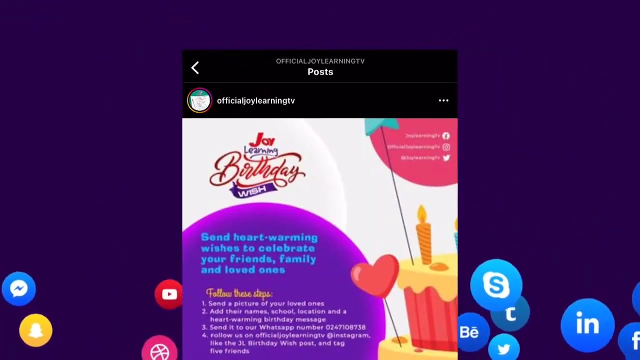 classroom screen and, as usual, it is time for jack to play and have fun. it has been made easy for you and this is how: send a picture of your loved ones, add their names, school and location and a heartwarming birthday message. and finally, follow us on official joy learning tv on instagram. 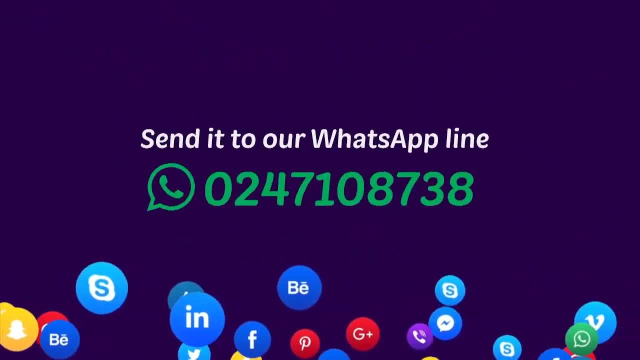 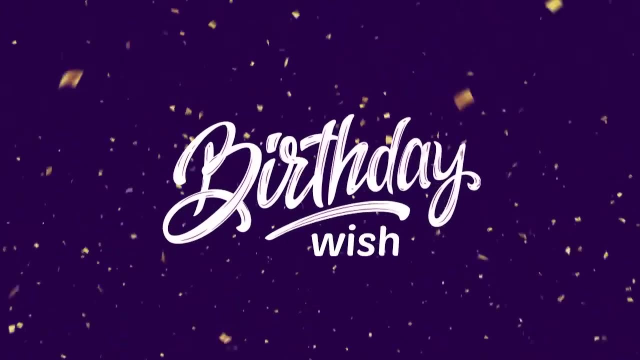 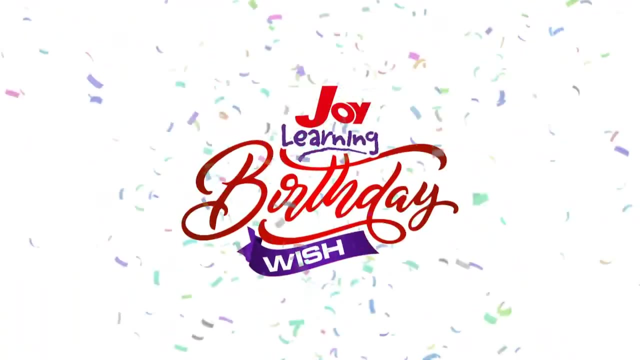 like the jl birthday wish post and tag five friends, send it to our whatsapp line 0247108738 and voila, your birthday wish will be aired on joy learning tv and all our social media platforms. learning is made fun with the jl birthday wish. joy learning, keep learning. 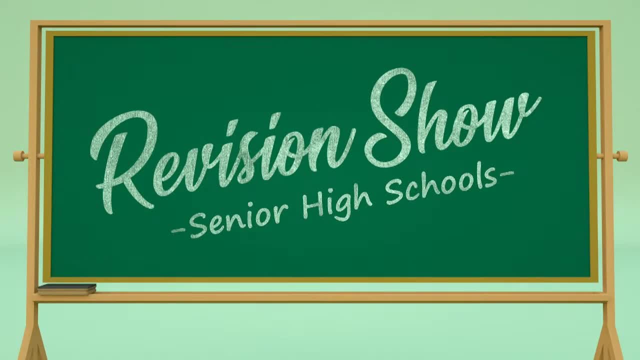 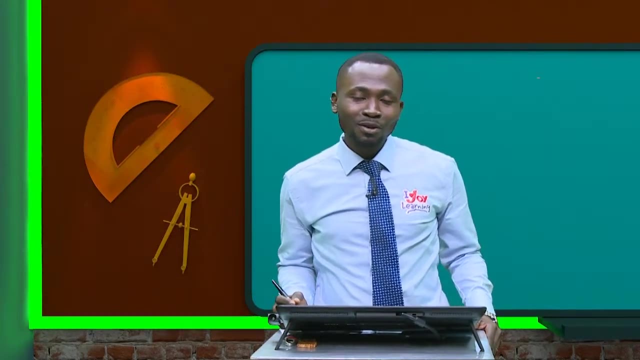 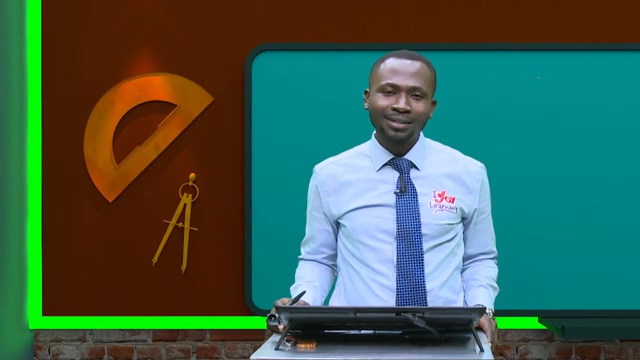 all right, welcome back. it's revision show time and you can call me pious, i'll be here with you taking you through something little on the law of radioactive decay, decay, constant, how do you do it? okay, so let's begin with the answer. and how about some life and decay, probability, activity and all? 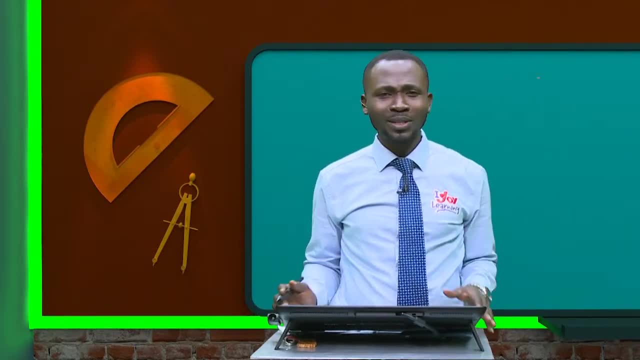 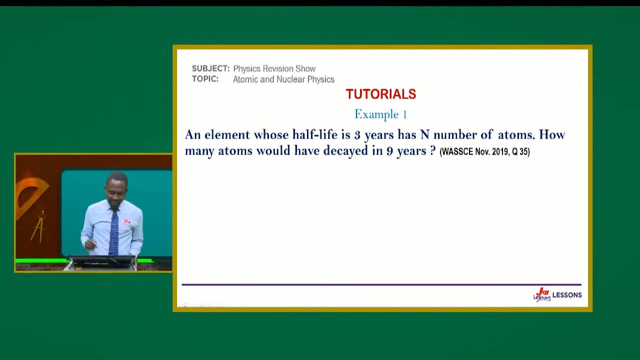 that it's a good time for us to try and answer two questions. and then i want to remind you that in some few minutes time i'm going to open a phone line so that you can call him, okay. so example one: an element whose half life is three years has n number of atoms. 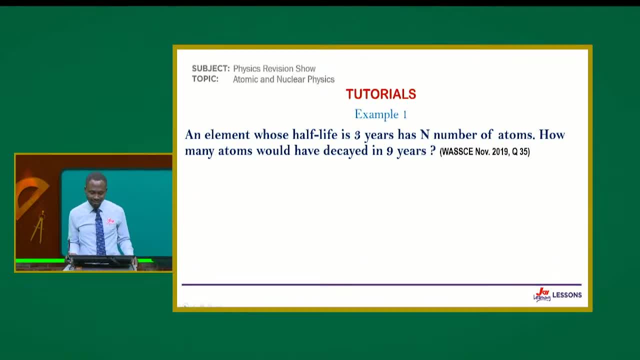 would have decayed in nine years. this is rossi, november 2019, question number 35. now we're giving possible answers: a- seven on eight n atoms, b- one on eight n atoms, c- one on three n atoms and d- two on three n atoms. so we have to try and solve this question. 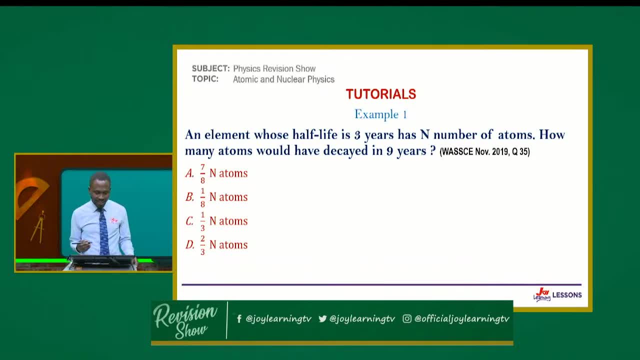 we can solve the question by looking at or by putting down the parameters in the question. we have been given half life, three years, so t half is three now the number of atoms present now is n. we were using n naught, so i'll say n naught equals n. 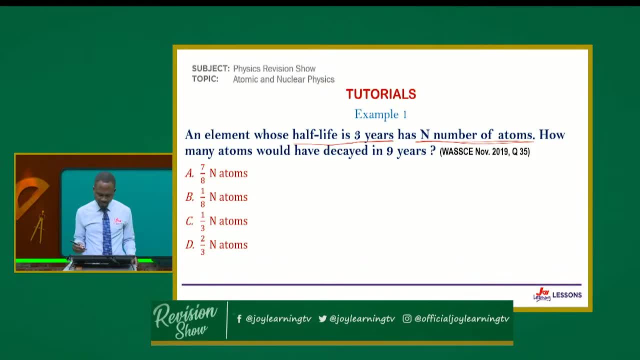 but don't worry with time, we'll replace it. okay, then i asked how many atoms will decay in nine years. so the time you are still is nine years. if you want to know the number of atoms that would have decayed, okay, in nine years, well then, we have to look at. 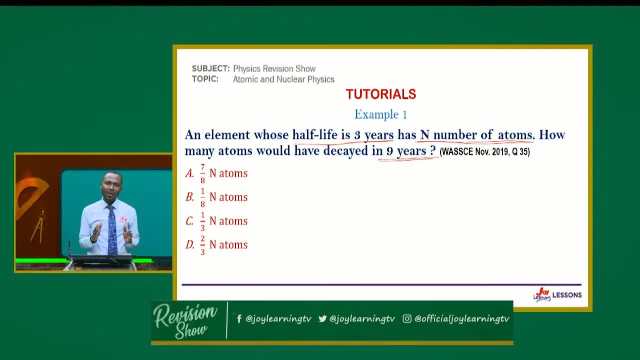 what we have initially, what we have left. then when we subtract, we'll know the amount that would have decayed. so in nine years time, what would be the amount of, or would be the number of atoms left? now that we have n number of atoms in nine years time, how many would decay in nine years? 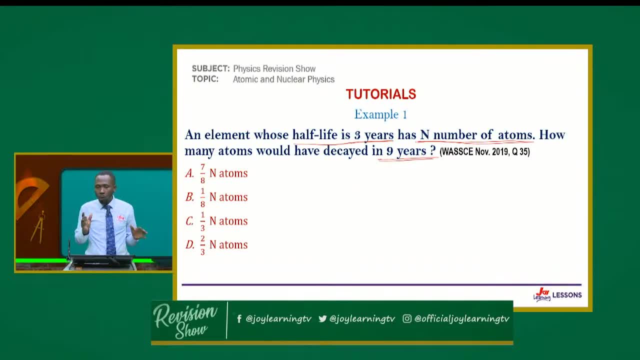 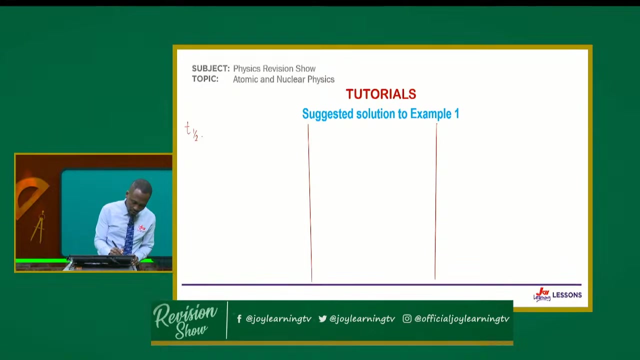 time, how many will be left when we sub? we had that and we subtract, we're going to get the amount or the number of atoms that would have decayed in nine years. so let's set the ball rolling. so let's put our parameters. we have half life, t, half to be three years. 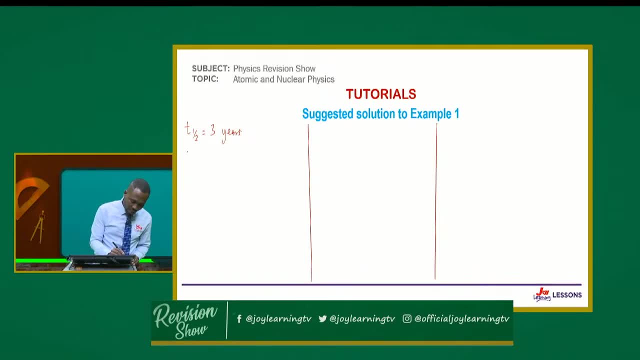 we have the number of atoms now. so i'll say n naught is n atoms. then we have the time to be nine years. good. so number of atoms that would have decayed is equal to the number of atoms present initially, Minus the number of atoms left after the decay. 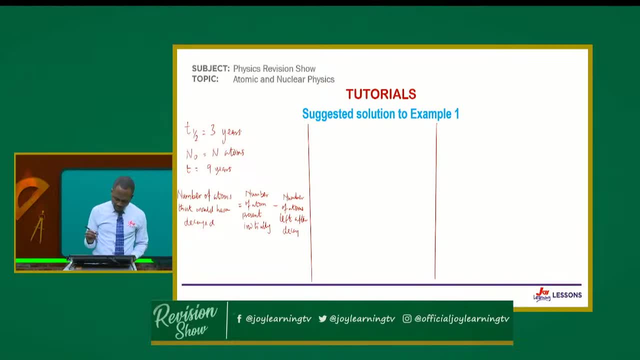 So let's move on. We have a formulating edge, that n. what is left? You see, we know the number of atoms initially present to be n, naught, and now I think it's n, So we know this one. 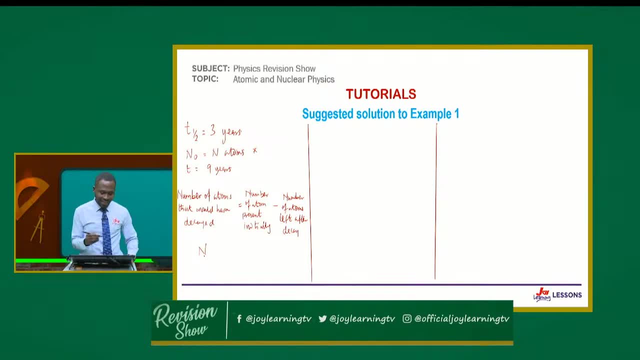 Now I'm supposed to go and look for n, the number that will be left after the decay. Then we can subtract, So n equals n naught over 2 to the power n right. So let's move on. 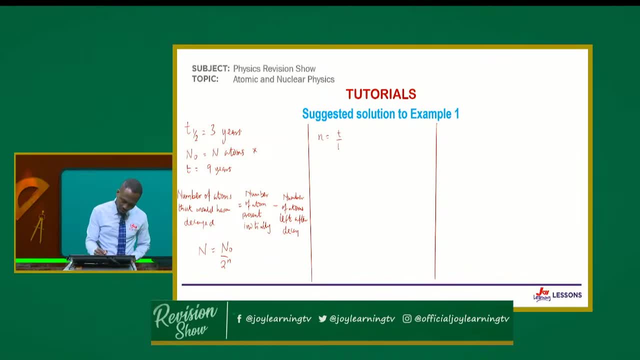 What's our n? Our n is t on half-life, right. So when you get t, which is our 9, on our half-life, which is our 3,, that gives us 3.. So that's the case. 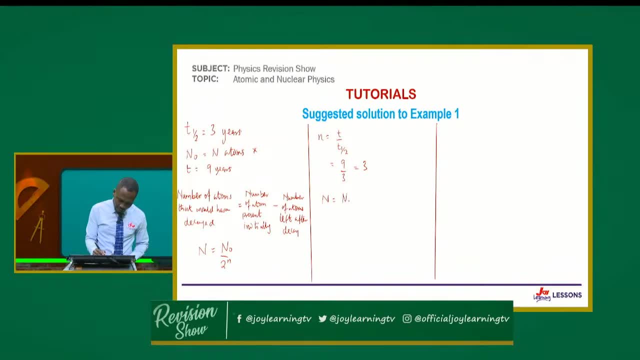 I'm going to get n giving me n naught on 2, 3.. Giving me n equals n naught over 8.. But don't forget that our n naught is the n atoms right, What is left. It will be the initial one over 8.. 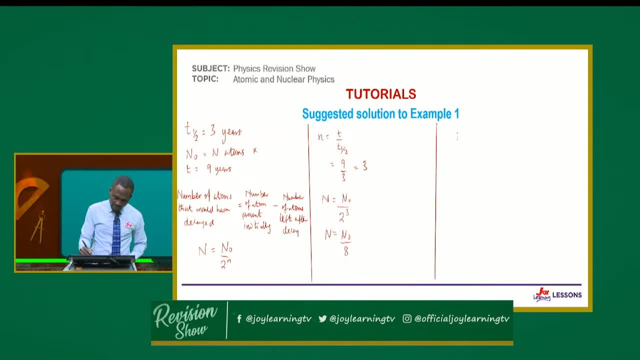 But according to the question, n naught is the n. So instead of n naught over 8, you're going to get n over 8.. So I'm going to get From the formula number of atoms present initially, which is n minus what I have. 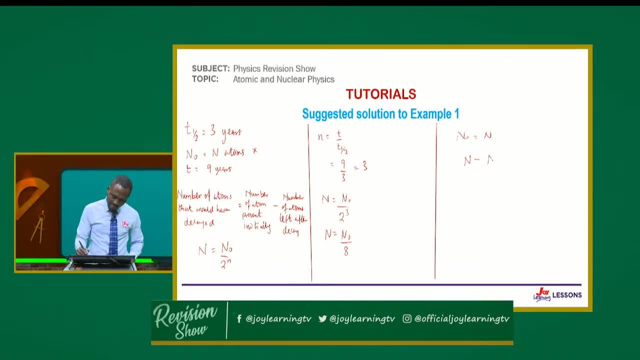 n number of atoms left after decay. So I'm going to get n on 8.. So this is 8 times 1.. The equivalent of n here is 1.. So 8 times 1, 8, minus 1 here. 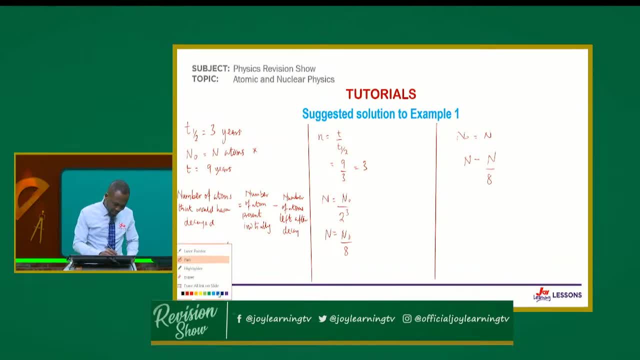 So just to make you understand, the equivalent of n here is 1.. N naught under n here is 1.. So 8 times 1 here is 8, minus 1 is 7,, all over 8.. 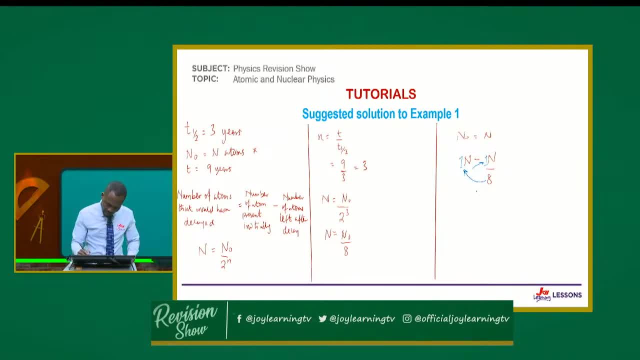 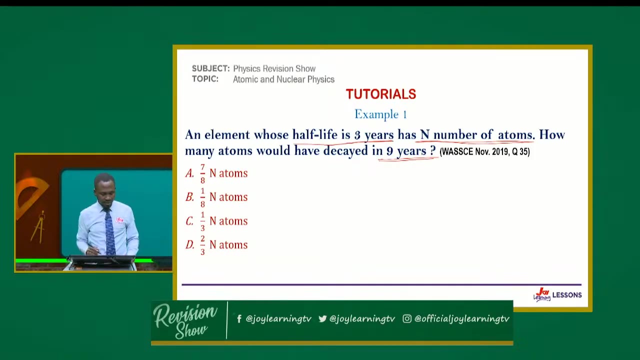 So here our answer becomes 7 over 8 n, 7 over 8 n. Let's see if we have this in the possible answers. So 7 over 8 n. atoms is here, And that becomes our answer. 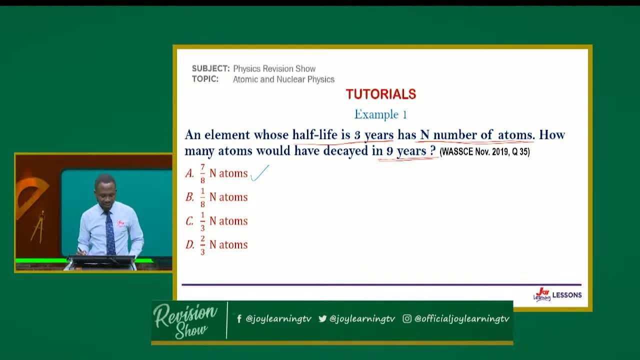 So in 9 years' time you're going to get 7 over 8 n atoms That would have decayed- 7 over 8 n atoms that would have decayed Good, I think we can get another example. 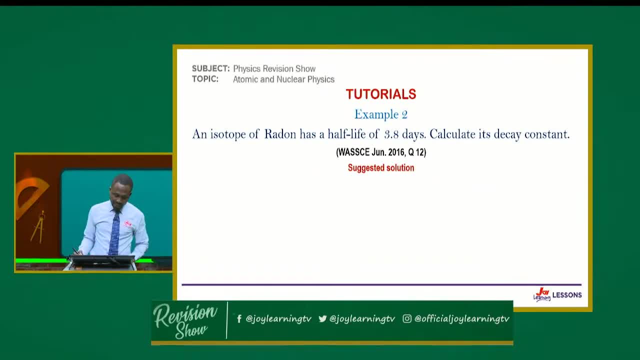 It says: an isotope of radon has a half-life of 3.8 days. Calculate its decay constant. An isotope of radon has a half-life of 3.8 days. Calculate its decay constant. It's also a fast question. 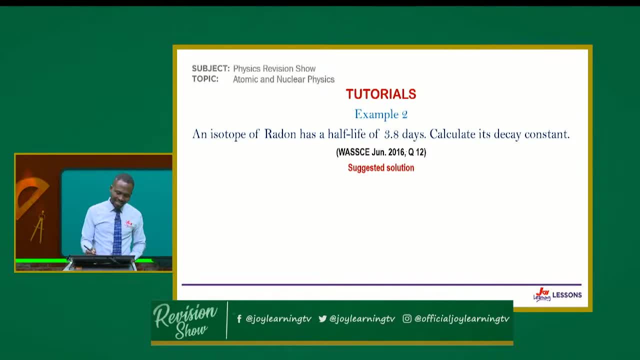 Wasee for school candidates 2016,. question number 12.. So, as far as question number 12, we had this question. So, like I mostly do, we start by putting down our parameters For this question. we have half-life. 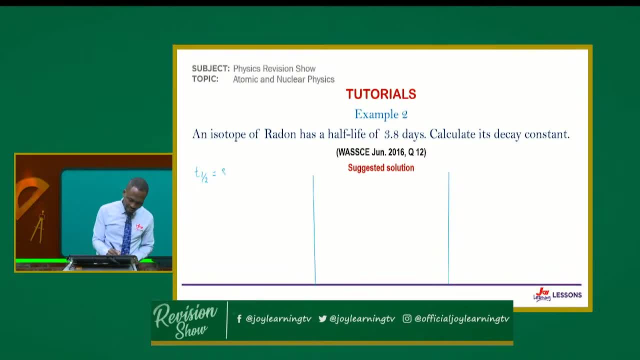 So t-half is 3.8 days. Yeah, I have to find decay constant, which is lambda. What's our formula? Our formula says half-life is equal to natural log of 2 on decay constant. So I'm going to get. 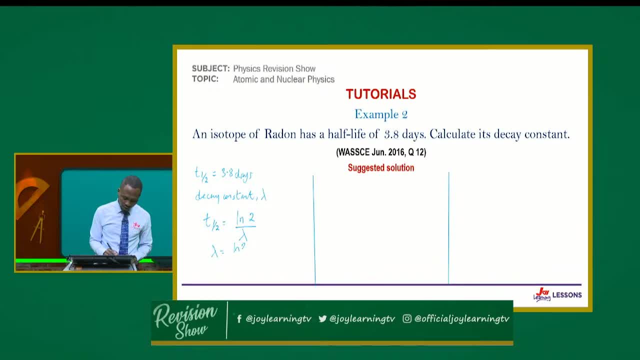 The decay constant to be natural log of 2 on half-life. So decay constant, give me natural log of 2 on 3.8.. To give me: With the calculator you can easily get that Over 3.8.. 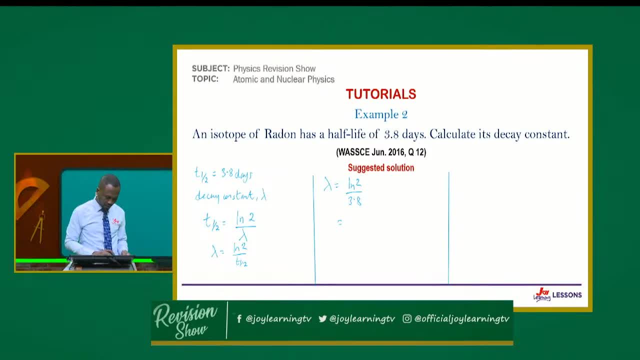 And that's going to give you an answer: 0.182.. So 0.182 C per day, Per day, Per day. But when we looked at the units of decay constant, what's per second? So we could also have solved this question. 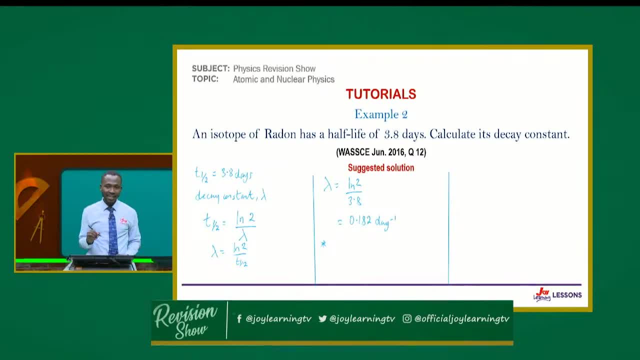 Leaving an answer Or an answer in per second. I actually chose this question to make you understand that Why can go as low as giving you very simple questions like this Just to test your understanding. So in that case I would have to change my half-life t-half. 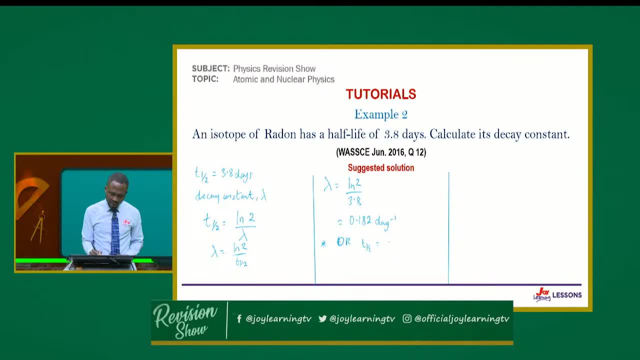 Which is 3.8 days to seconds. So I'm going to get my half-life to become 3.8 days times 24 hours in a day, times 60 minutes in 1 hour, times 60 seconds, making 1 minute. 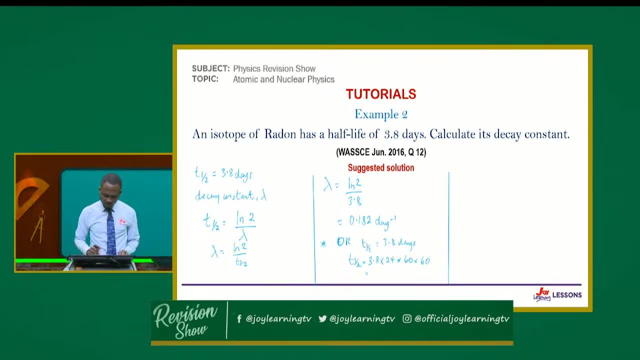 So 3.8 times 24 times 3,600 times 60 times 60.. So that gives me 3-2-8.. 30 seconds, So 3.8 days times 24 hours times 60 minutes times 60 seconds. 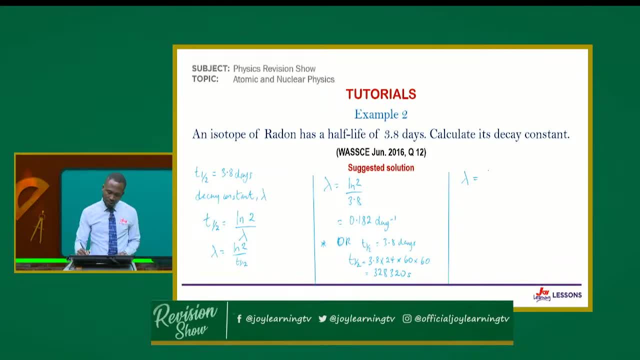 So in a second. So in that case lambda will give me log of two on three, two, eight, three, two, zero seconds. so when you guys that divided by that and I'm getting two point one, one times ten exponents minus six per second, per second. 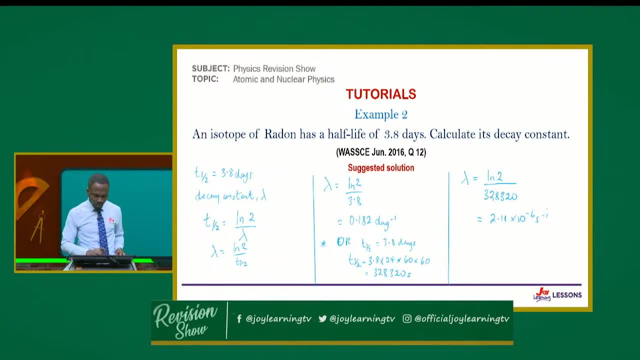 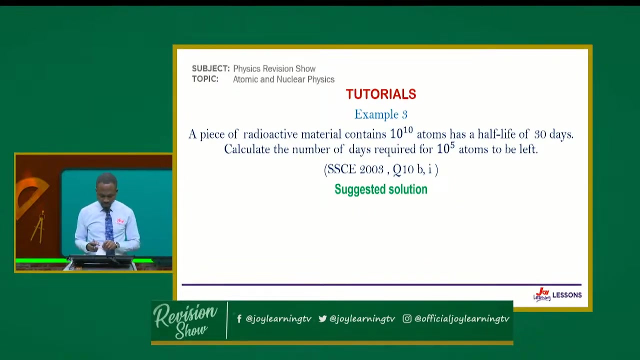 so you can also change the half-life from the this two seconds, like I've done here, and then you follows you with the procedure, follows it with a procedure. alright, we can move on. that's another example. it says a piece of radioactive material. Now, a piece of radioactive material contains 10 to the power 10 atoms, 10 to the power 10 atoms, and has a half-life of 30 days. 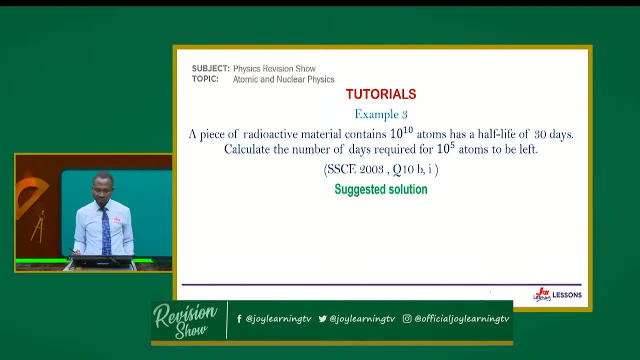 Calculate the number of days required for 10 to the power 5 atoms to be left. So we have a radioactive material that has got 10 to the power 10 atoms. So that becomes our N? naught. So initially you have 10 to the power 10 atoms. 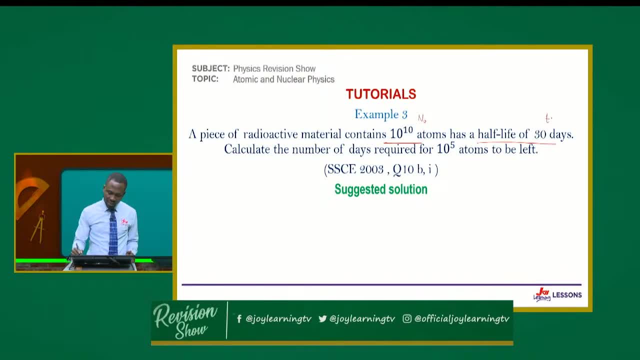 Then the half-life to T, half 30 days. We are asked to calculate the number of days. So what we don't know is the time, The number of days required for 10 to the power 5 atoms to be left to admit that our N becomes 10 to the power 5.. 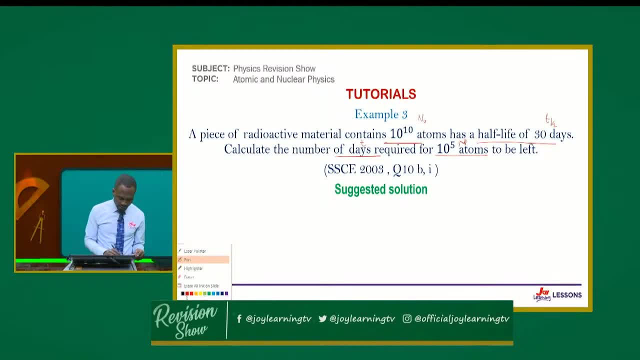 So let us try and put down our parameters and see what we can do about this. So I have N naught to be 10 to the power 10.. So we have N naught to be 10 to the power 10 atoms. 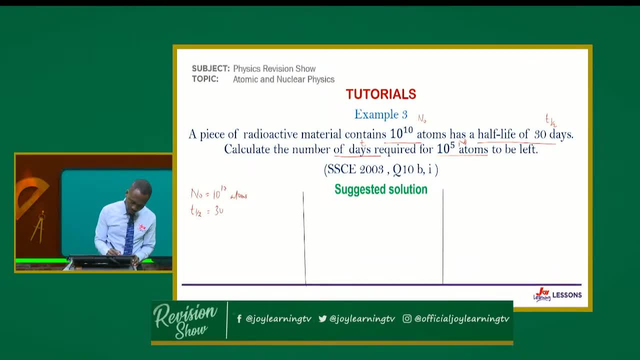 I have half-life to be 30 days, We have N of atoms remaining 10 to the power 5 atoms, And we are asked to find a time T. So we will go with our decay equation, which is n because and not e, minus lambda T, but I can just pick it. 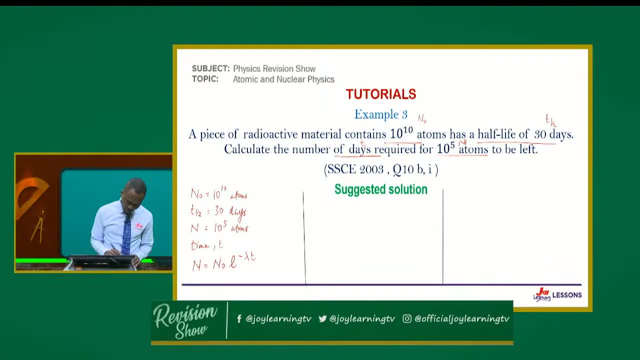 like this. I'll work this out separately, so T this way. so let's put things into perspective. we want to find T, we know n, we know n not, but the information we have here, we can find T so that we can come back and put it in there. we could. 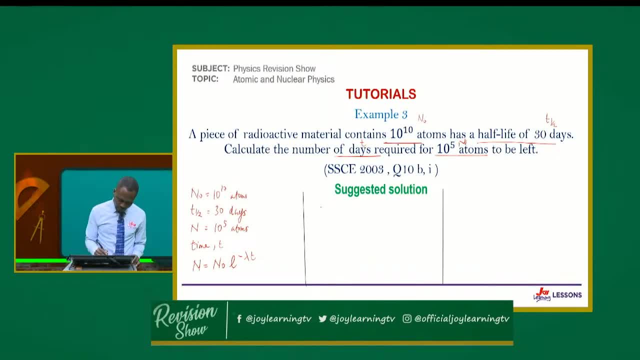 let's find lambda. so I'm gonna get T half because that on that. so our aim of this is right. C, but we can find lambda. after we give it to us, then we come and put it into the equation, manipulate it to find T so lambda. just give us natural log of 2 on the half-life and lambda. 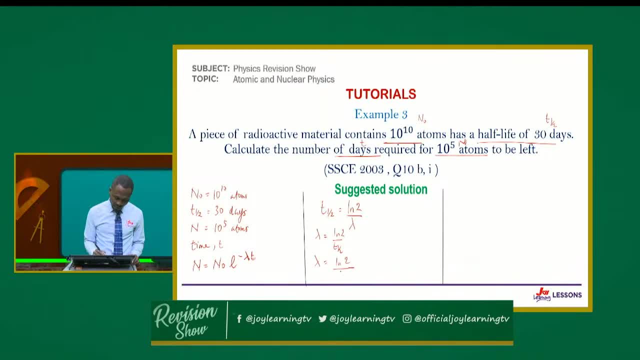 give us a log of 2, so I have life 30. so let's use the calculators, get natural log of 2 all over 30 and that's going to give you zero point, zero, two, three, one. okay, so we can move on. so in place of n, I have 10 to the power 5. I'm gonna get 10 to the. 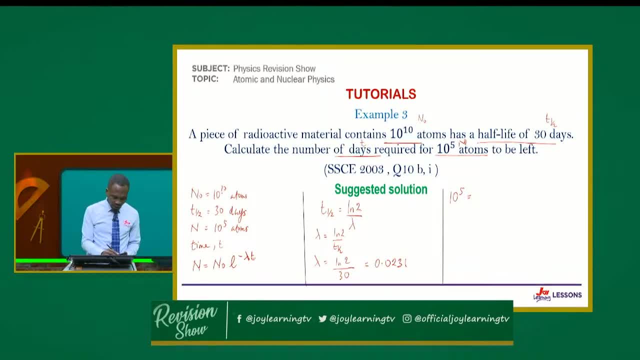 power 5 atoms equals, and n not to the power 10, 10 to the power 10 exponent. are we good to go? minus? then lambda is 0.0231, then T, which you don't know. so now the rest is our marks. you have to find ways. that means to get. 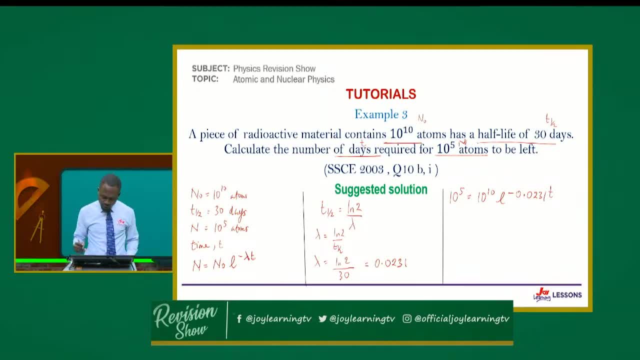 what we want. okay, so I divide both sides by two to the power five, I'll get 1, 2. I'm dividing both sides by 10 to the power 5, probably. let me just show it. so this 1 and 2 is not that big, it's justоровice, and 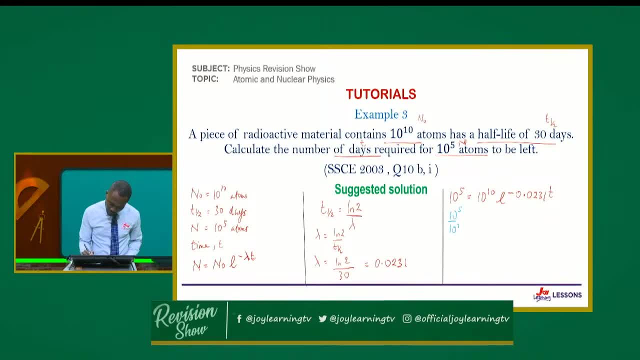 3 is n and 3 is not the berries. and old 7 x 2 times one is not that big. so this t x 2 y is b. so if we did get 10 to the power 5 on 10 to the power 5 equals 10 to the power 10 e minus 0.0231 t on 10 to the power 5.. 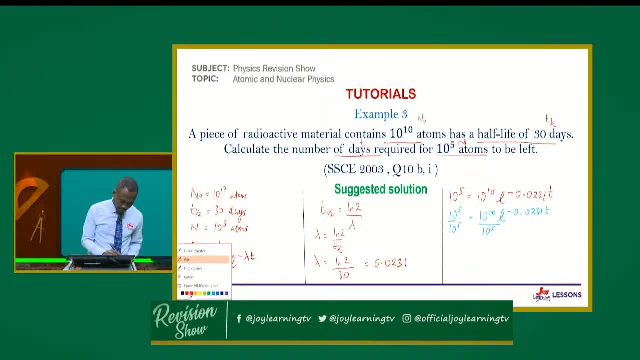 So ideally I could just skip this step and move on. So this will give me 1, because it will cancel out, I'll get 1.. Okay Then, from indices 10 to the power 5 numerator. if this 10 to the power 5 should go up, it becomes 10 to the power minus 5.. 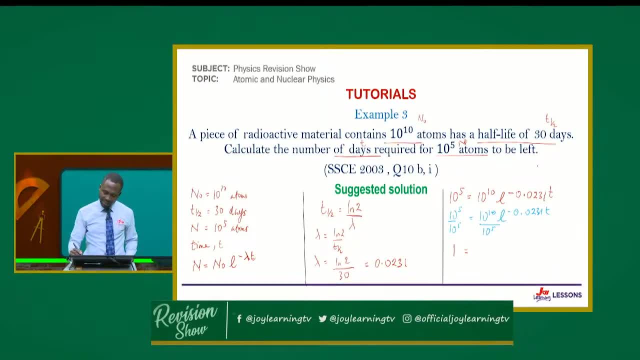 So you get 10 to the power, 10 times 10 to the power minus 5.. Something like this: 10 to the power, 10 times 10 to the power minus 5.. You give me 10 to the power, 10 minus 5.. 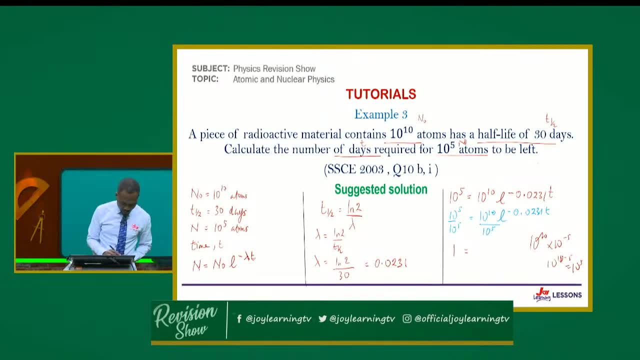 10 to the power 5.. So that should be okay with us. So I'm going to write 10 to the power 5 in place of 5. All that, So I'm going to get 10 to the power 5.. 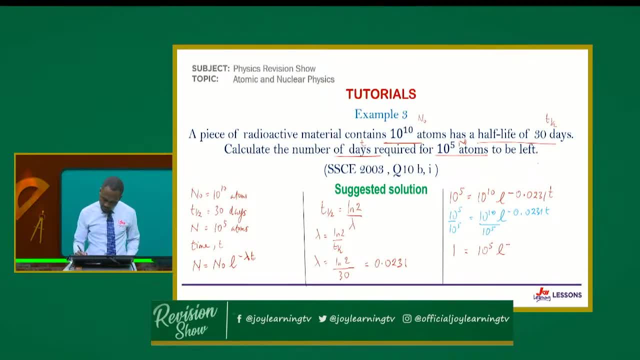 Write Exponent: negative: 0.0231 t. Let's keep working. What can I do? We can have 1 over 10 to the power 5.. Okay, 1 equals all that. We are trying to take away this negative sign. 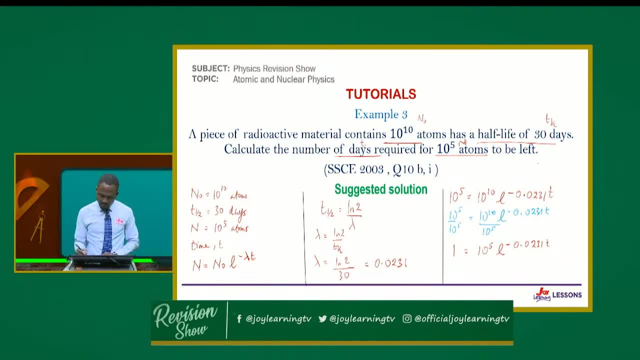 So, like I did, If I divide both sides by 10 to the power 5, I will still get 1 over 10 to the power 5.. Oh, It's equal to e minus 0.0231 t. Let's move on. 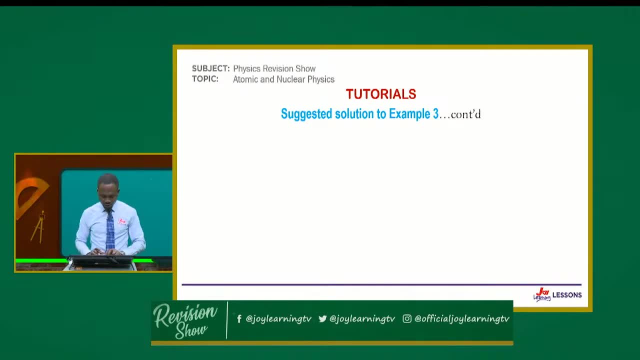 That will give me. I'll just repeat my last step so that you can follow through. So I have 1 over 10 to the power minus 5 equals e minus 0.0231 t. So 10 to the power 5.. 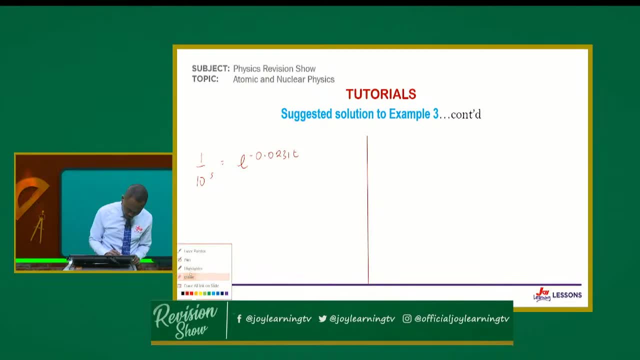 Sorry, Sorry. Good, This will give me 1 over 10 to the power 5. So It's equal to 1 over e minus 0.0231 t, So that the negative goes away. Then I can find the reciprocal on both sides. 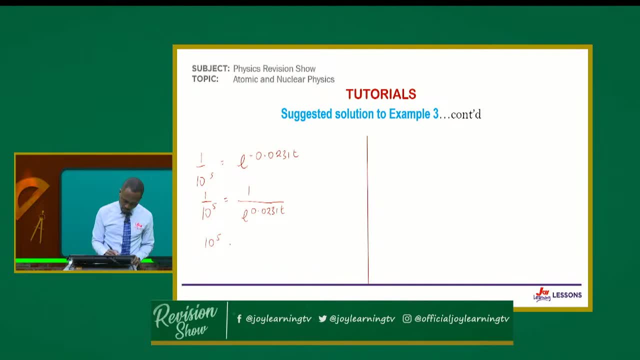 So you get 10 to the power 5.. Write It's equal to 1 over T E 0.0231 T. right, Alright. So when it gets, If Log Off 10 x 5 to base. 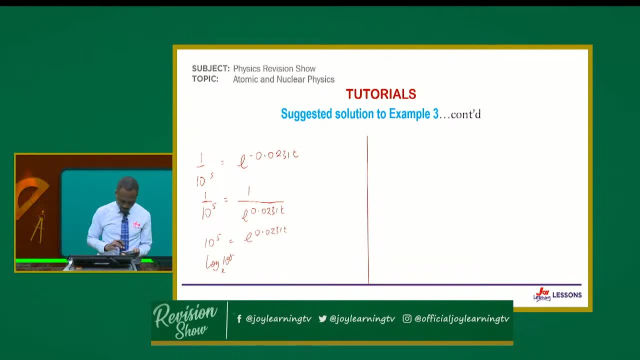 E. Right, It's equal to natural log of E. So I'm going to get 0.0231T to base E. So I'm going to get that of 10x25 equals. now I'm going to get log of E to base E. 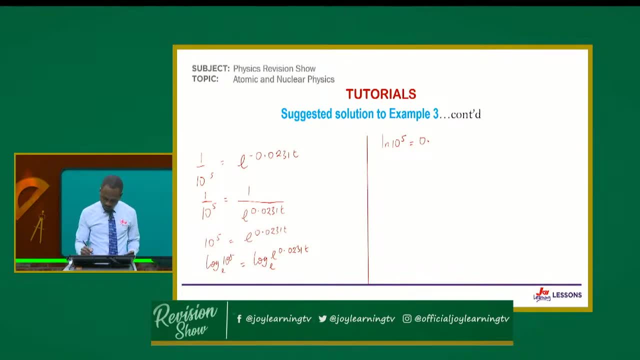 So 0.0231T, That's log, That's log E to base E. This will give me 1.. That whole expression of log E to base E will give me 1., Equal to 1.. So I want to keep natural log of that. 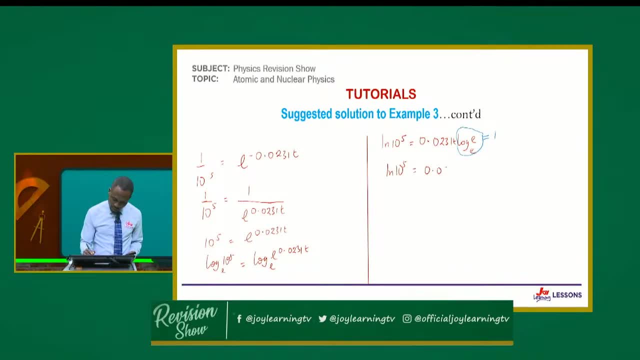 So that of 10x25 will give me 0.0231T. So T will give me the natural log of 10x25 on 0.0231T. So let's try to see if we get an answer. 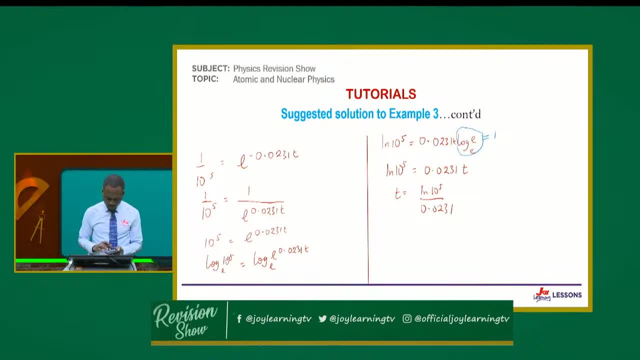 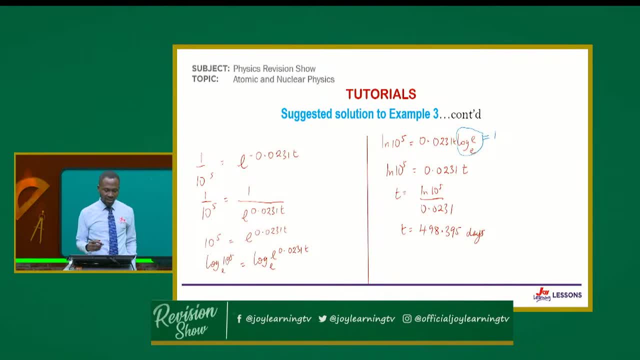 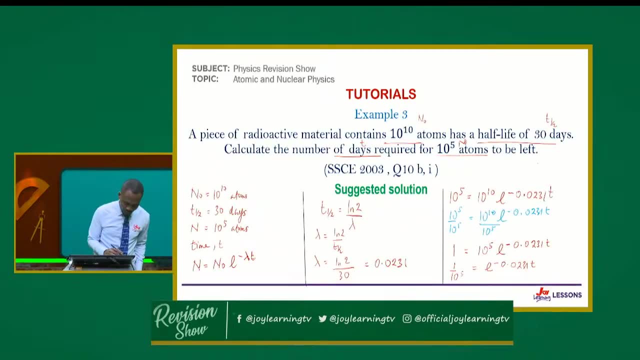 Wow, I'm going to get. T is equal to 498.395.. So it's important to take your time and go through the steps. So, right from the onset, from our parameters, we put our decay equation there. Then we find lambda from this expression. 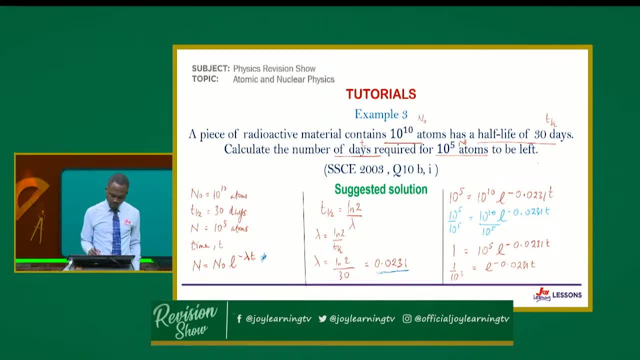 Then we find lambda from this expression, Then we find lambda from this expression to get the lambda to give us 0.0231. then we move on, put it back into the equation. this is 10 to the power 5, 10 to the power 10 e minus lambda times T. 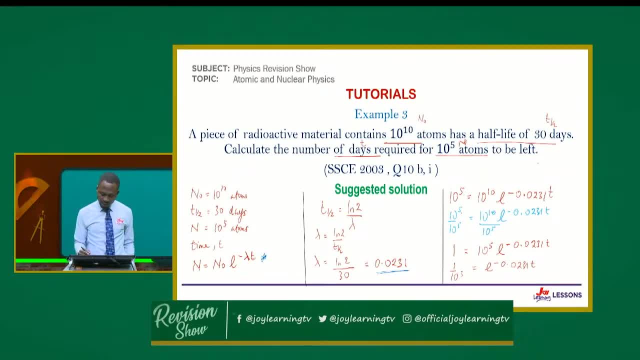 variable sides by 10 to power 5. so we take this away. I got one, then you can power 5, e that so, but again by 10 to the power 5. I want this to stand alone, to get this, then to take away the minus. I bring this whole thing as a denominator, so I 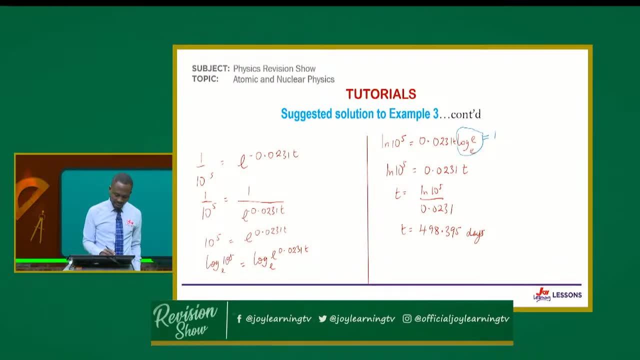 have 1 on that, 2 negative goes away, 1 on that. then we can reciprocate to get this expression. you find natural log to be a log to base e for both sides and this log based log, e to base e, becomes 1 and this one I maintain it as natural log of 10 to the power 5 giving. 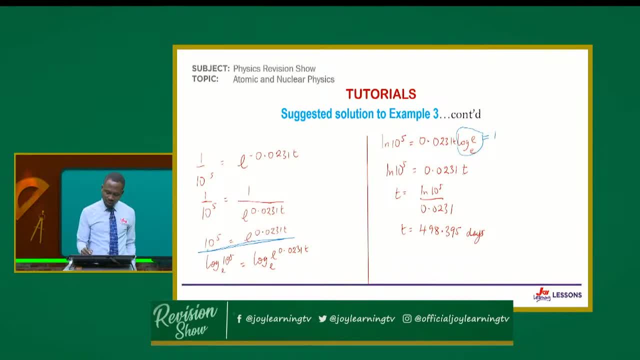 me this. then I divide this by what's attached to T, its coefficient, and that gives us 498.395. this, it's a good time to open the four lines so that you can try hands on the. you can try hands on the problem of the day. you have seen the questions already. you can call in zero. 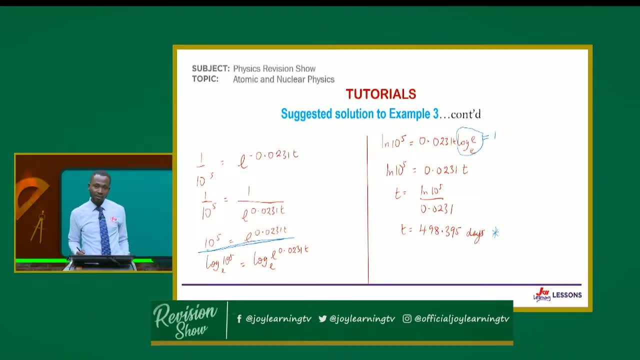 three zero two two one one seven zero five. the numbers will be shown on your screen. zero three zero two, two one one seven zero five. or zero three zero two, two one one seven zero six. zero three zero two two one one seven zero five. or zero three zero two two one one seven zero six. kindly tune your volume of a TV. 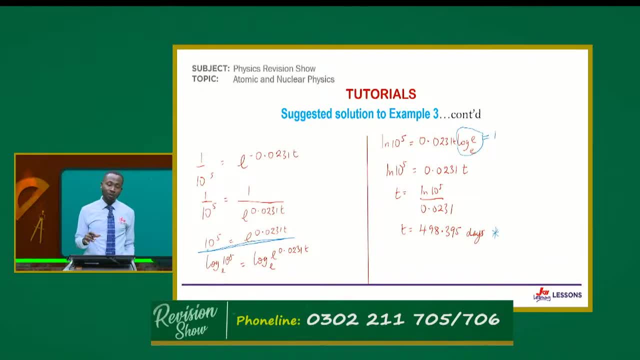 set when you call in so we can communicate via call handset, mobile phone, whatever we're using to call working, and then try and give answers to the problem of the day. very, very simple questions. so 0, 3, 0, 2, 2, 1, 1, 705 or 0 3 0, 2 to act out 4A. you see that you have a very simple exercise from. 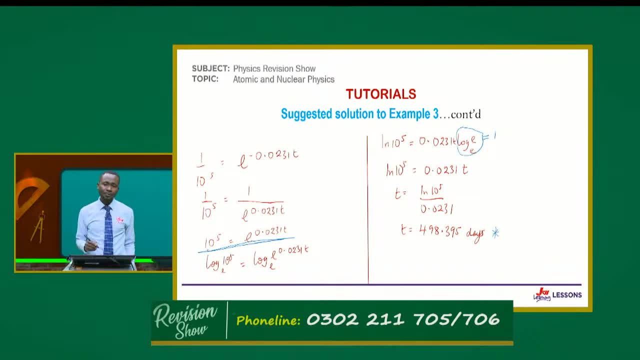 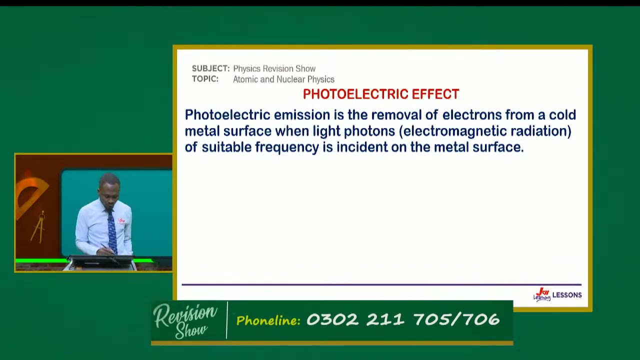 two, two, one, one, seven zero six. so in the meantime i'll try and do a recap on photologic effects. i'm trying to take you through that and when you're asking, when your call comes in, i'll stop and then attend to you so we can look at photoelectric effect. 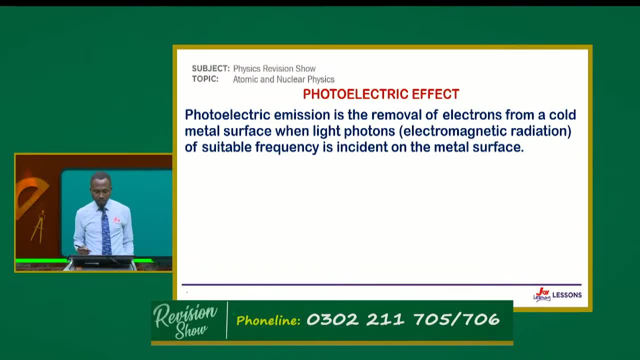 and that text will call it photoelectricity. so what is it? what is it? it is the emission or the remover of electrons from a cold metal surface. from a cold metal surface, when light photons or when electromagnetic radiations of suitable frequency is incident on the metal. 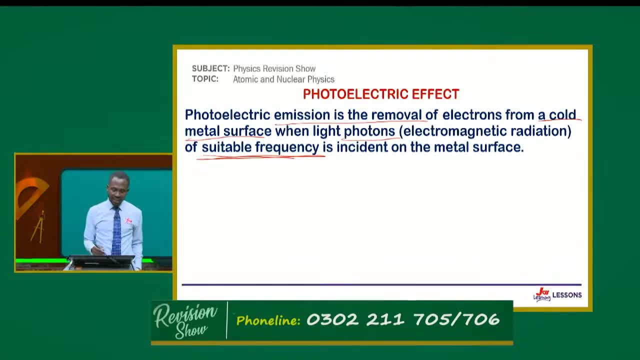 surface. so we are talking about having a metal surface, so this will be our metal surface. then with this there should be electrons on the metal surface. so when radiations are incident on the metal surface, these radiations contain tiny packets of energy, which you call photons- photons. so when the photons are incident on the metal surface, 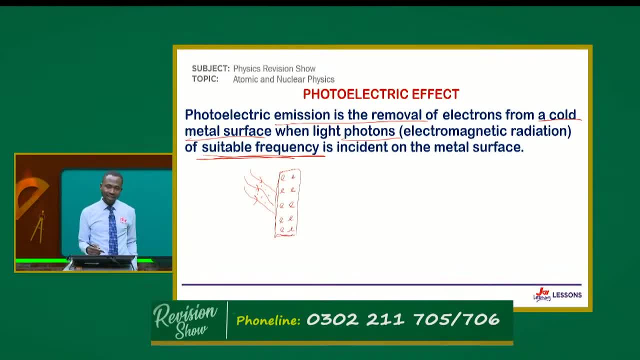 the electron absorbs all of the energy of the photon and then it's able to move out of the surface of the metal and this phenomenon is called photoelectric emission- photoelectric effect- i guess it's a color on the line. hello, you have anyone online, hello, hello, good evening. 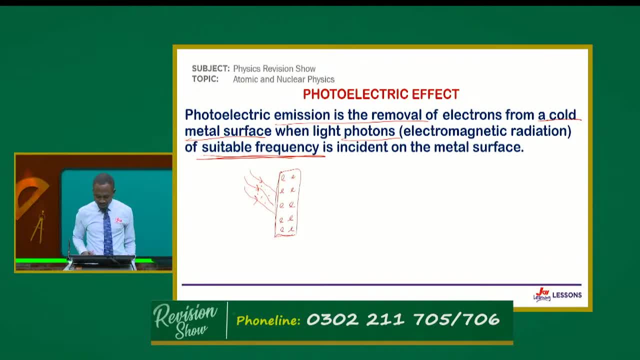 good evening, sir. your name please, and where are calling from. my name is: can you speak up a little bit? i'm trying to hear you. hello, yeah, can you speak up a little bit? yes, your name please. my name is okay. okay, please go ahead. you wanna answer the question? 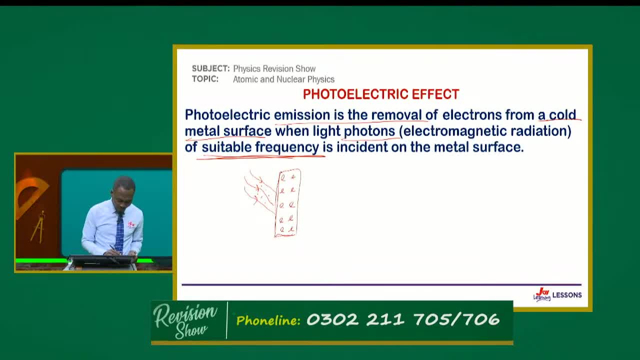 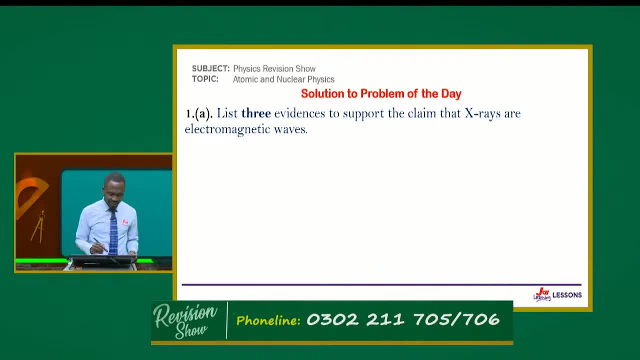 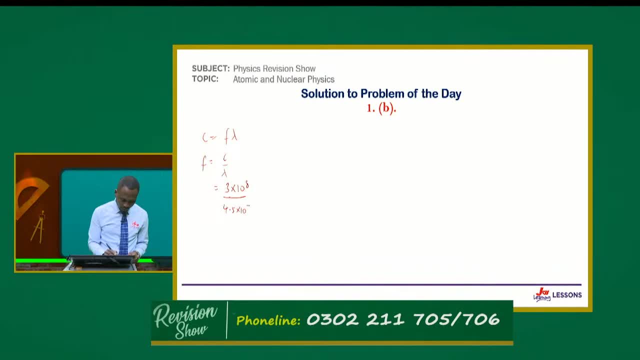 okay. and then we blend is given as four point five times 10gres, with 180. all right. all right, if okay. The equation is the energy of quantum radiation, which is equal to the Planck's constant times the frequency HF. okay, But the Planck's constant is given as 6.6 times 10, raised to the power negative 34.. 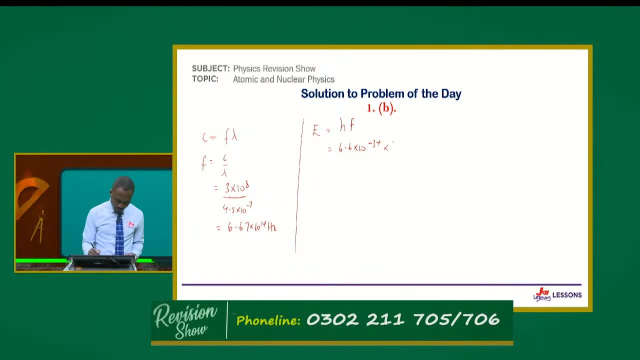 Okay Times the frequency, which is 6.67 times 10 raised to the power of 1000.. Okay, Therefore, the energy of the incidentalized will be equal to 4.40 times 10 raised to the power negative 19.. 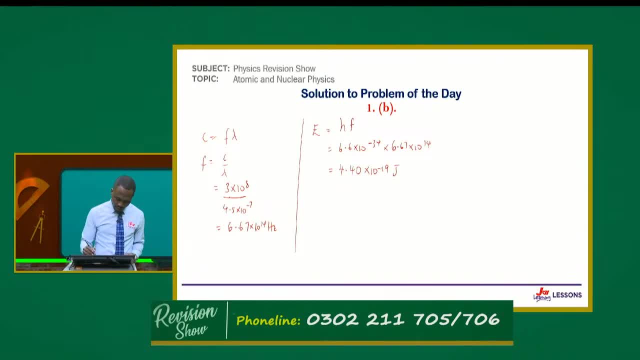 Good, Good Again. the energy of the photoelectrons emitted. What name will you give that energy? Huh, What name will you give that energy of the photoelectrons? Energy of the incidentalized. Okay, The energy of the incidentalized. 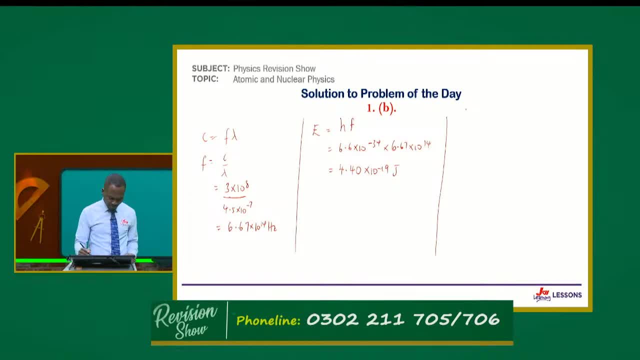 The energy of the incidentalized. What name will you give that energy of the photoelectrons? What will be the name? What's that energy? Energy of quantum radiation. Okay, That's the kinetic energy. Kinetic energy, All right. 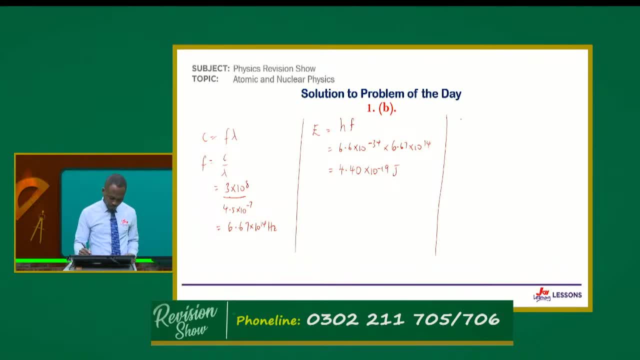 So please go ahead. Okay, From the Einstein equation of photoelectric effect. Good, Making the work function. subject: You want to rather make work function the subject. Sorry, The kinetic energy, the subject. Good, So kinetic energy will be the subject. 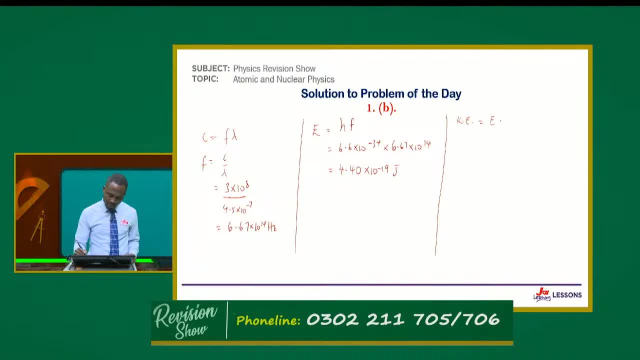 Yes, What kind ofobicic is the kinetic energy? Come, You can get the kinetic energy. Okay, What's that? So this is the kinetic energy, This is the energy So you can express every part. Okay, The connective energy. 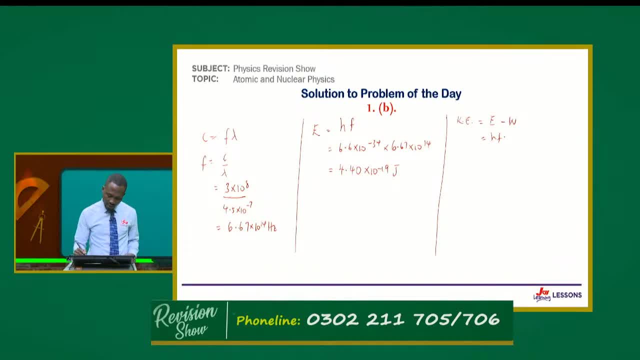 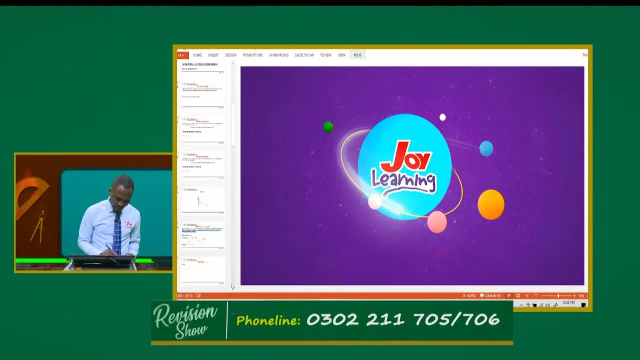 So you can start to change the to by 3.marciane. We got that OK, So that's negative 19 times minus the Imelda. all right, very good, very good, that's impressive. you have done justice to all the questions you've sought for frequency of the radiation you sought 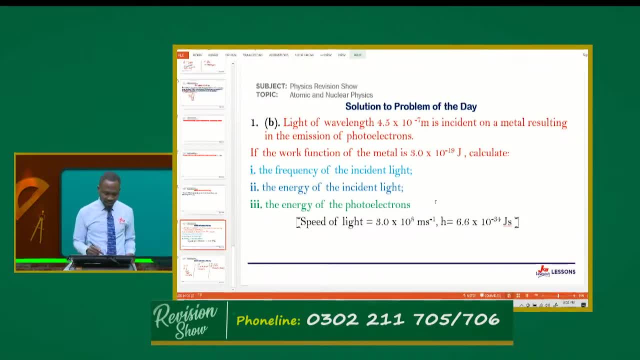 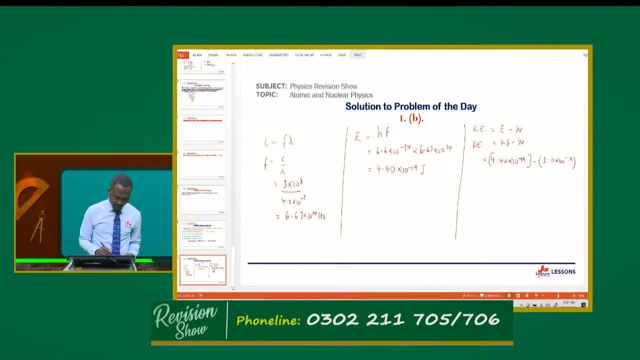 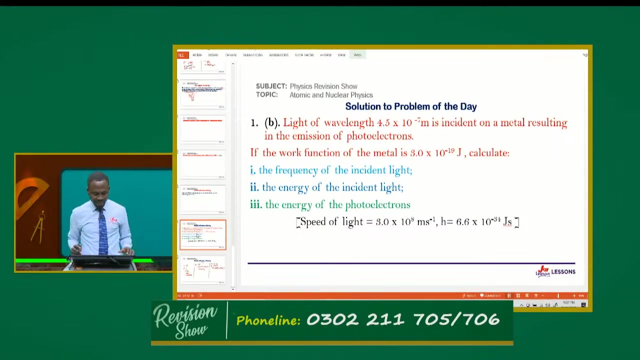 for the energy is the photon you've sought, for air, the photoelectrons. so my producer will talk to you right. all right, thank you for calling. we appreciate your call. thank you, all right, so does it. he called to answer question 1 B and he has been able to work it out. 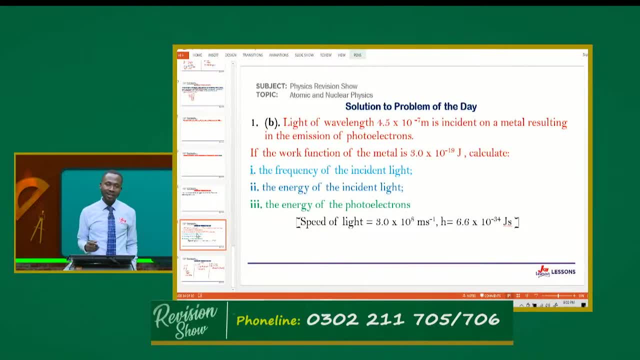 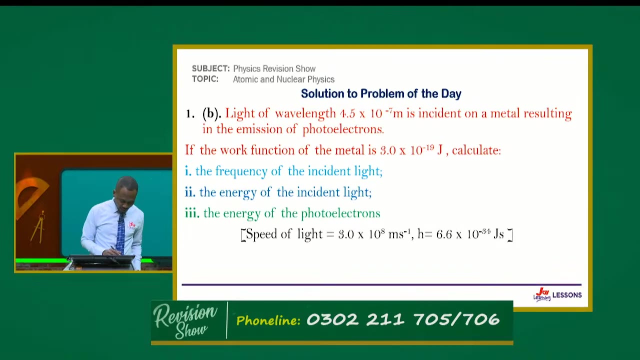 completely, everything correctly. Bravo, well done, well done. that's that's impressive, that's impressive. he's really really done so. so, so well. that's impressive, that's impressive. so he's done justice to that. he's giving us what the frequency of the radiation or light is here, the energy of the. 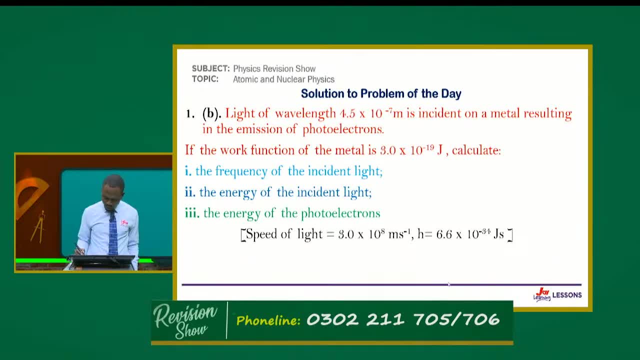 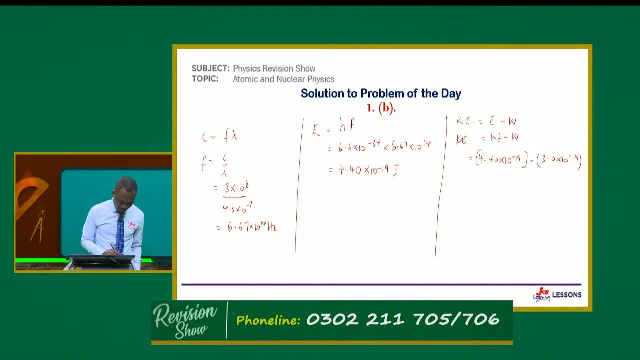 incident photon. he's done all that he's supposed to do. that is very, very, very good of you in for that is impressive. you've done well. Bravo, Bravo, Bravo, all right, all right. so direct the call on a lie. hello, all right. good evening, your name, please. 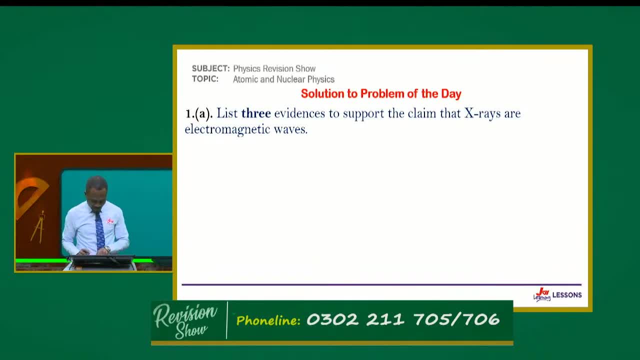 okay, why are you calling from, please? all right, so we want to answer Question number 1A. Yes, All right, please go ahead. So the evidence one: Okay, It travels x-rays. it travels through a vacuum. Good, 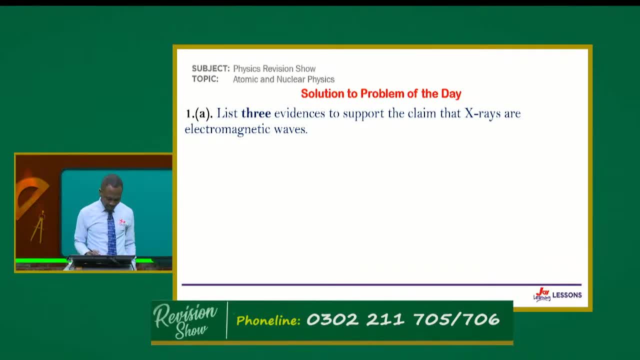 X-rays travel through vacuum. That's why they are claimed to be electromagnetic waves- Good, good. And the second one is: x-rays can be polarized- Good, They can be polarized, okay, Yes. And the third reason is they travel at the speed of light. 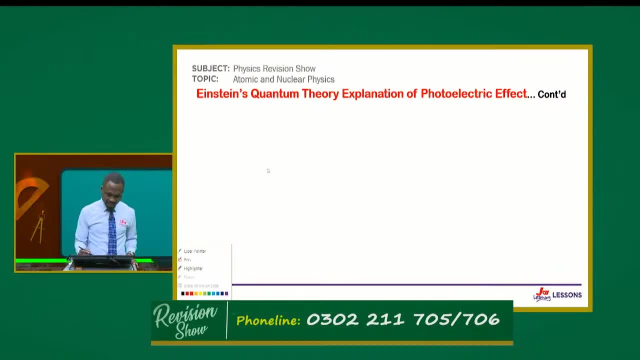 Good, They travel at the speed of light. That's also good, Fine, So thank you. Thank you so much for calling My regards to everyone in Techieman watching us tonight. Okay, thanks, Good, So today my students, my viewers, have been able to really do justice. 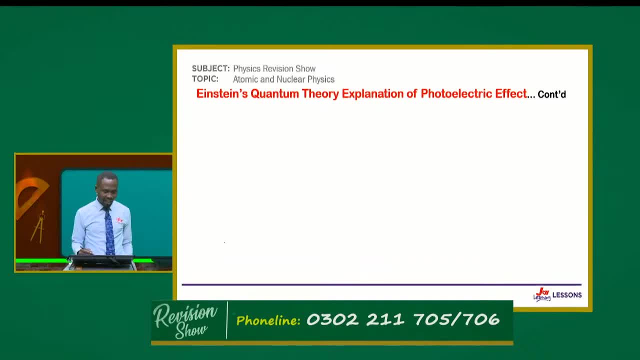 to the Problem of the Day questions. So you see what I've been telling you: that it's advisable to try your hands on question number 12.. Why? Because question number 12 is manageable. Once you prepare for it, you will be able to just get all that you're supposed to get. 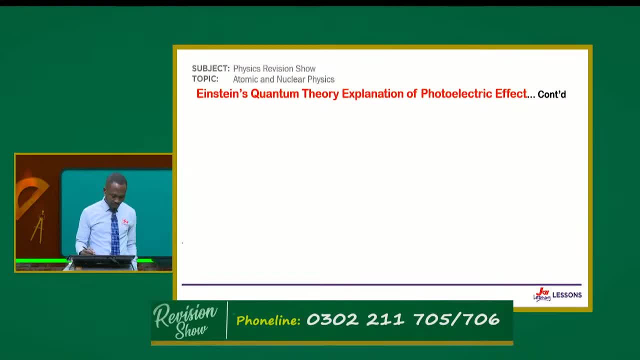 All right. So thank you for calling. We appreciate your call. Thank you so so, so much, All those watching us. Thank you for calling. I have a caller on the line. Hello, Hello, Hello, Hello, Good evening. 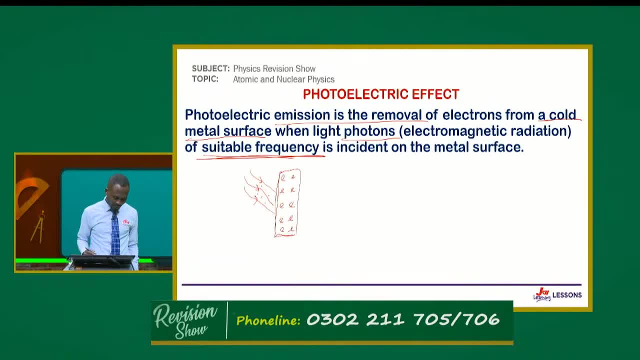 It looks like I've lost the caller. So we're looking at photologic effects, So we have a little bit of a picture. We have electrons on the surface of the metal and once the photons are incident on the surface of the metal, these electrons are able to gain energy and then they move away. 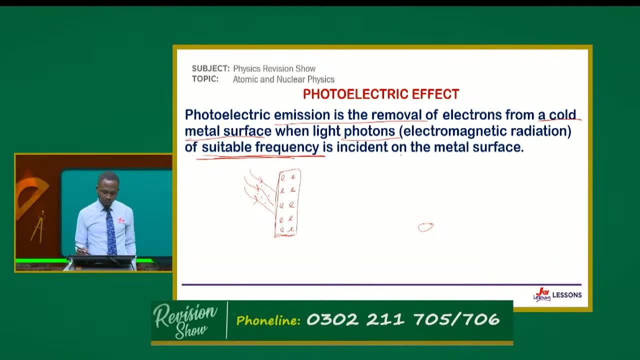 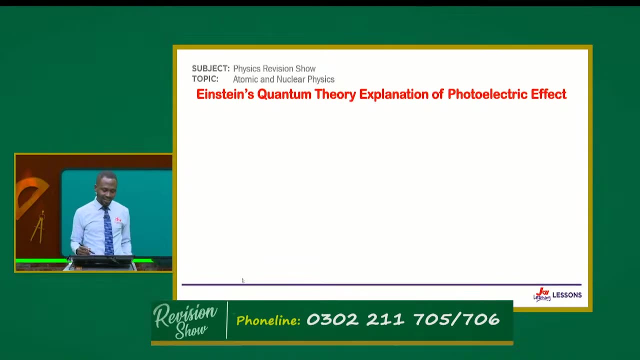 They move away, And this phenomenon is what we call photoelectric effect. Now, Einstein, He was a physicist And I'm going to explain it to you. So photoelectric effects gives a very good explanation to photoelectric effects. Einstein is saying that when you have the photons incident on the metal surface, it 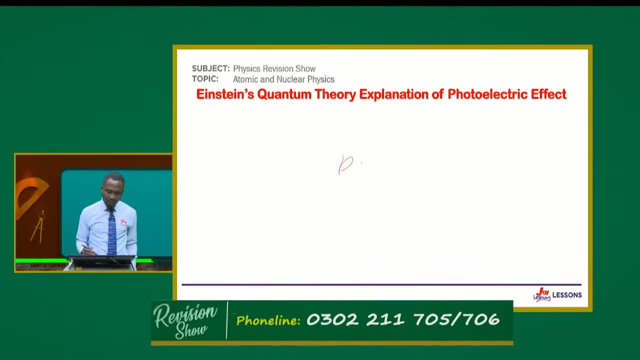 happens that these photons carry a particular quantum of energy, And he reveals an example. He was a philosopher, He was a scientist, He was a scientist, He was interested in physics, He was a scientist. that energy with E. okay, so E here is the energy contained in the radiations which 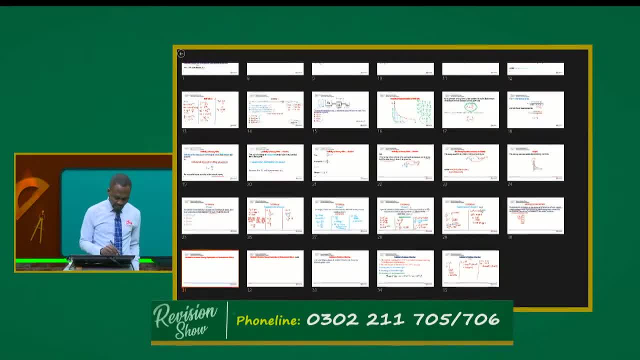 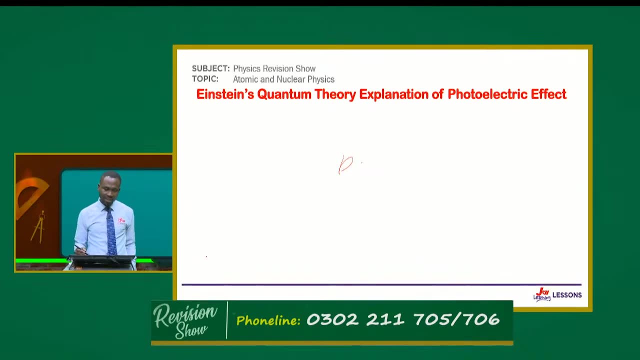 is the photons. and then he tells us that part of this energy is used to do work. product energy is used to do wake. what is our work? for that work is to break the bonds between the electrons and the surface of the metal. so part of the energy is used to break bonds between the electrons and the metal surface. 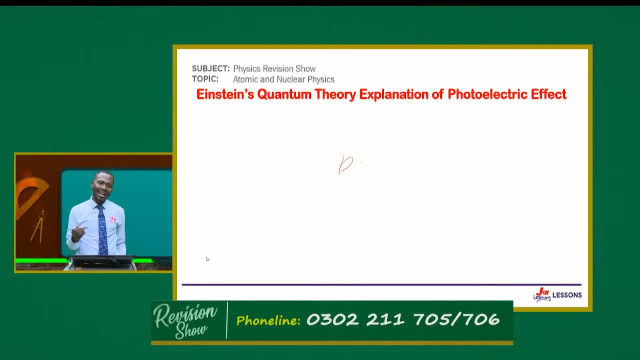 which you call the work function. then, as I says, that part of the energy that is left becomes the maximum kinetic energy with which the electrons move away from the cold metal surface, part of that energy left becomes maximum. I chance on the marking scheme from my egg where students were supposed to write or state: 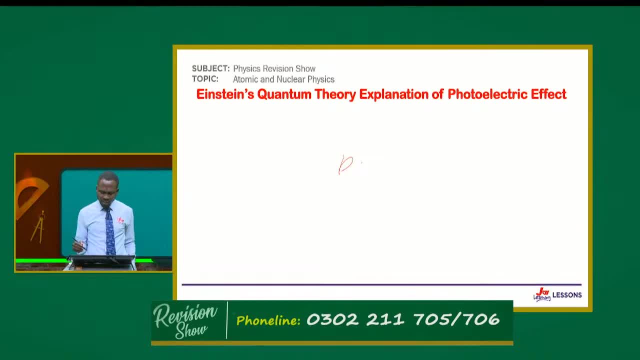 Einstein's equation for the defect, and then you magic. our connection is such that if students do not maximum to kinetic energy, the pros you'll be given. so when you are writing that equation e is equal to W plus key is kinetic energy, you have to bring subscript marks, because that is. 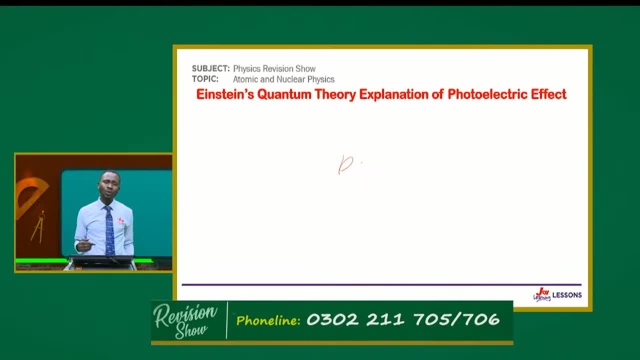 the maximum kinetic energy. so we can define the work function and we can also the threshold frequency. we are saying that the photons that are going to incident on the metal surface, they should come with a particular kind of frequency, a suitable frequency called the threshold frequency, and f- it's not f naught- is used to present threshold frequency, f naught. now, 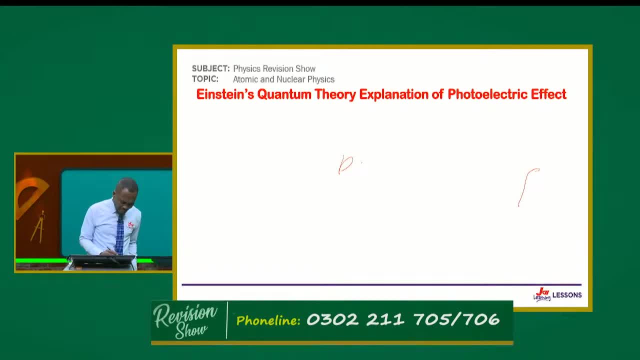 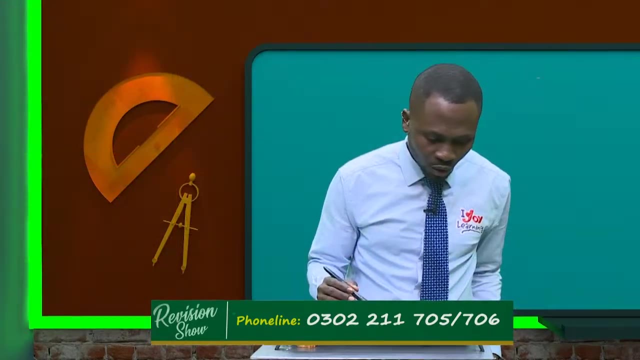 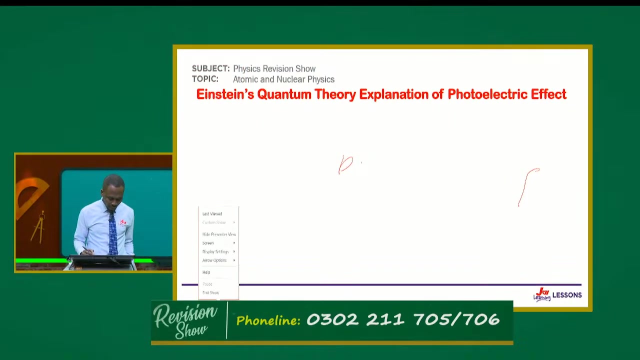 what we are saying is that when the photons are incident on the metal surface, if they don't come with the right or with a stable frequency, they will not cause electric effects. they will not cause electric effects, they must come with a suitable frequency, which you call it frequency, and when that happens, 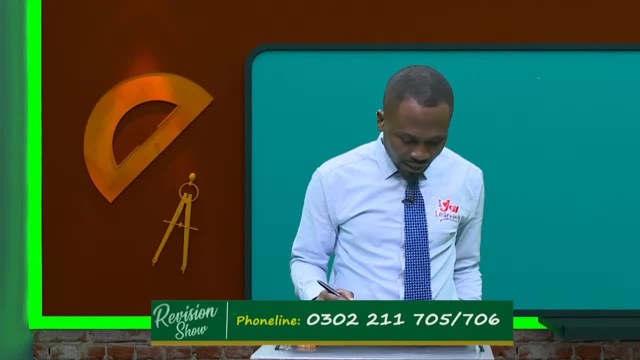 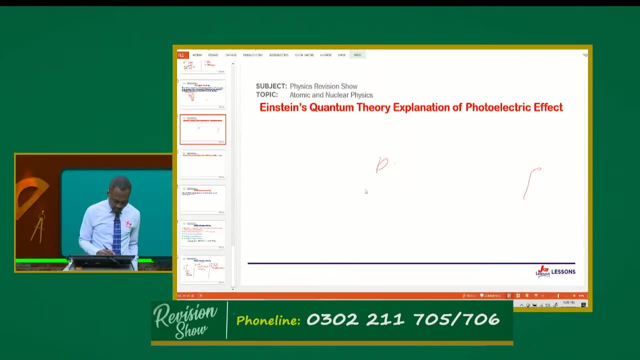 we are going to have electrons gaining all the energy of the incident photon and in that case they are going to come out of the metal surface. so i want to get e, being the energy is equal to the work function plus maximum kinetic energy with which the electrons move out of them, the data surface. now, if you make 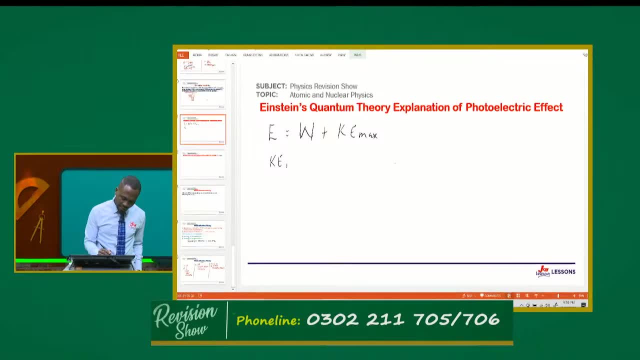 ke minus the subject ke max becomes e minus w. now e is equal to plant constant times frequency and w is equal to h f naught, where f naught is called threshold frequency, threshold frequency, so we can get this equation to be: ke max is equal to h f minus h f naught, and this equation is called einstein's equation. 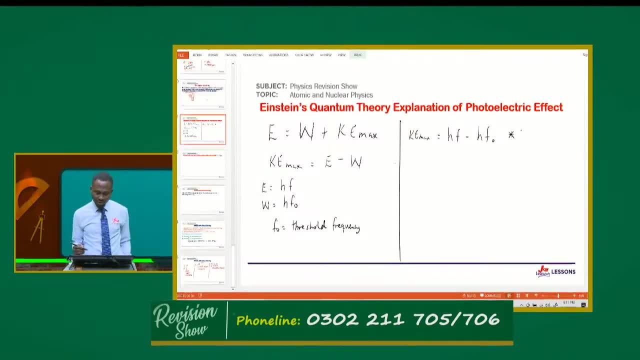 for photoelectric effect: einstein's equation for photoelectric effect. this equation can help us solve a number of questions. from this equation to you can try and draw a graph. now i want to compare this equation with the equation of a straight line. y is equal to m, x plus c. so if i'm comparing, 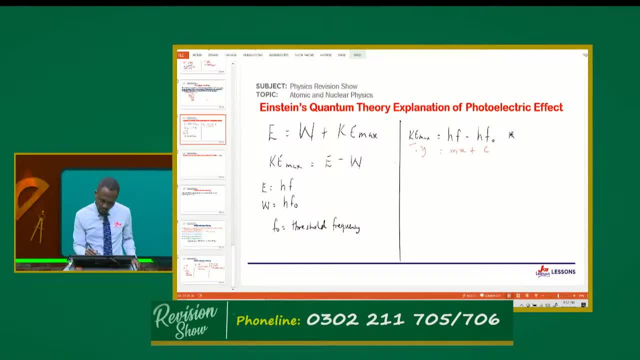 the y axis of the expression f. if i'm in the straight line, then ke max should be on the y axis. then i'm going to get frequency on the x axis, then the gradient i'll come to it plus constant, then i will have an intercept c and this whole expression hf notes, because i intercept, so should. 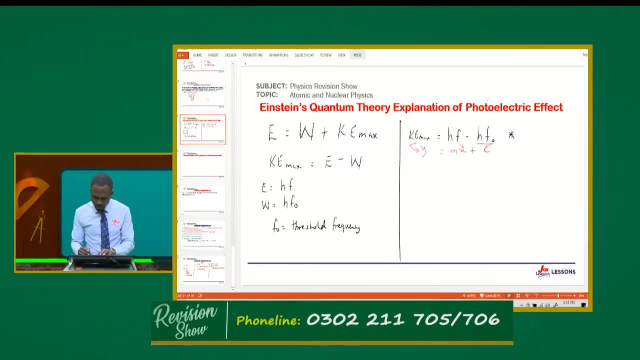 we try to get a graph like this. so I'm on the graph like this and I'm going to plot K max here on the vertical axis against frequency F. so this will be in joules, this will be in hertz. now I'm going to get a gradient M which is 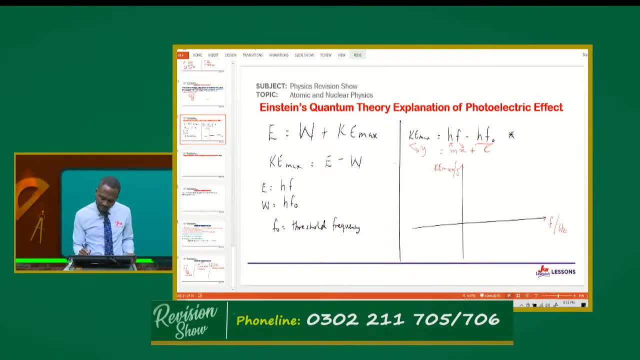 positive H, then I should get an intercept on the negative axis. so my graph is going to rise but it will not pass through the middle, or let me say the origin. it will not pass through the origin. it's going to get an intercept on the negative axis. 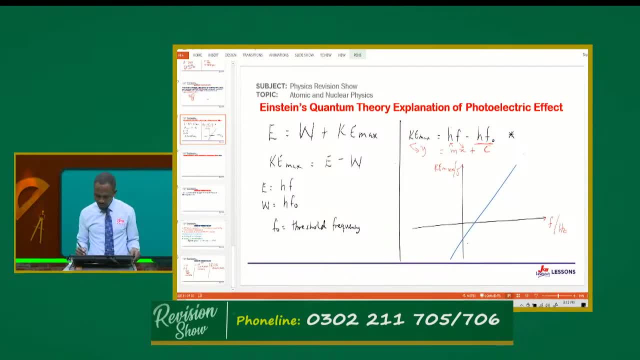 this way. so this place will be my intercept on the negative axis. so this is the same as minus H, F naught or minus W, and here I'm going to get F naught, which is the threshold frequency. then if you find the slope of this graph, 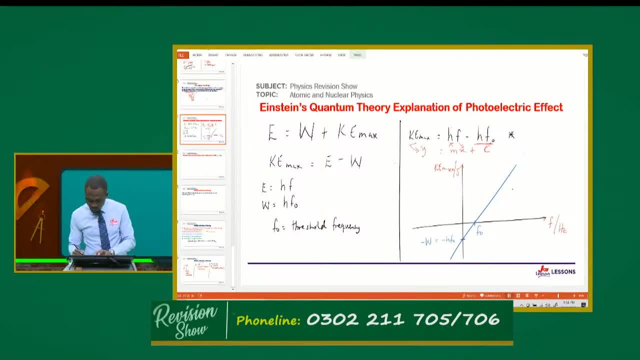 why can drop this graph for you label portions and ask you to identify those portions? so this becomes my slope, and my slope represents the plant constant H. my slope represents the plant constant H, h. all right, right from this expression to, we can see that ku max is directly proportional to hf, which is e. 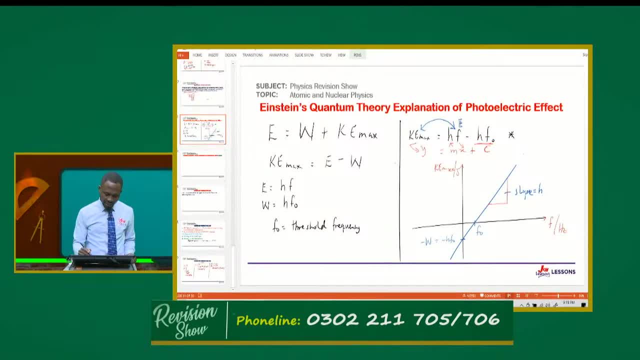 the radiations, the energy of the radiations. now we are recall fundamental characteristics or properties of effects which are similar to something like laws of effects. one of them is that the kinetic energy of the photoelectrons, what the electrons? electrons are simply the electrons that are emitted out of. 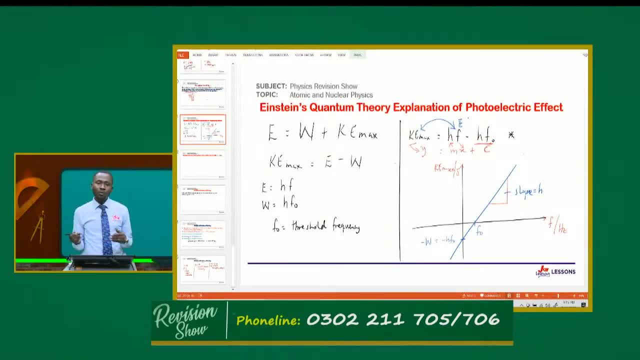 the cold metal surface when photons of stable frequency are incident on the metal surface. so if you have photons with the right frequency hitting the metal surface, the electrons that go out that are emitted as a result, they are called photoelectrons. now the energy of these photoelectrons- kinetic energy- will see the move very proportional to frequency of the incident. 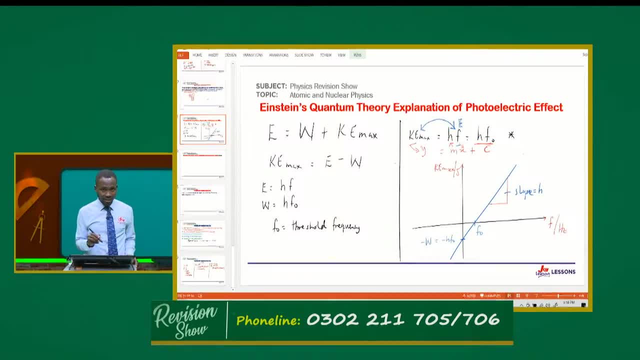 radiation very important. it is not dependent on the intensity of the light that is incident on the metal surface. rather, is dependent on the frequency of the incident photon. now, for every metal to there is a particular frequency of the incident photon below which there will not be emission of. 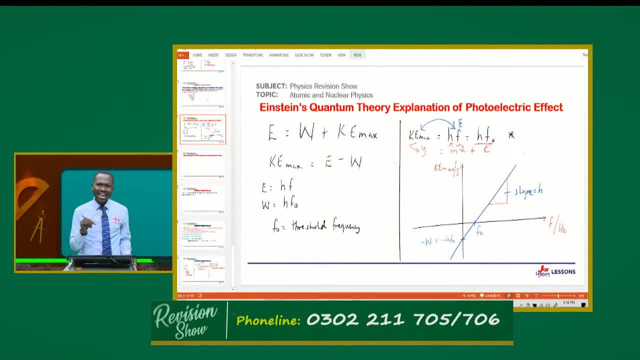 the photoelectrons. so as i say that every metal will have a particular frequency at which the photons should incident on it to cause the electrons to be emitted, to cause the electrons to be emitted. so as you prepare for the exams you should, you should be able to get this in mind. we have a 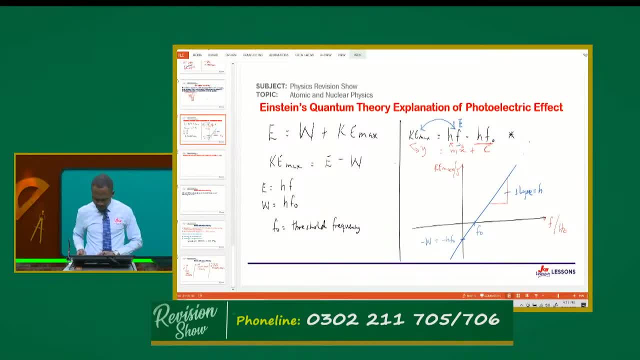 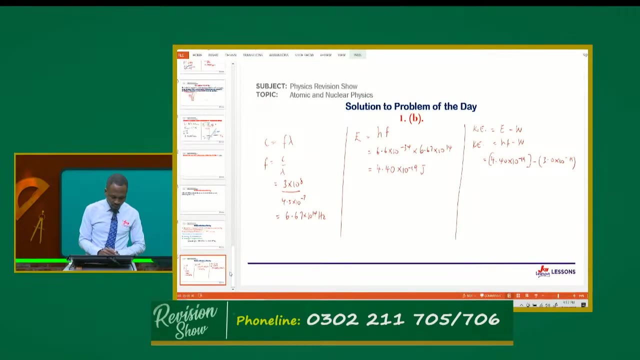 caller like: hello, good evening, your name and we're calling from, please, hello, my name is okay, please. why are you calling from, please? okay, at this description we won't be able to pick any more calls. we won't be able to pick any more calls. but, as i was saying, as you are preparing for the exams, you need to understand some of 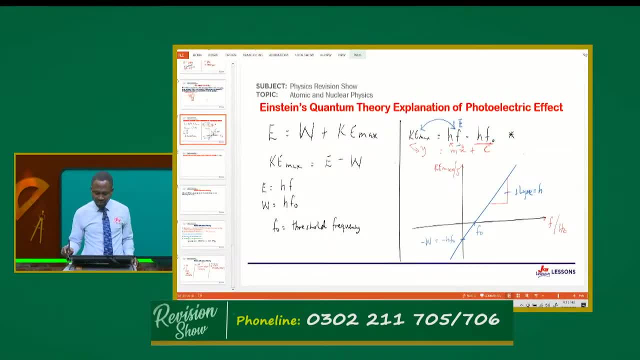 these things, why i could not really ask you to state the laws of photo effect, no, but rather you will be given scenarios like maybe in a different way that you will be able to get the results, because right now you are giving scenarios like maybe in a different way, the different process, you 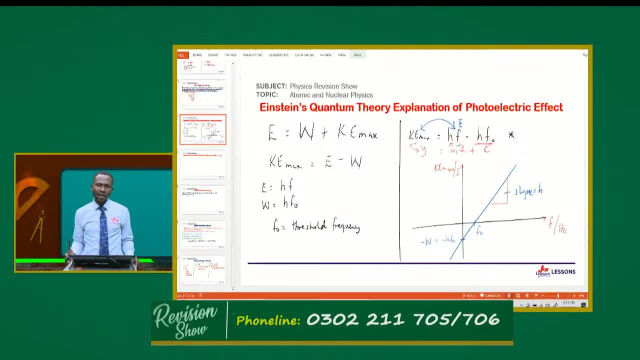 will be given scenarios like maybe in a different way, the different process will be different ways. Like maybe in a photocell, what will affect or what will influence the rate at which photoelectrons are emitted? Or in a photocell, what will influence the energy with which the electrons move? 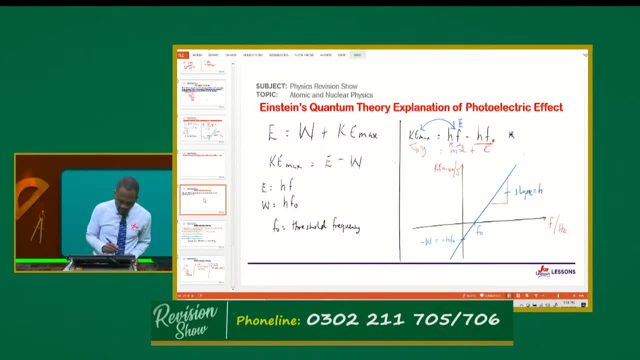 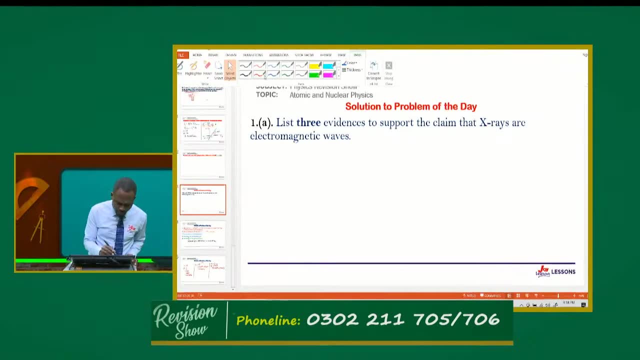 Okay, so you need to consider all these things Now. we had a question about X-rays and we're asked to tell or give evidence that supports that X-rays are electromagnetic waves. So what are electromagnetic waves? Waves that can travel through both vacuum, so they can go through vacuum. 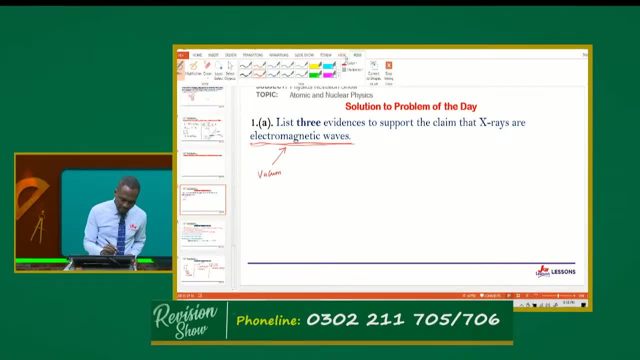 And they can also go through a material medium, So waves that can go through both vacuum and a material medium. So if there is a vacuum they go through, if there is a material medium they go through. we call them electromagnetic waves. 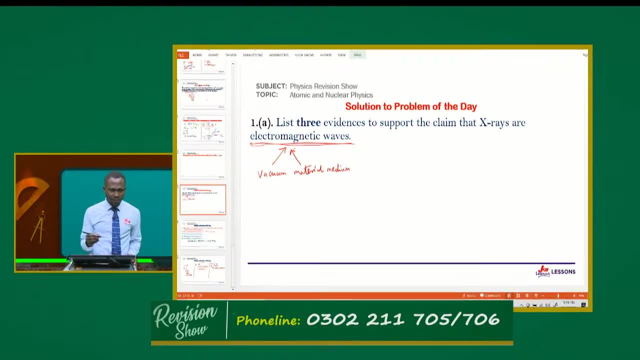 Then these waves have got some properties And, like the caller said, they travel in straight lines. They travel in straight lines. That's one, Two. what else can they do? They travel with a speed of light in vacuum. They travel with speed of light in vacuum. 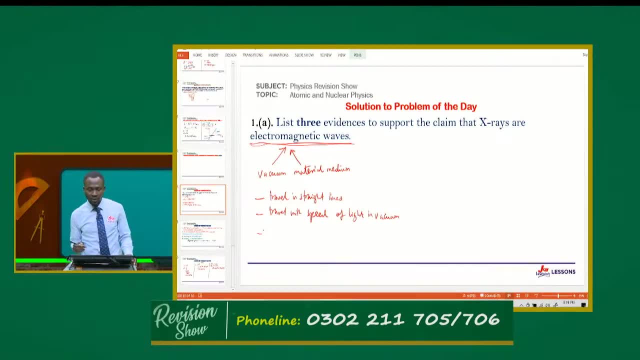 They move with a speed of light in vacuum, Which is Three point zero times the power, eight meters per second. Now they can be polarized or they can be. they can be polarized. So these are the answers that the caller gave. 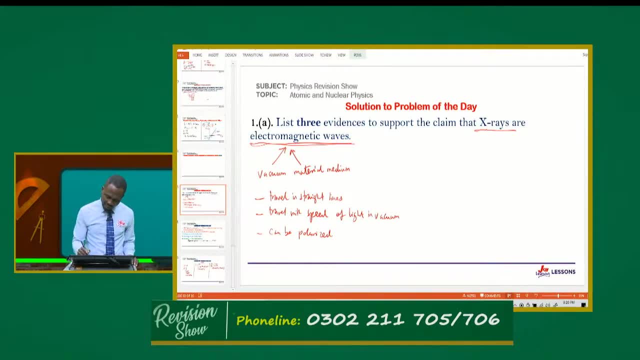 Now I want to focus on what we call X-rays. Then we can draw the curtains for tonight's recent show. What are X-rays? Sometimes ago, X-rays were used in the medical field for something which is no more So, because now we have what we call the ultrasound scan, but still we can use X-rays to detect bone fractures. 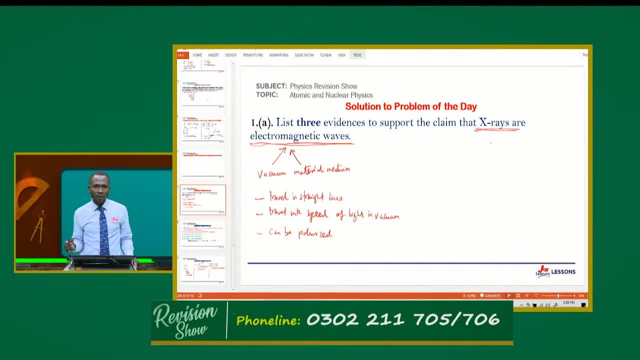 You can use X-rays. normally you go for X-rays to check what is going on with the bone, what is going on. if there is a fracture, you want to locate where it is. X-rays can do that for you. X-rays can even help us locate, maybe, a swallowed object. 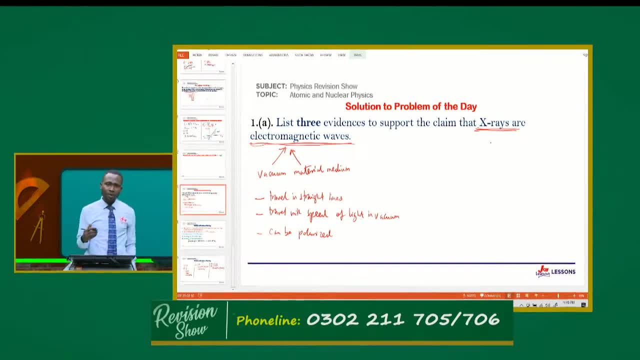 So what are X-rays? The production of X-rays is an application of what we call thermionic emission, So thermionic. So I want to take the opportunity to talk about this because we're talking about photoelectric effects. Now, in photoelectric effects you have photons incident on the metal surface. 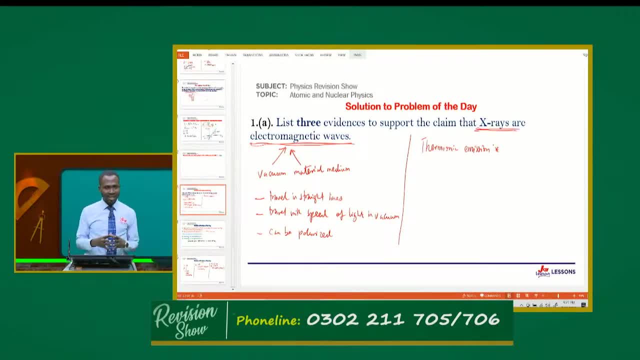 Electrons get energy, Then they move out In thermionic emission. you have a metal and the metal is heated to a sufficiently high temperature. As a result, electrons are emitted from the hot metal surface. So the emission of electrons from a hot metal surface, when the metal is heated to a sufficiently high temperature, is called thermionic. 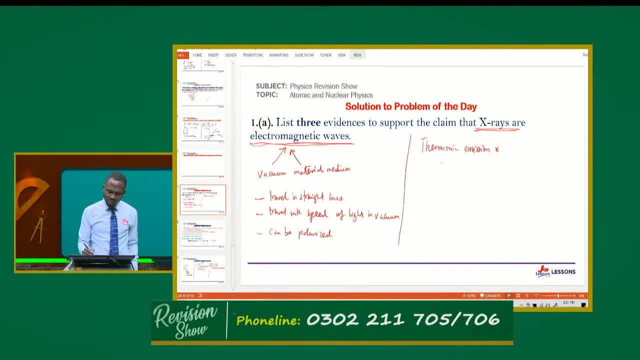 And those electrons that are emitted are called thermal electrons. So they are electrons emitted from a hot metal surface, when the metal is heated to a sufficiently high temperature. Now, to get X-rays, you must get what we call cathode rays. 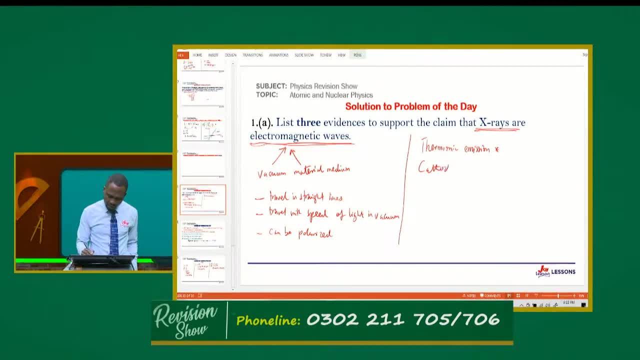 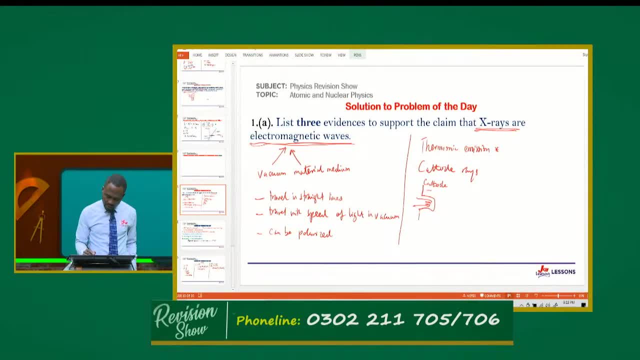 A metal negatively charged, Then I have an anode. So let me see this one. This is my anode. positively charged, charged. This is my anode as a target metal. Now, when the cathode is heated, when the 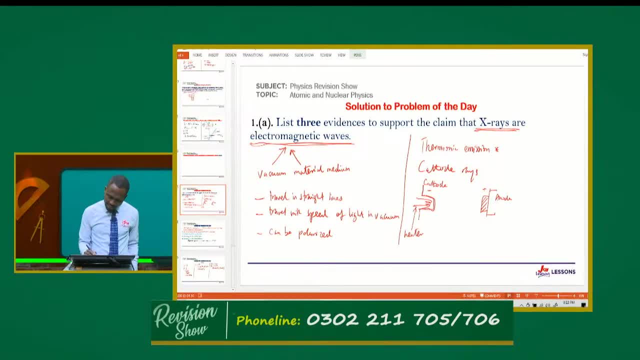 heater heats the cathode, the metal gets heated to a sufficiently high temperature. electrons then go away from the cathode, So a stream of electrons which you call a cathode rays. so stream of electrons called cathode rays. they move from the cathode and because they have a negative charge, 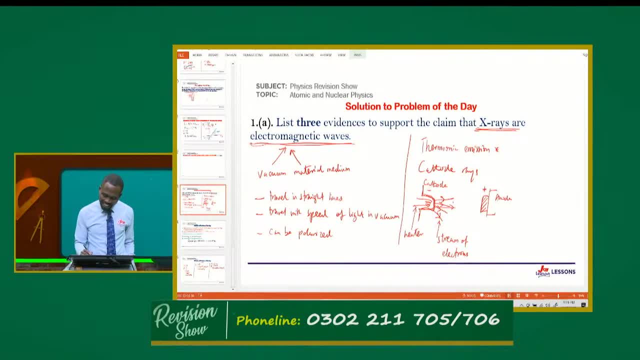 have a positive anode in front of them, they accelerate towards the anode so they come to hit the target metal. but they cannot penetrate through the target metal. they cannot go through the target meter. so what happens? they hit it and as they are moving, they contain, they have kinetic 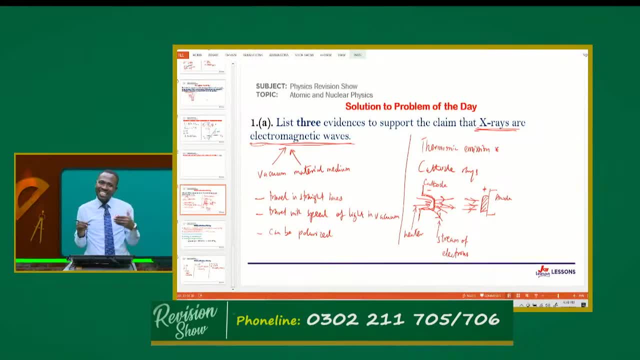 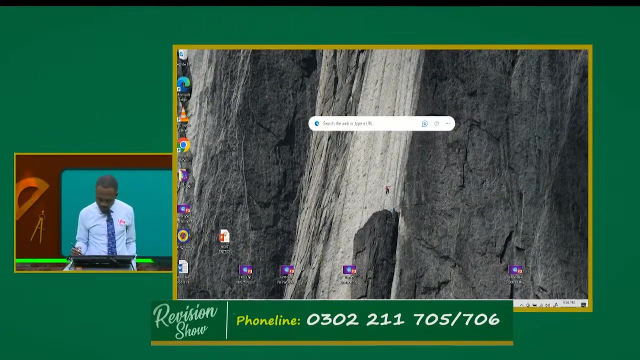 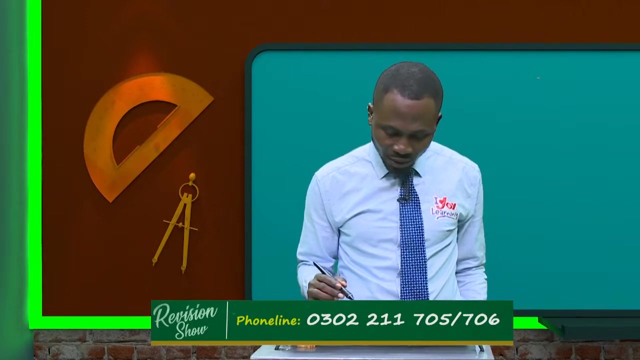 energy. so as they come to a sudden stop, they are going to lose some energy. in losing energy, they give off radiations, radiations. these radiations that are giving off i want to call x rays. i will call x rays. so x-rays are electromagnetic radiations. simple as that. x-rays are electromagnetic radiations. 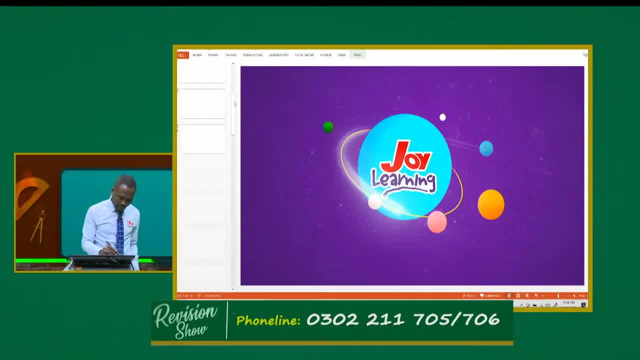 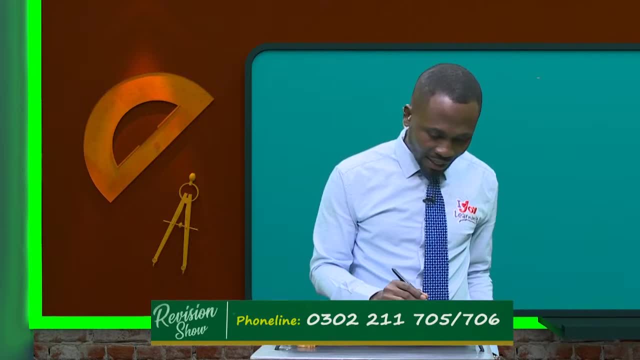 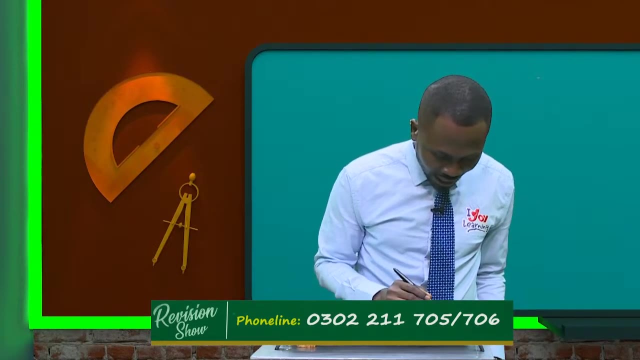 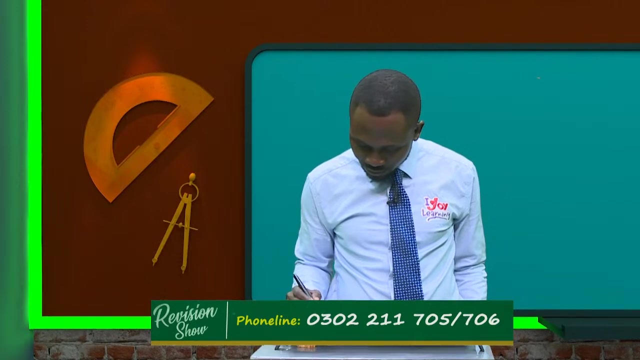 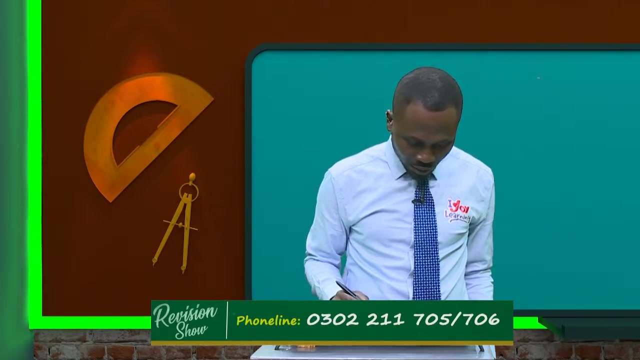 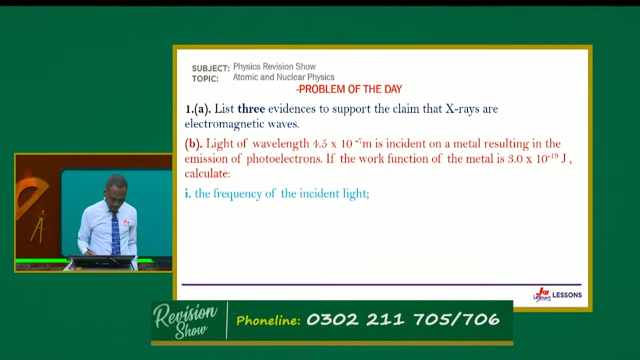 that are emitted from a core, from a metal surface, when that metal is struck by fast-moving electrons. fast-moving electrons, they are called x-rays, x-rays, so x-rays are electromagnetic radiations that are emitted from the metal. when the metal is struck by the fast electrons, the electrons will give off, they will give off radiations and then 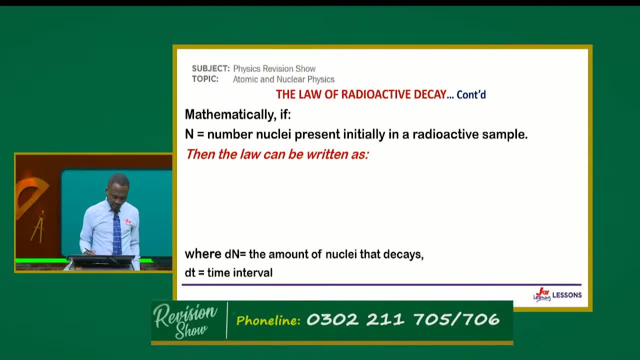 we have what we call x-rays. so usually we just say the x-rays are electromagnetic radiations obtained or produced when fast-moving electrons are struck, are stopped by a target metal. i think that's all time you don't permit us to have tonight. tonight we're able to look at. 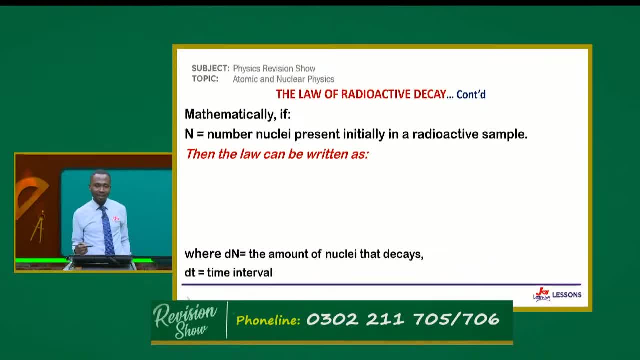 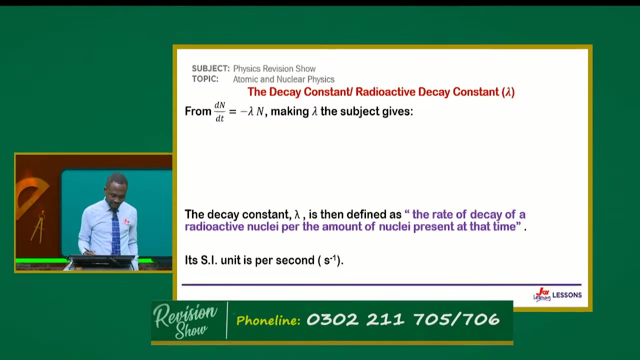 the law of radioactive decay, look at the decay constant, at the decay equation. so as we prepare for the exams, read around these lines, do not forget the equations that you will need to recollect as you move on. and then try your hands on some of the equations that will let you. move on as you move on and then try your hands on somets and some of these equations that you will estar on, and so they will generate you a evaluation that you can do, an districts observation that will create to a particular situation that will suggest they will be able to depend that you are not require that and them. they may remember you are special for you are going to consider it this way. if you can conflict the, also, tools will be able to anticipate and guide how a person is of the ongoing tasks. May, for example, anson how much time and effort the motionije three times a day only you have so far. 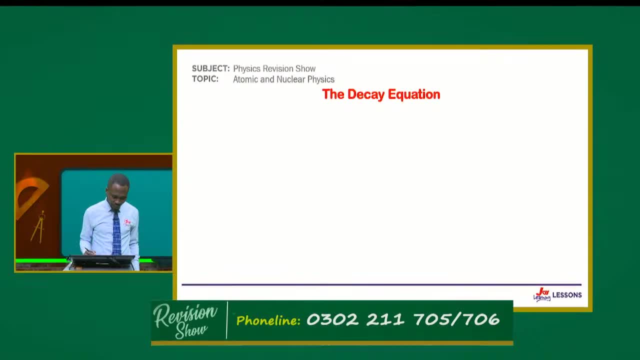 hands on some of the past questions and the decay equation, decay constants, half life, and then you should be able to tell that you are really poised for the exams and then we will get you covered here on the joyland interlucent channel with what you should expect and what should keep handy. okay, so as we go through the 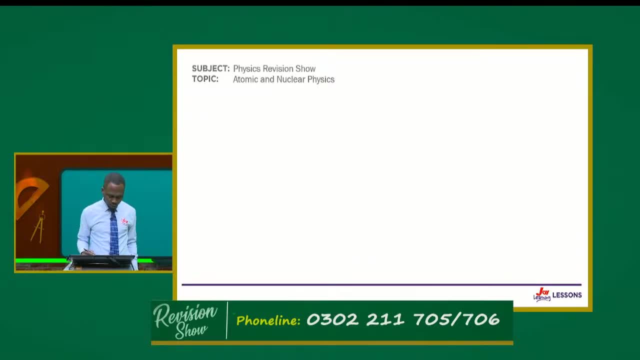 week. make time with us here by YouTube or Facebook, then we would be able to help you get up to date with what are supposed to know. in our next show we try and look at other areas too, but you can master as far as the exams is concerned, as far as the exams is concerned. so you take good to Joel and 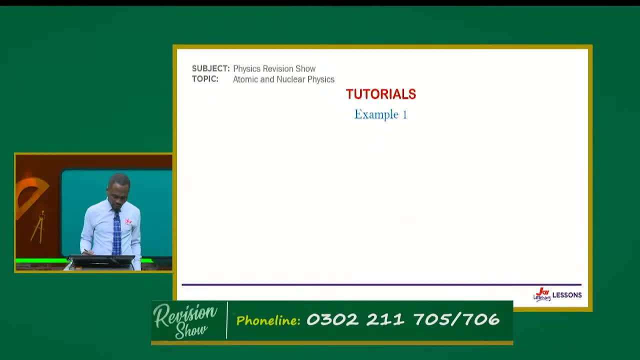 intuition and we say: you keep learning alright. so with the lesson coming to an end, you need to know some properties to of x-rays. x-rays have a very high frequency. that is to see the rate at which they can move through matter and out of matter per second is very fast. so x-rays have very high frequency, very 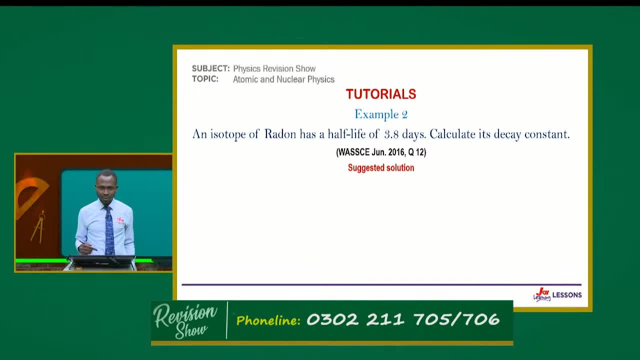 high frequency but I have a short wavelength. okay, so when you draw the electro magnetic spectrum you are going to have x-rays as part of a certain frequency. you are going to have many frequencies. you are going to have of the spectrum right, maybe in increasing order of frequency, if you do. 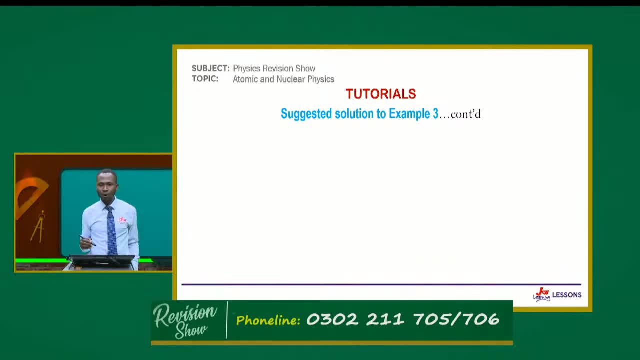 that you see, x-rays come just before gamma rays. x-rays come just before gamma rays, telling you that x-rays have a very high frequency, but you have C equals F lambda, F equals C on lambda, so frequency and wavelength are inversely proportional. in that case, if they have a very high frequency, then they are gonna have a.